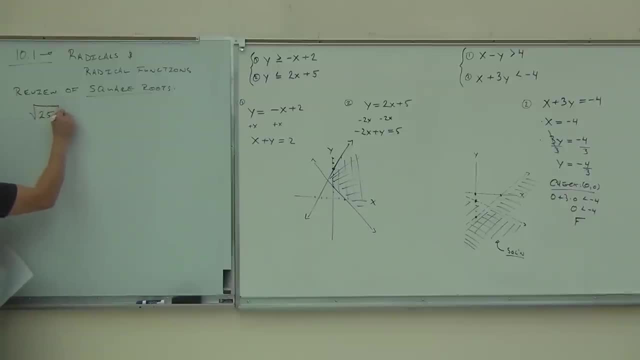 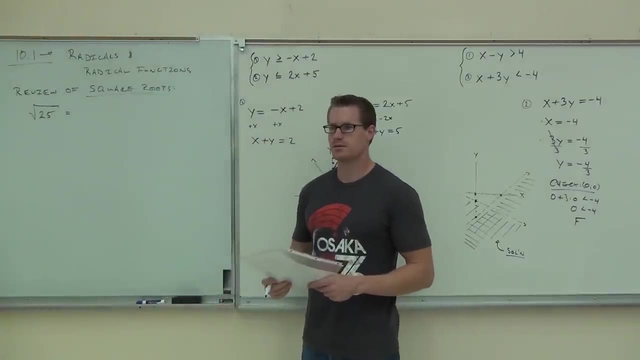 What does a square root do? Say that again: Okay, a base number, sure, Basically, what this is doing is undoing the act of squaring a number. So what you're saying is that some number squared would be 25,. 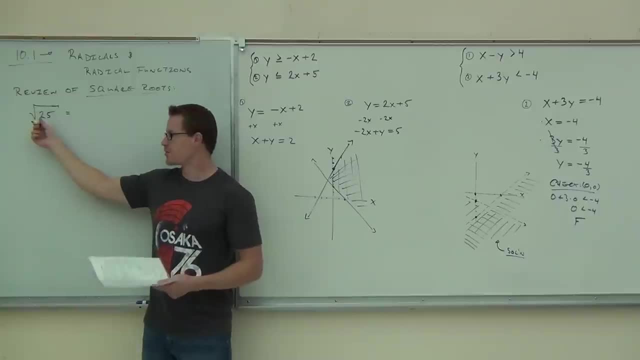 what's that number? Or undo this for the square and the number is Five. that's right. So we're saying five times itself would give you the 25 inside of our square root. That, by the way, if you want to know the name of that, 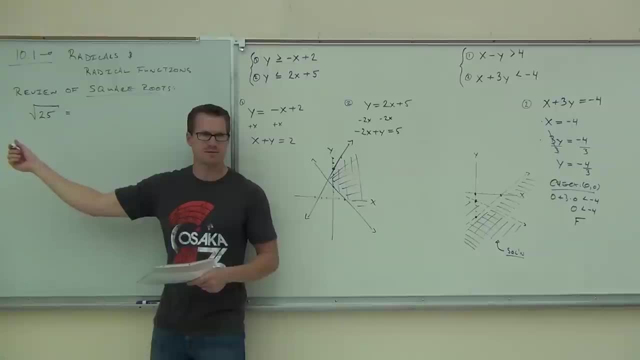 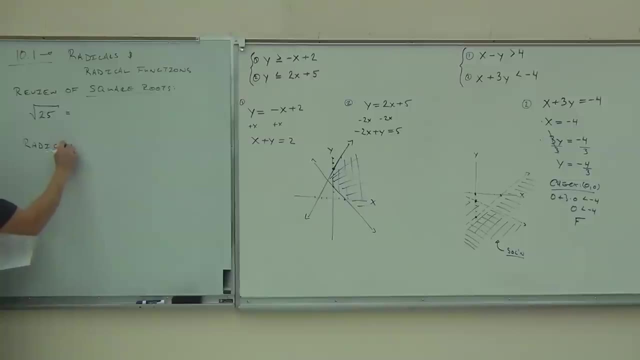 that's called the radicand. Can you say radicand Radicand? It's a Like that It's not radicant. all right, You can right: Radicand Radicand. Yeah, not radicant. 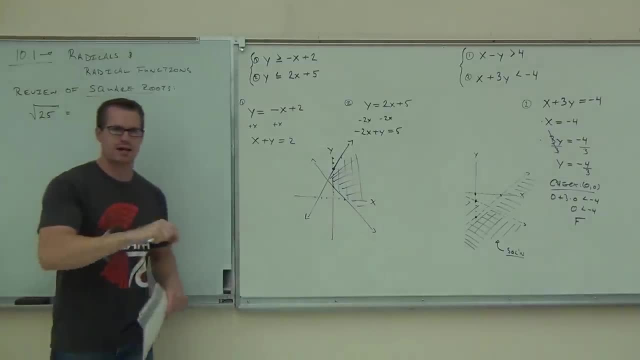 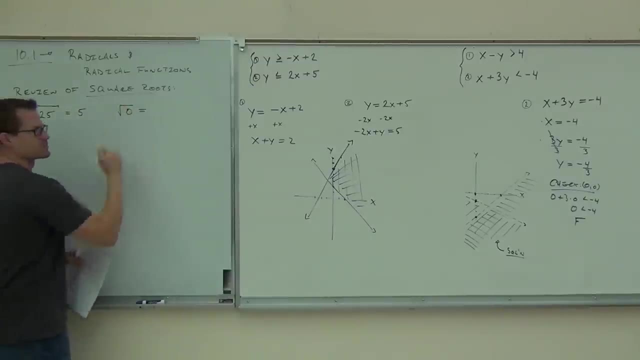 So we're finding what number times itself gives you the radicand In this case? yeah, it's for sure, five. How about the square root of zero? Is the square root of zero possible? Yeah, zero, Sure, why not? 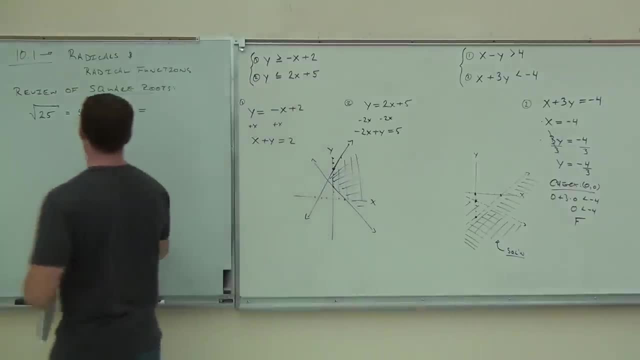 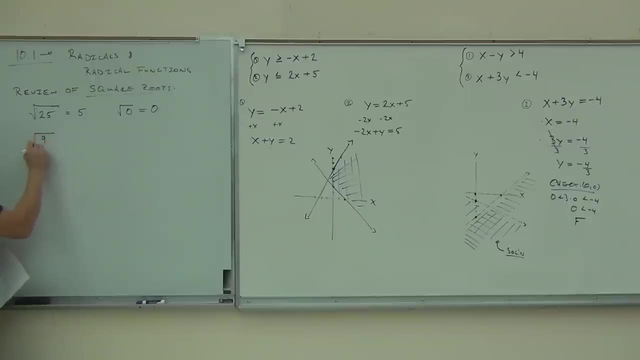 Is zero times zero zero. Yeah, that works So, yeah, that's possible. So when you get square root of zero, for sure you can have that. That's fine. How about the square root of fractions? Were we okay doing the square root of? 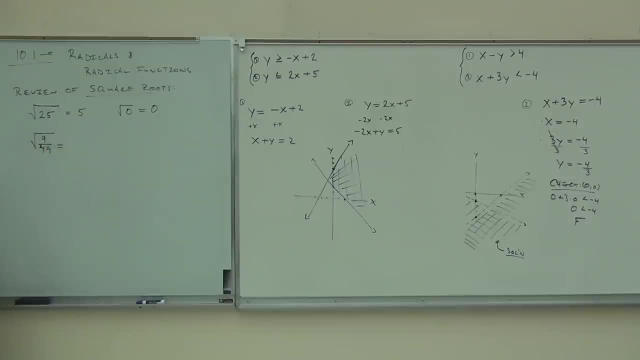 Fractions. Square root of nine over forty-nine would be Three over seven. Good, We take the square root of the top one, take the square root of the bottom one, the numerator and denominator. We have three over seven for sure. 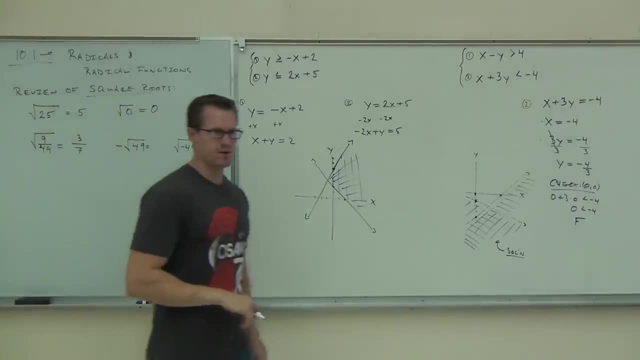 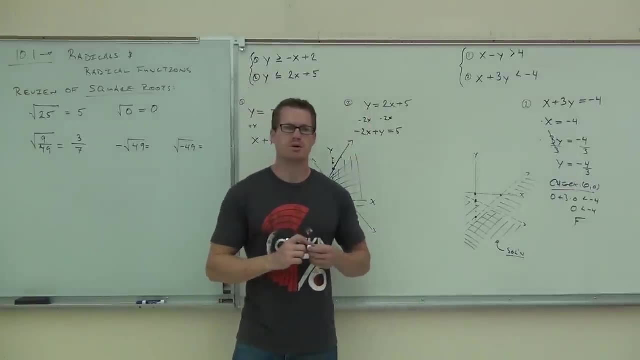 Negative square root of forty-nine and the square root of negative forty-nine. are they the same or are they different? No, only once possible. Only one is possible in what we know as the real number system. The other one will be possible when we deal. 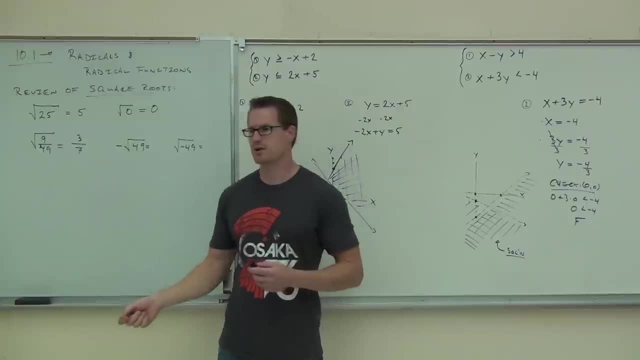 with the complex number system That's going to be in chapter well. end of chapter ten, 10.7.. So that's in this chapter. We are going to know how to deal with this one by the end of this chapter. 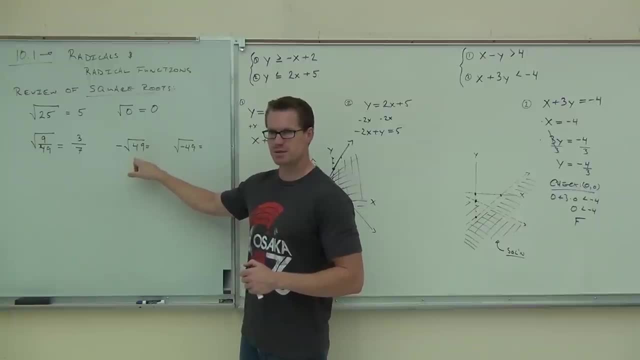 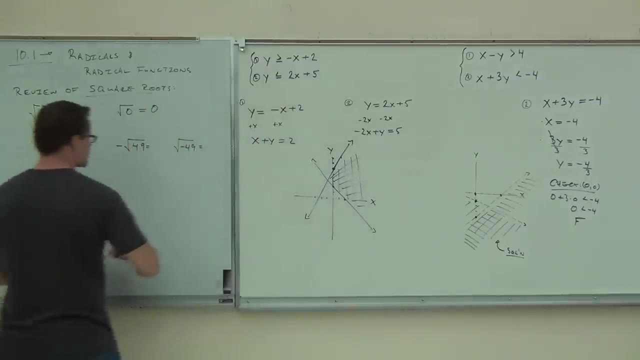 Right now we can only deal with this one. What's the difference between these Negative seven? the other one is not possible. Why is one negative seven? Because one negative seven is outside. Okay, very good. So in this case, when the negative is outside, 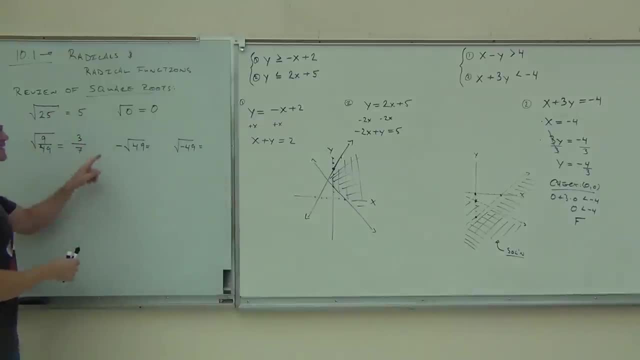 of our square root. it's not being applied inside there. This is saying: take the square root of negative seven, take the square root of negative seven and make the opposite of the square root of 49. It's basically what it is. 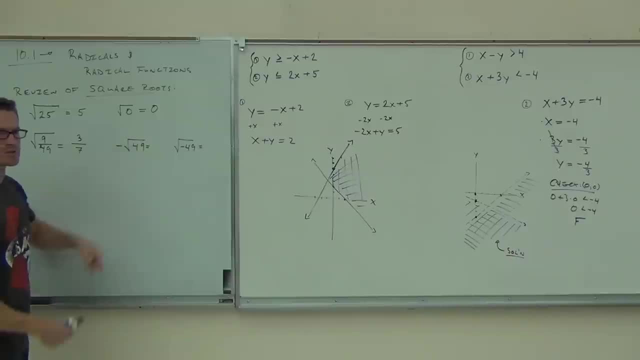 So you go: what's the square root of 49? And then make that the opposite, so negative seven The square root of negative 49,. right now there's no number times itself in the real number system. that's going to give you negative 49.. 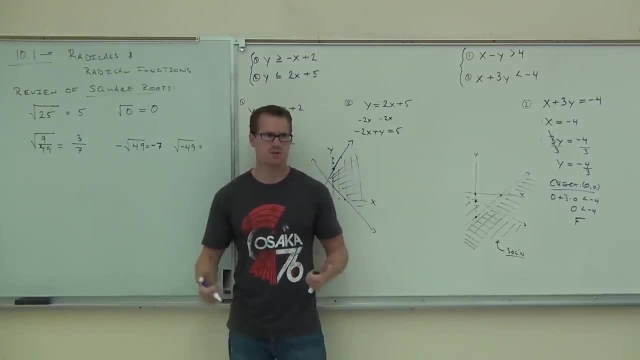 You do seven times seven, you get 49.. You do negative seven times negative seven, you get 49.. That's not going to happen for us. So here we have. well, I need you to write, don't just put NA. 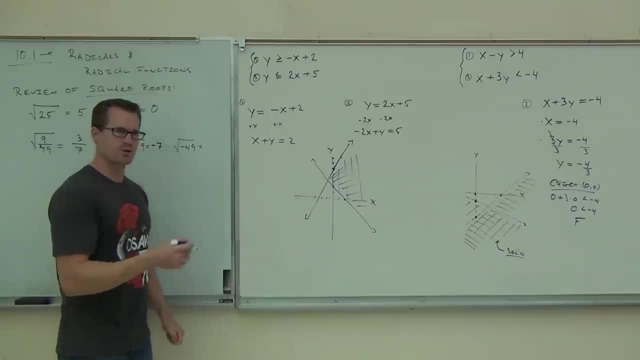 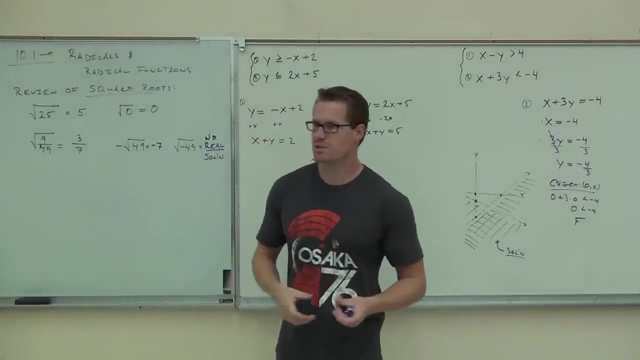 Don't just put no solution. I need you to be very specific, right? So we're going to put no real solution, No real solution, And what that says a real number is the numbers you've been dealing with since you were. 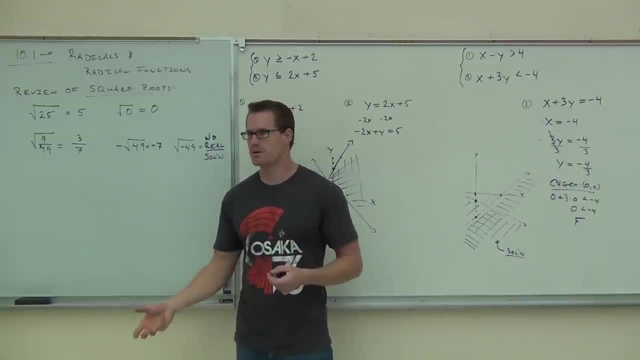 like in kindergarten. Every number you can probably think of right now in your head, Every integer, every rational, every non-ending and non-determinative or non-terminated, non-repeated decimal, everything you can think of is a real number. 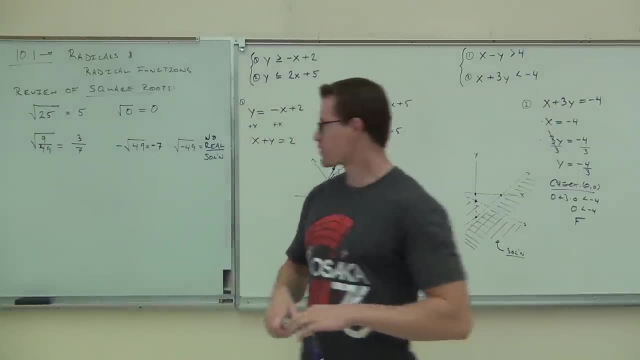 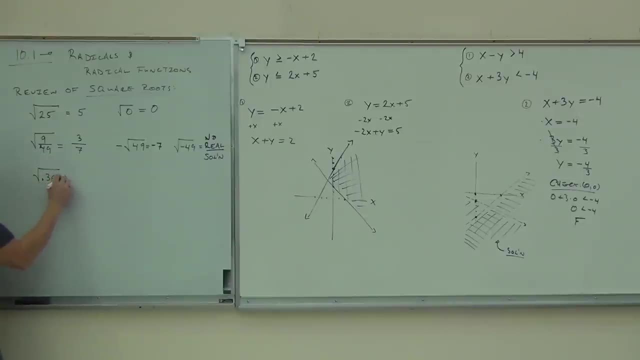 We're going to deal with another set of numbers at the end of our chapter, though. Okay, one more thing that we can do: square roots of decimals. How's the square root of 0.36?? Is it still possible to take the square root of a decimal? 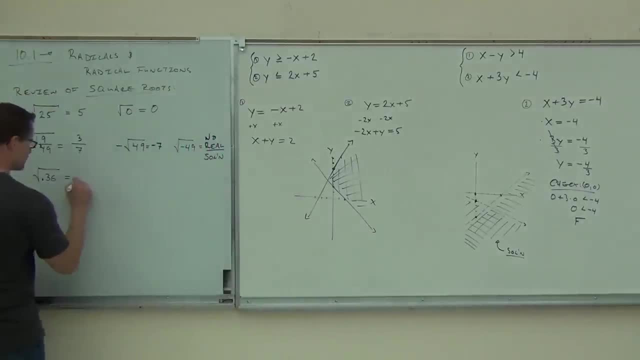 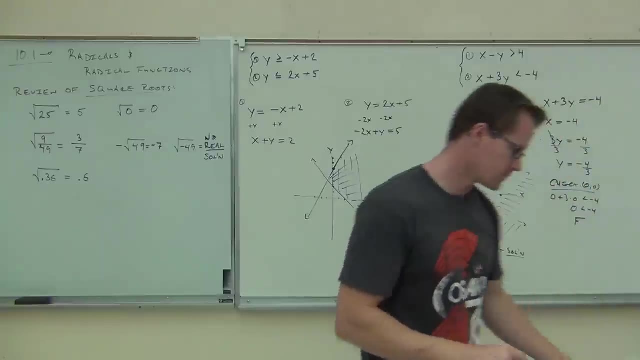 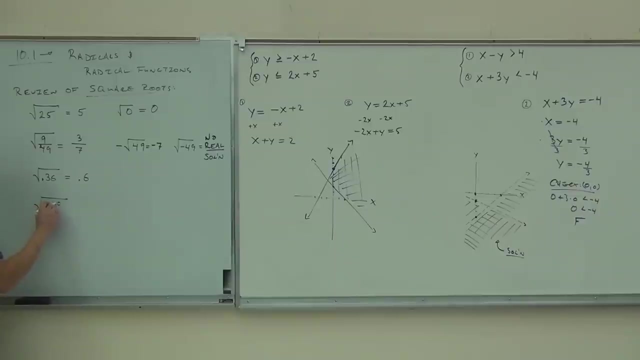 Yeah, for sure. yeah, yeah, It is actually 0.6, for sure. Yeah, 0.6 times 0.6 is 0.36.. That works Okay. Can you take the square root if it involves variables? 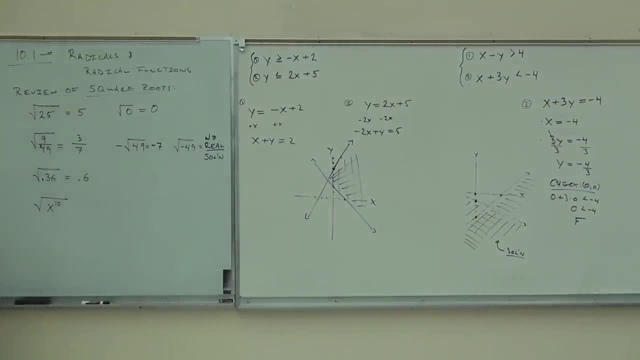 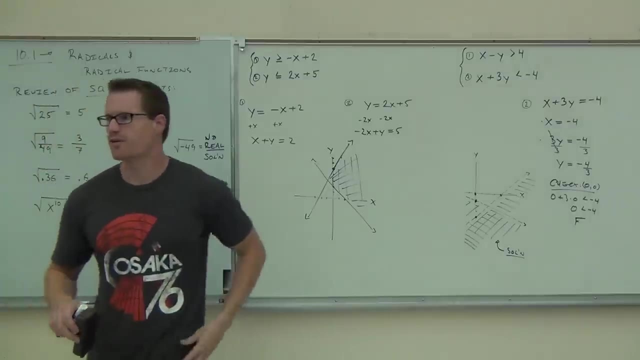 How I need you to understand. yeah, you're right, I need you to understand what we're actually doing here with the square root of 25.. So, if we're doing the square root of 25, what really is happening is that this is possible. 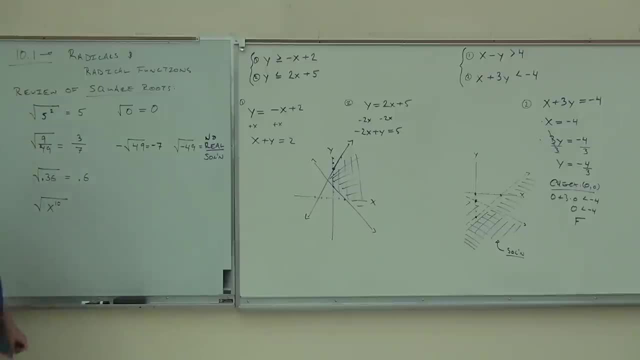 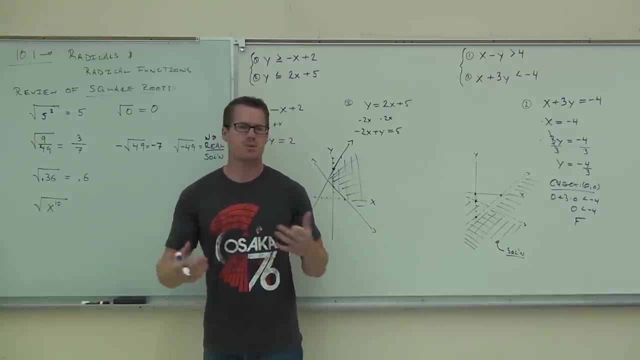 because this is 5.. That's 5 squared right And ultimately what's happening is our square root is undoing the squared part of this. You can think of it like that. They're inverse operations. So whenever you have a square and a square root, you say, oh, okay. 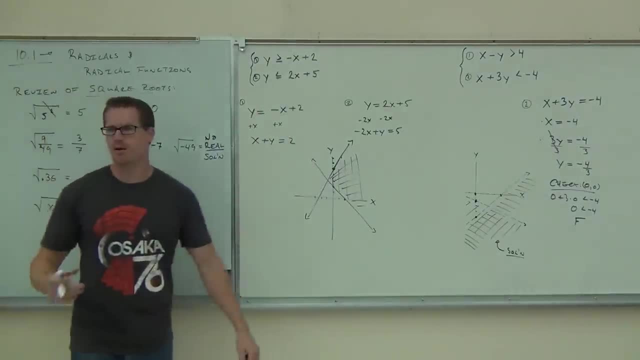 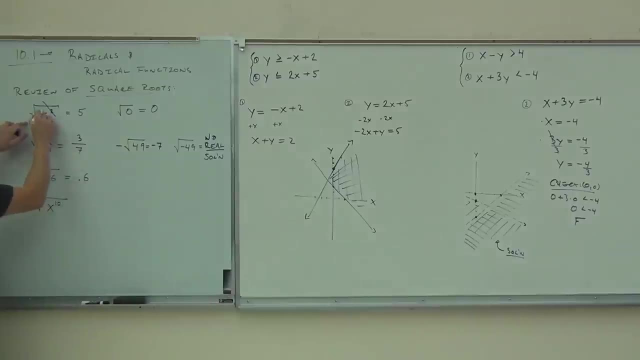 I know that, these two things, if you want to say cancel out or simplify away or whatever you want to call that, that's what's happening. The square root is undoing that square and we get whatever we're left with inside of our radicand. 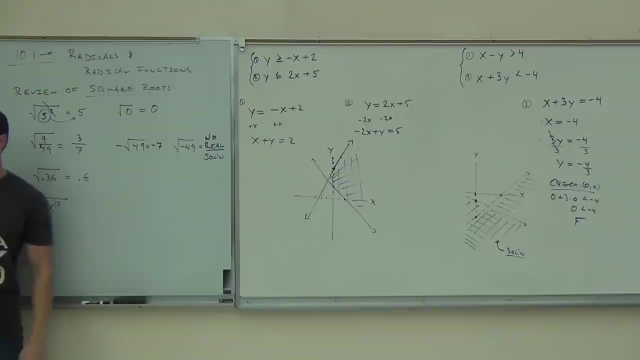 That's our answer there. That's why that works. Are you with me on that? You can do that with everyone else. I'm going to give you one of these examples. This is 3 squared, They're 4.. The square root's going to undo that square. 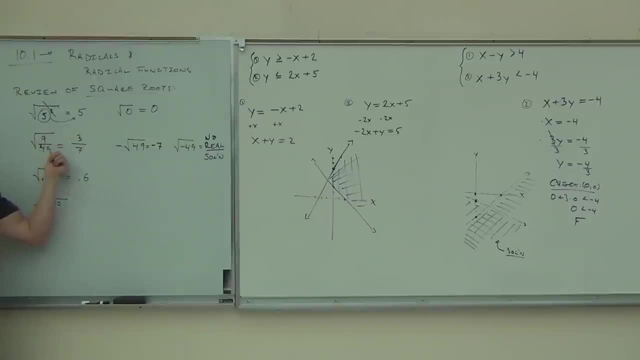 We're going to get 3.. This is 7 squared. The square root's going to undo that square. We're going to get 7.. I'm not sure if you're okay with that. All right, Can we write this in a similar way that we were able to write that? 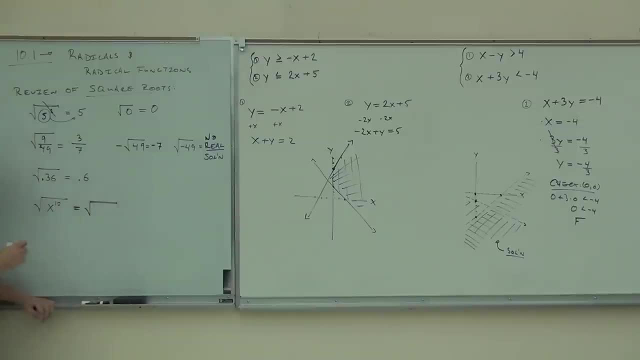 And the answer is yeah. Yeah, if we write this as a square root of, instead of x to the 10th, I need you to be able to use those rules for exponents X to the 10th. you could write this as x to the 5.. 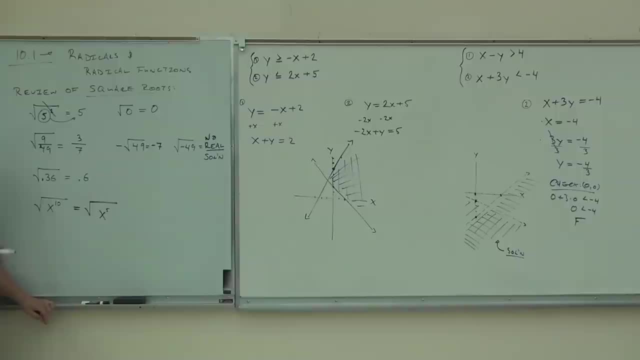 Well, wait a minute. We want 5 times 2.. How do we write exponents as multiplied? Do you remember when an exponent is raised to an exponent? What do you do with that? Like x to the 2nd to the 3rd. 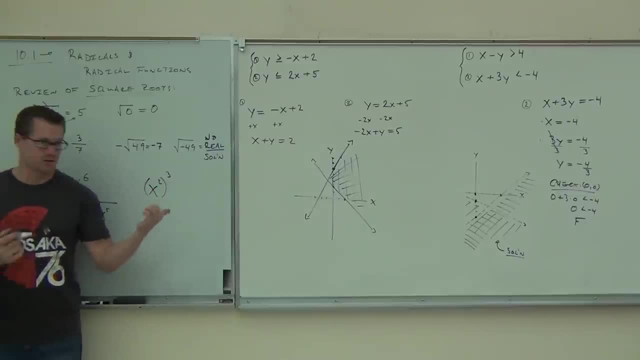 Do you add those or do you multiply those? You definitely multiply those, These ones. you would add, right, Those. you would add: These ones you multiply. What I'm going to do is try to write this in some way that I have a square up here. 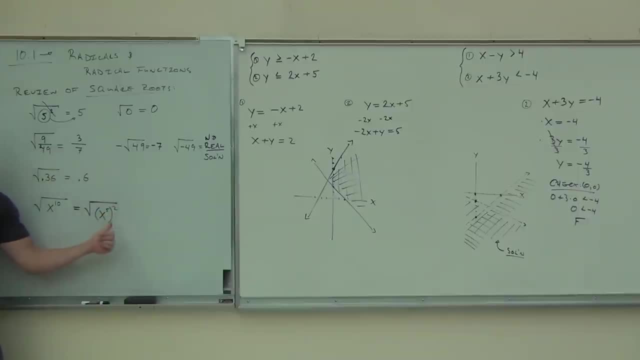 Is this square? Is this square? Is this still? x to the 10th? Sure, But now watch. I have a square root and I have a square. What happens to a square root and a square? Can't switch them out. 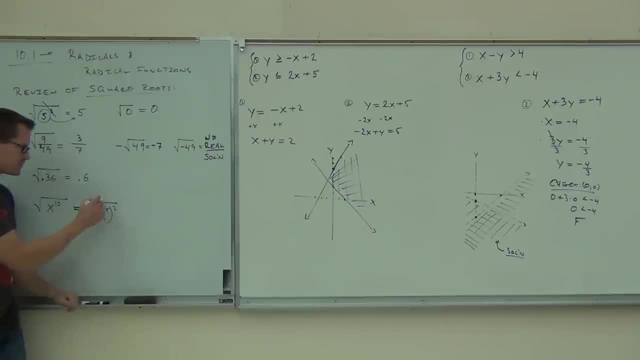 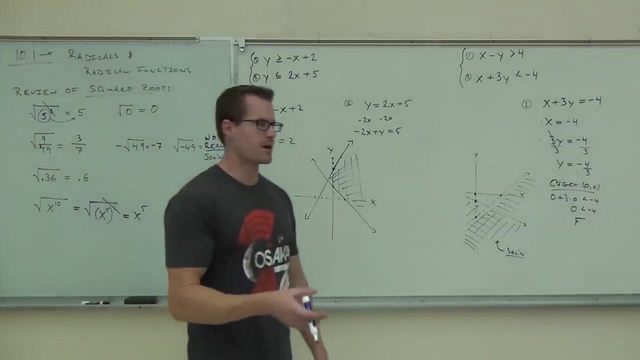 So they're going to eliminate each other and they're inverses. So, on the right hand side, what do I get out of that? So, by writing this as something squared, we can eliminate that. I'm going to show you. I'm going to show you one other way to do this. 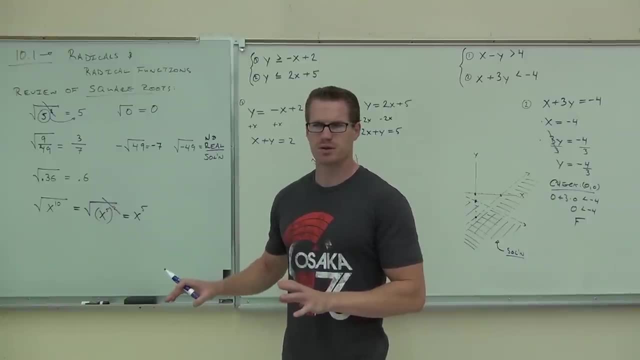 You're going to think right now that why are we going to do this way? This seems a little bit longer, But trust me on this. Get used to this way as well, because we will be using it later on. I'll show you this in a second. 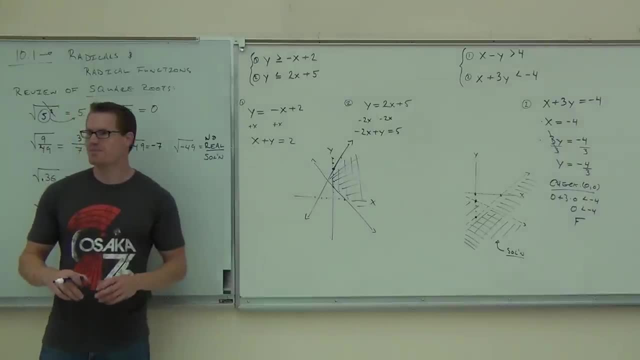 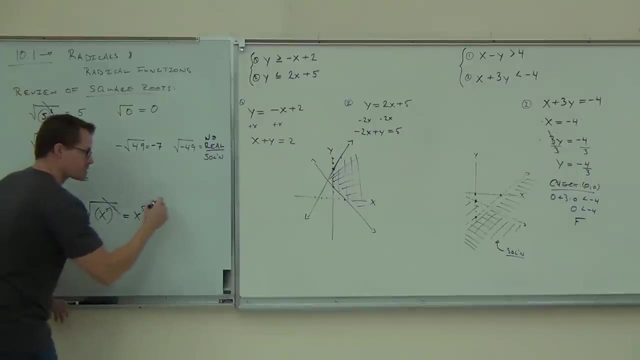 Well, actually I'll show you this in like a week and a half, But it will be good to practice it. There's another way that we can do this. Do you remember that I also told you we can when we multiply things like this: 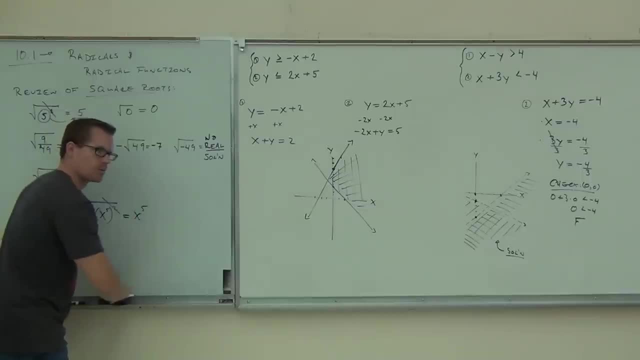 we add those exponents. Yeah, Okay, So we're going to do this. We'll watch it here on the board. We can do this two ways. We can do it this way: Great. Or you could write this as: Instead of x to the 10th: would it be okay with you if I wrote x squared times, x squared five times? 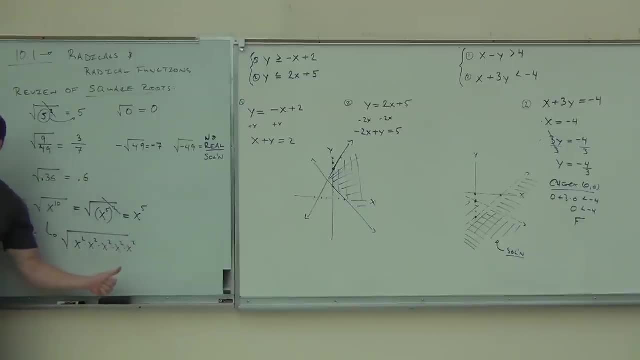 Yes, Is that still x to the 10th? to you? Yeah, x squared, x squared. We add up all those exponents right: 2,, 4,, 6,, 8.. That's x to the 10th. 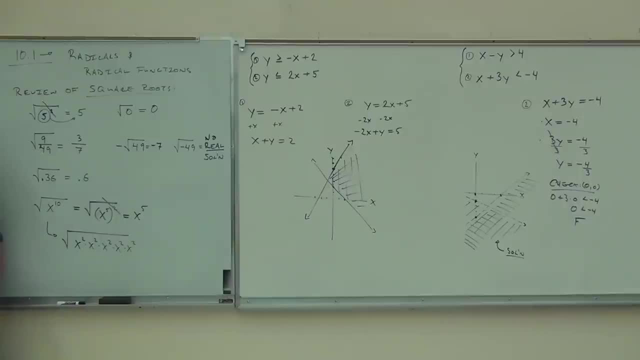 Not sure if you're agreeing. Okay, Do you see the Everywhere we have an x squared? why am I making x squared? What's my root out here? It's a square root. Square roots will undo your squares right. Everywhere we have an x squared. it will simplify out. 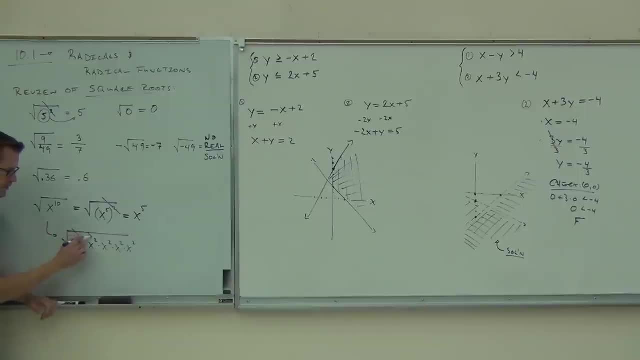 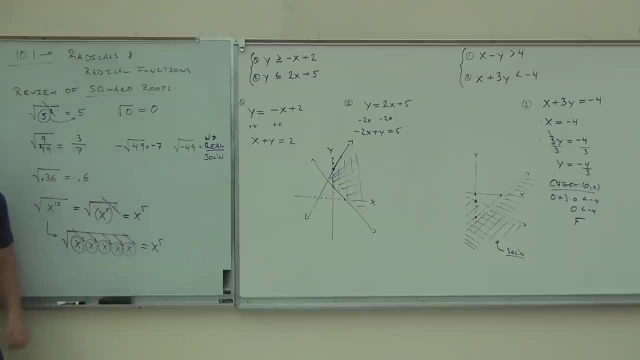 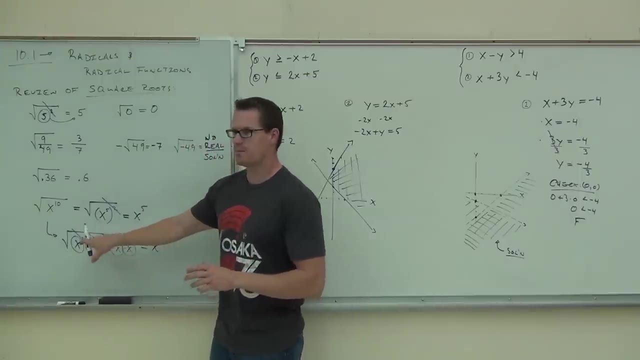 I'm going to have x to the fifth: Same answer, The same answer. Now you might be wondering: why in the world are we doing that? By the way, this works. I need to show you why this works. by the way, just a little note. 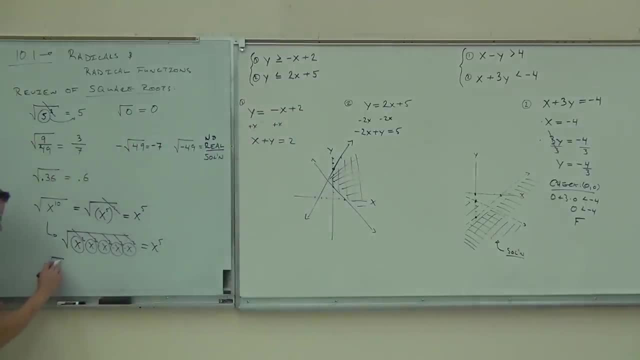 This works because you can always separate as x squared times square root of x squared times square root of x. You can do that as much as you want. You can separate that product into different x squares, okay, So each one, you can simplify that out. 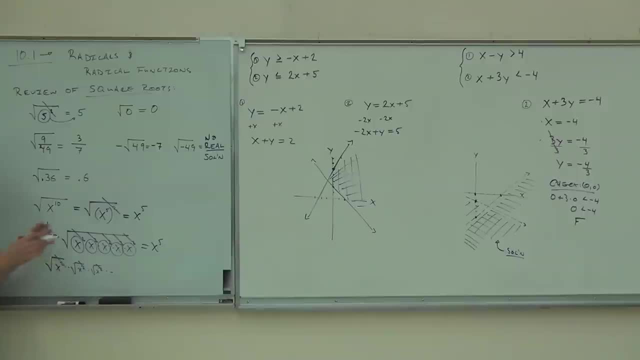 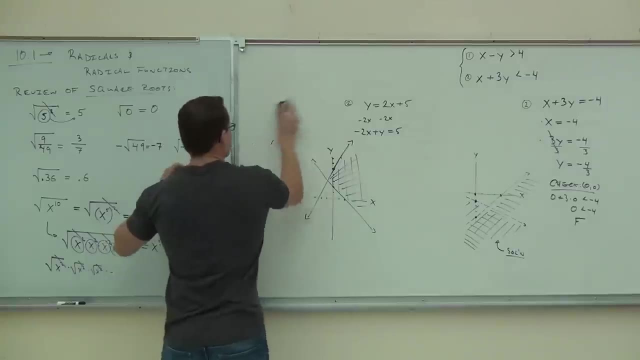 X, x x. You see the idea. You can do that every single time. Now, why are we doing this? Why, I'll leave that. That's a good little note. Why might we want to do that? This one seems so much quicker. 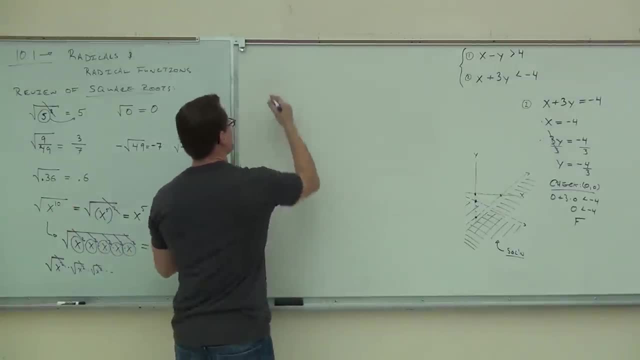 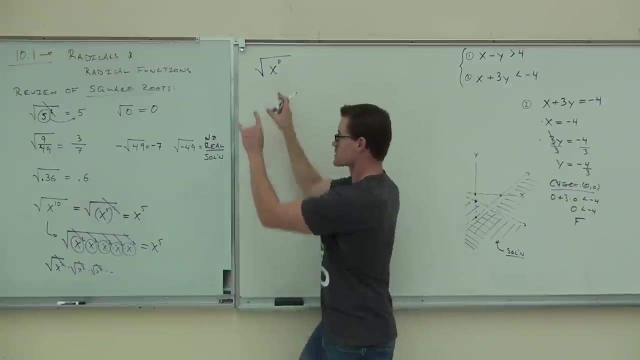 That's true, It does, But the question is: could you simplify this with that method? Can you simplify this with this method? Can you write this as what we did here is, we wrote this as x to the sum number times 2, right. 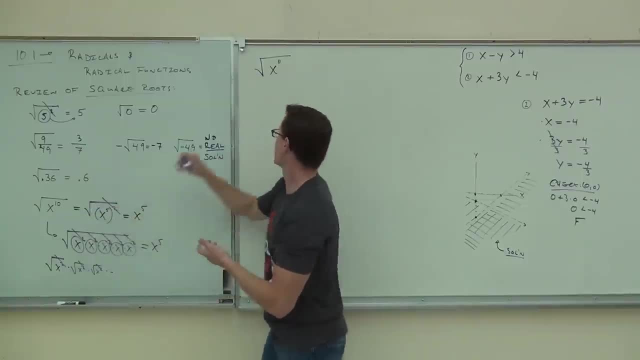 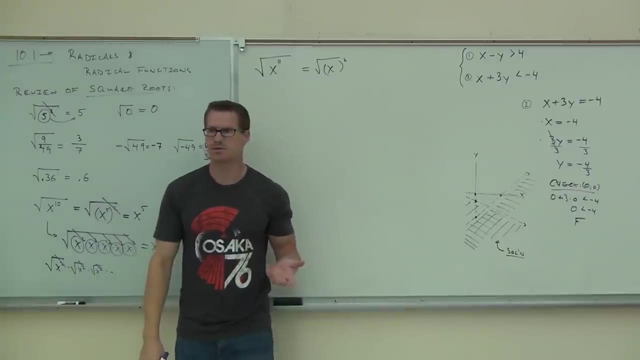 And that worked because this was equal to 10.. Can you write this as square root of x to sum number to the second? No, No, What times 2 equals 11?? No, Five and a half. Well, that doesn't really work so well okay. 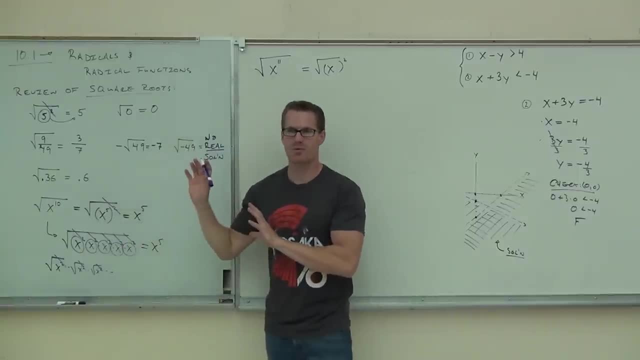 We can't do that. That's not going to help us out at all with this problem. So I had to teach you another way to do this. You see, using that method I can simplify this. I'm going to go a little bit ahead of where I'm supposed to. 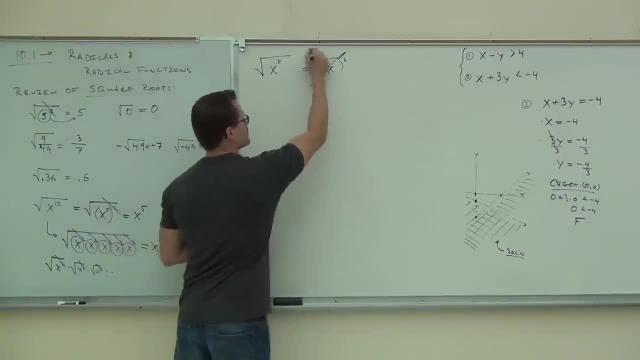 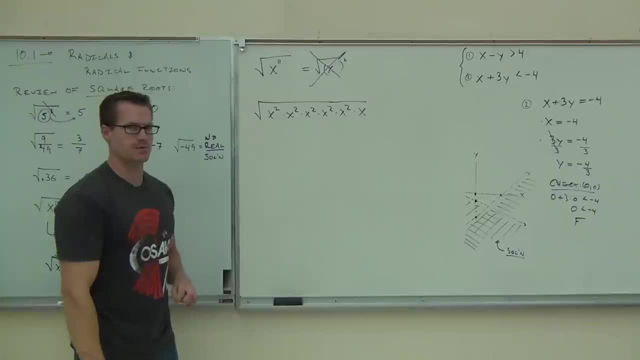 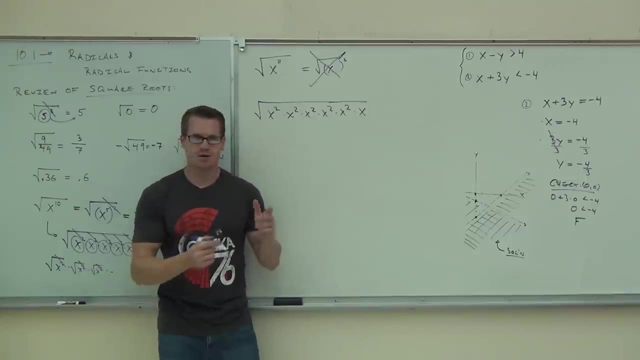 X. Perfect, Okay, Perfect. We're going to look at what simplifies out of this. This again: do you see why this simplifies, by the way, each of these? I could write this as a square root of x. squared times square root. 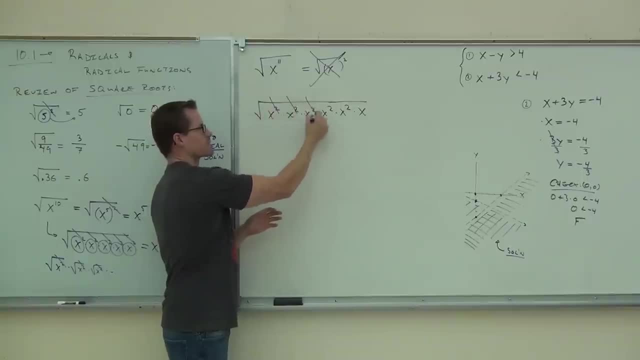 of x, squared over and over again. In each case, those squares are going to simplify, but this one does not. This one does not. I want you to look at what happens Whenever we simplify something that's going to go outside of our radical. 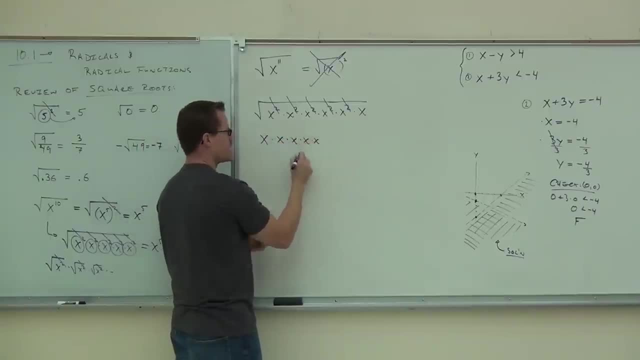 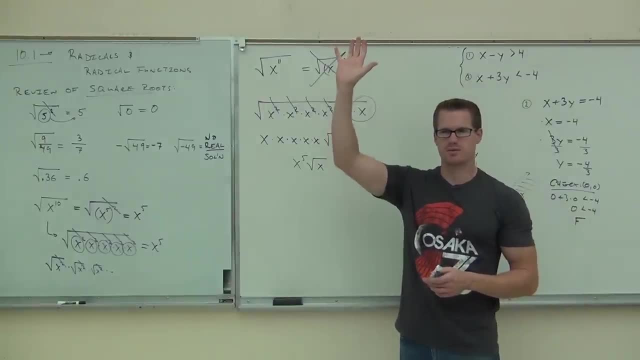 Yes, no. How many people are with me on that one? Not so much on that. We're going to come back to that. I just want to kind of preview that This is about two or three seconds from now. I just want to let you know that the reason why we're doing two different methods here is 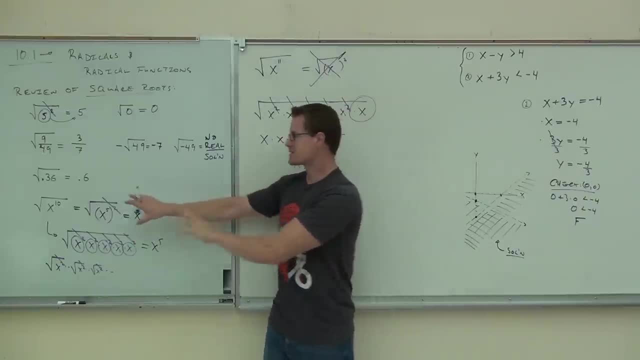 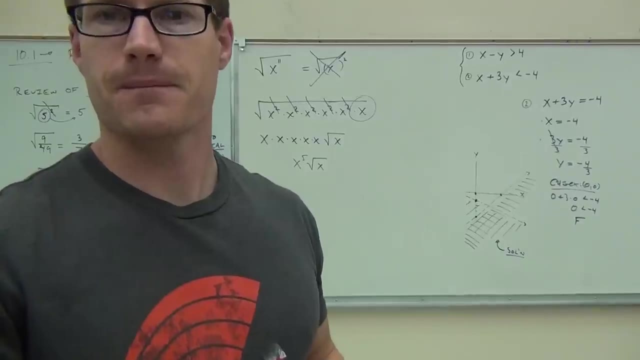 because we will eventually be dealing with stuff like that and I don't know if you're okay with at least this part of it. All right, we'll start this tomorrow and we'll finish that on the next one. So we're noticing that, in just like this situation, we could write this as something to the second. 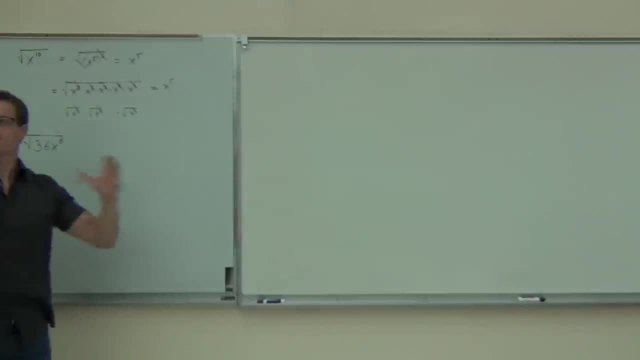 power. the square and the square root. They're inverse operations. They will simplify out of that expression and we're going to get just the radicand. Remember that was inside of our radical left. Or we could separate this as x squared times x squared. 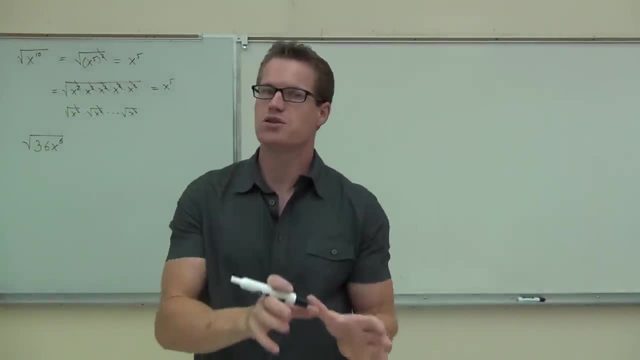 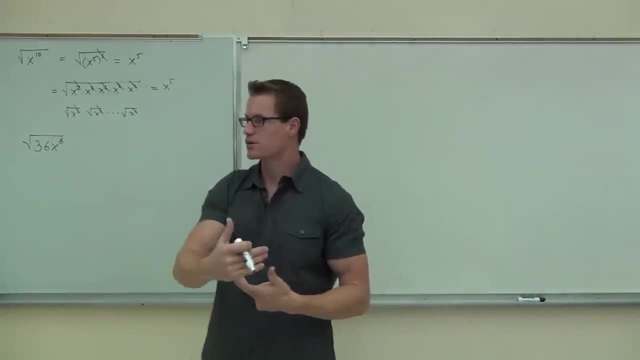 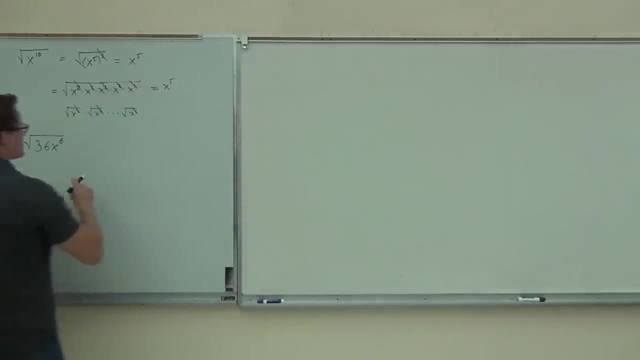 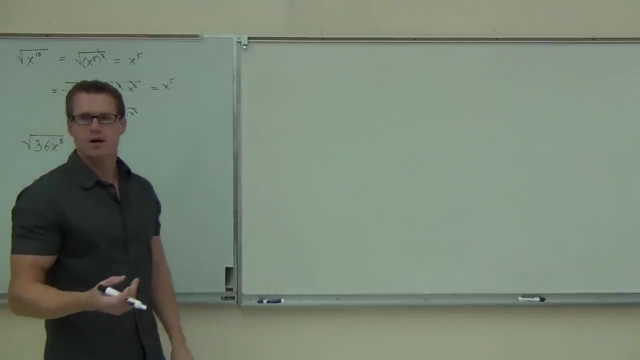 operations and we get just the radicand left over. We can do the same situation here, Even though we don't just have a variable. we have a number and a variable. we can do the same idea. What is the square root of 36?? 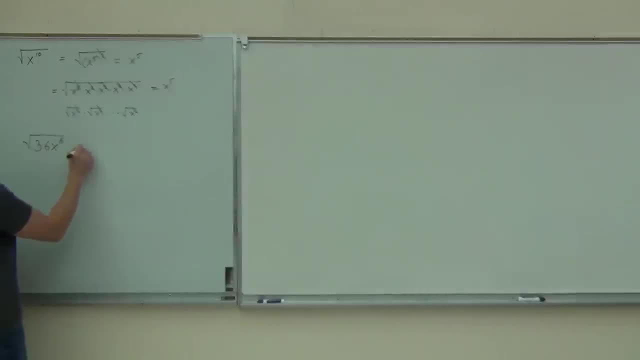 36.. Okay, So we could write that as 6.. Also, I'm going to leave that for now just 36, because I know I'm going to be able to take the square root in just a bit. Also, I need to deal with this x. 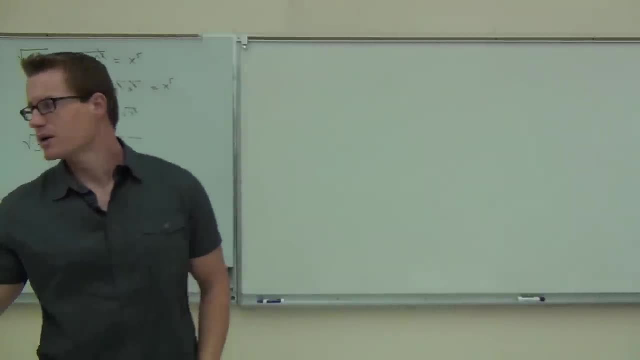 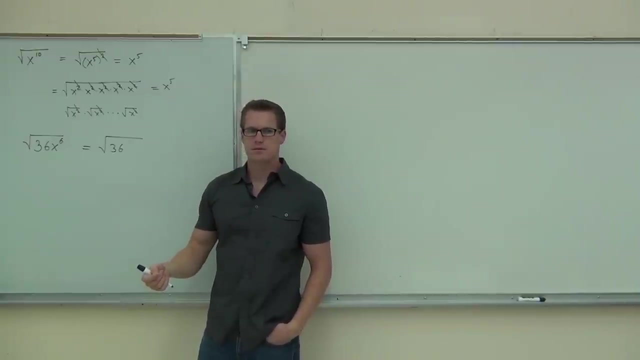 to the sixth power. Now, there's two ways to do x to the sixth power. We could do it like this: as something to the second power. How would I do that? Okay, so we're trying to write this as something to the second power. We're noticing that x to the first power is. 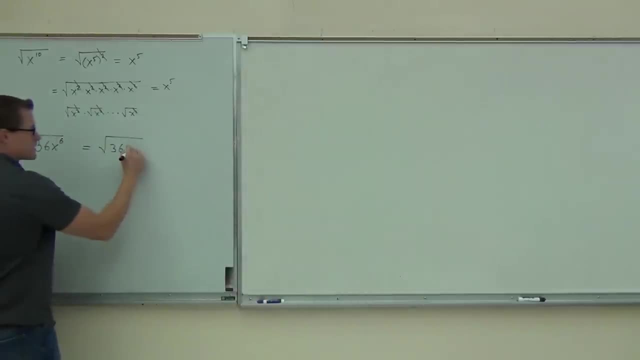 multiplication. So how do we write x to the sixth as something x to something squared, Of course? yeah, we're going to do the third. That was already said. Is that still x to the sixth? And now we can do the square root. Can you tell me what's the square root of? 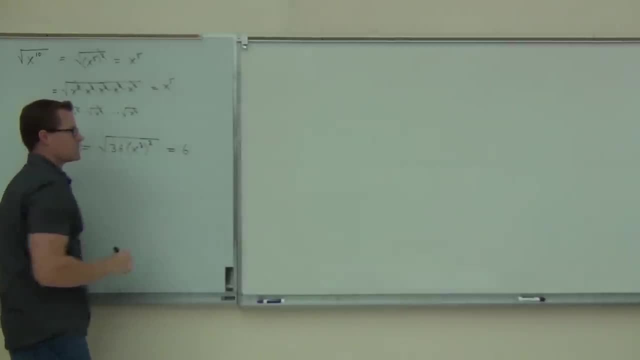 36? What happens to this square root and that square? What's going to happen there? Can you tell me what I'm going to have left over? Some of you are not with it today. You guys got to be with it. It's Friday morning, Let's go, Come on. So what's going to happen to? 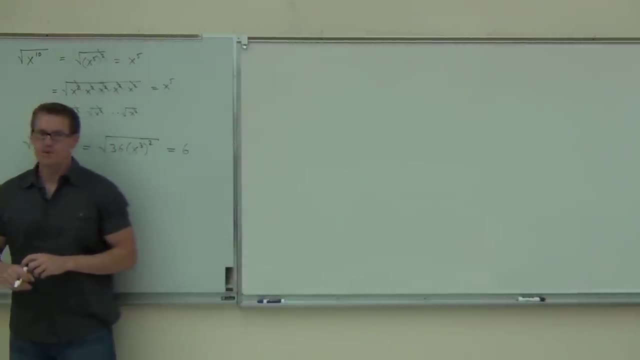 my square root and my square. What happens there? Okay, so there are inverses. They're going to be gone. What do I have left over? That's the answer. Now, if I did it the other way, some of you are going to prefer this. 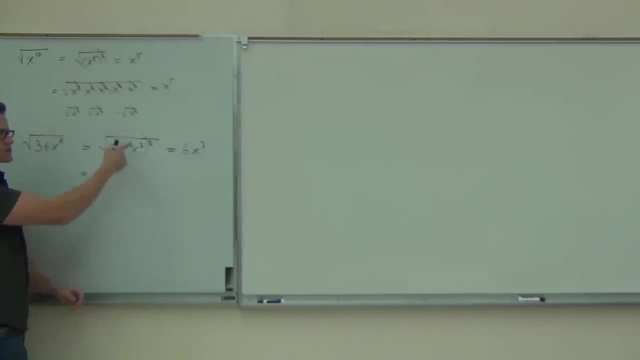 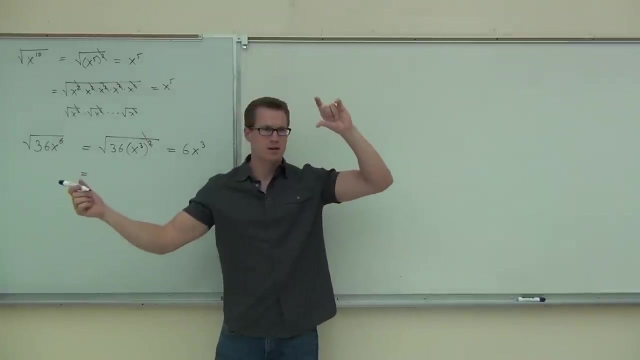 method, by the way, That's fine. I like that method. It works all the time. This one only works if you have an even power. If you have an odd power, does that work? You can't write it as something to the second, because something times two doesn't give you an odd. That's. 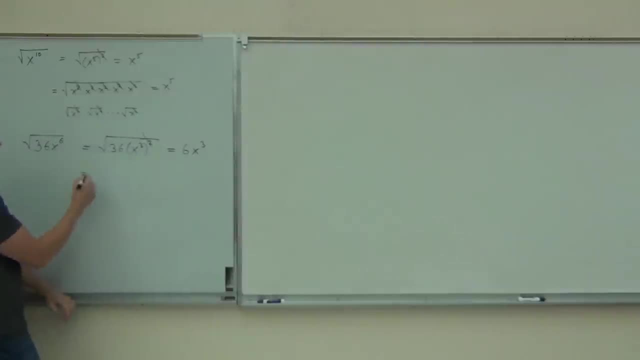 the problem. That's why we have to learn this method as well. So if we did it the other way, we could write this as 36.. And instead of x to the sixth, what I'd do is write it this as x squared, x squared, x squared, And you'll see that I can still take the 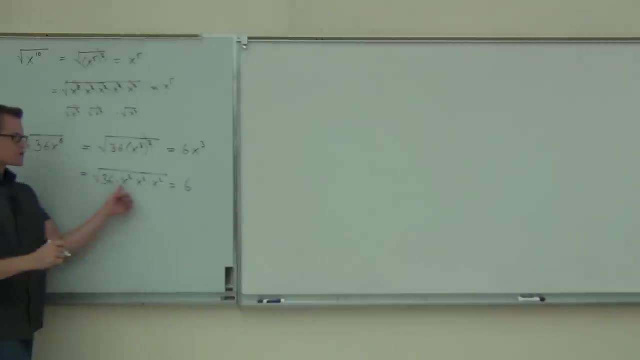 square root there. The square root of 36 is still six. Square root of x, squared. square root of x, squared. square root of x, squared. Notice how this square root, because I can separate it like that every one of those twos is going to be crossed out. The square 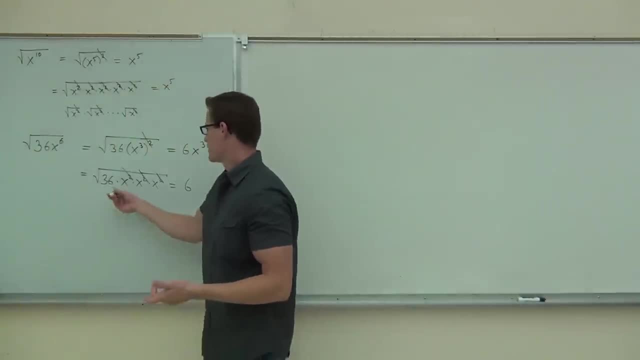 root is going to undo every one of those squares. And again, how many x's do I have left over Three, So I'm going to have x to the third. Either way, we do that, We're fine. How many of you feel OK with that? so far, Good deal, Good deal. Try a couple. 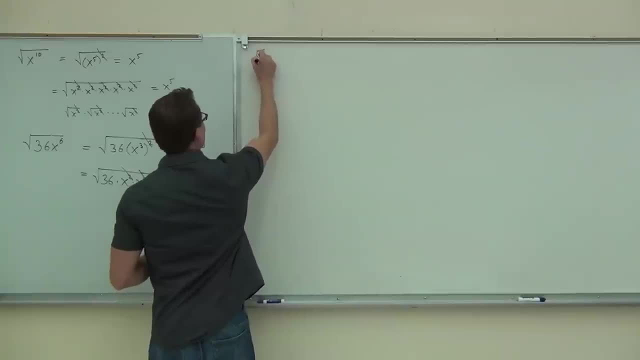 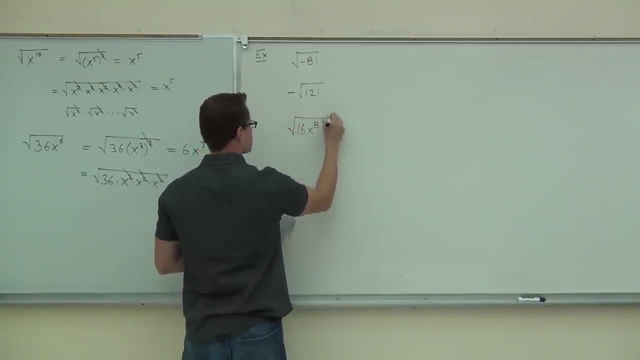 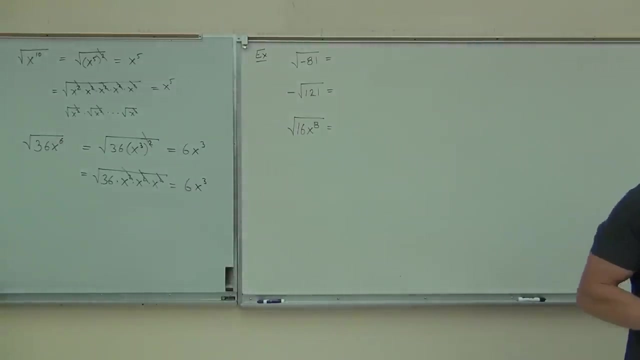 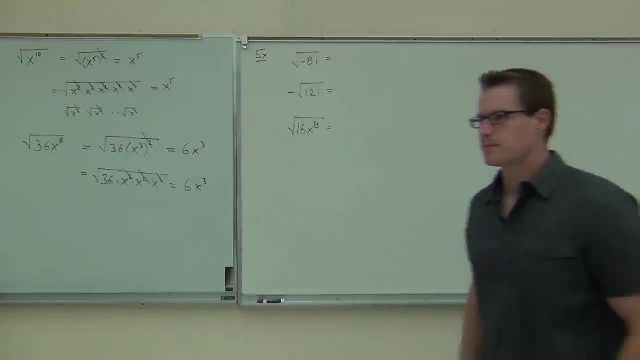 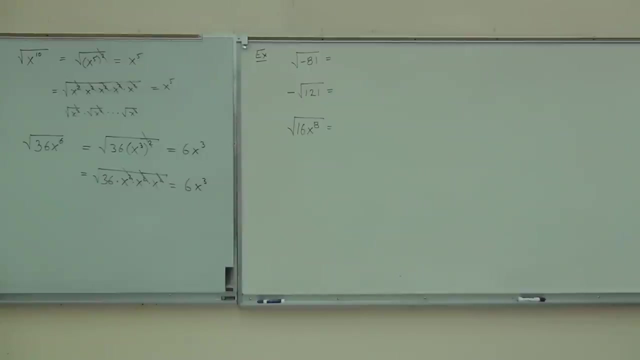 of these on your own. all right, So they don't take too long. Let's work on those. All right, so let's do all of them. What would you do? All right, Good, All right. So the first two are just some numbers. taking some square roots of those, if you can. 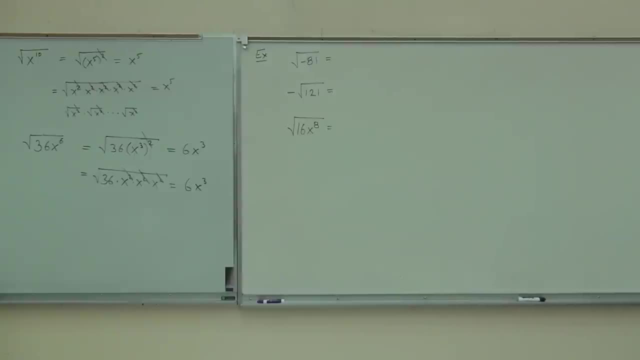 The last one. they have a variable in there. Use one of those two methods. You don't have to show me both, Just use one of them. I don't care which one. This one: Ultimately, we're going to be doing this or this. when we see these problems most likely. 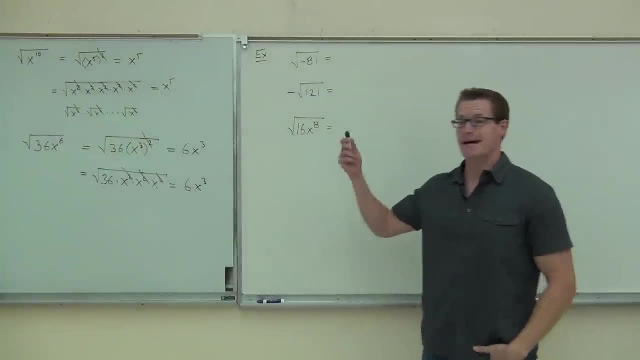 from here on out. So first one square root of negative 81, how much is that? No solution, No solution, No solution, No real solution. Yeah, we will have a solution on this in section 10.7, for sure. 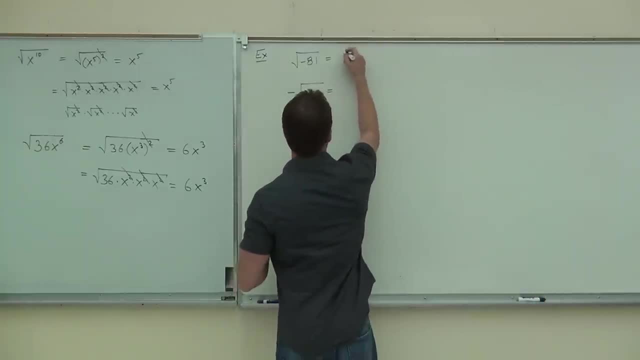 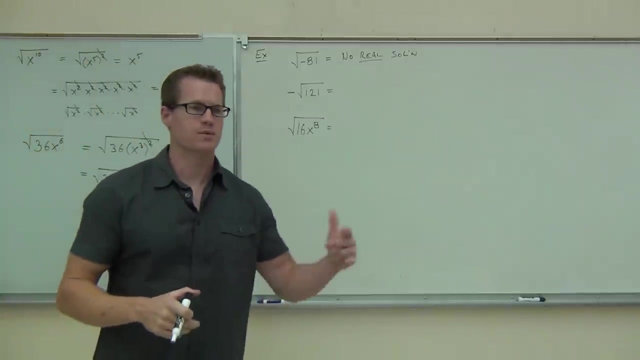 But right now we are dealing with real numbers. we have no real solution. Why no real solution? What's the matter there? Yeah, We know that a number times a self cannot give us a negative. So if the radicand is negative inside of a square root, we can't do it, not in the real. 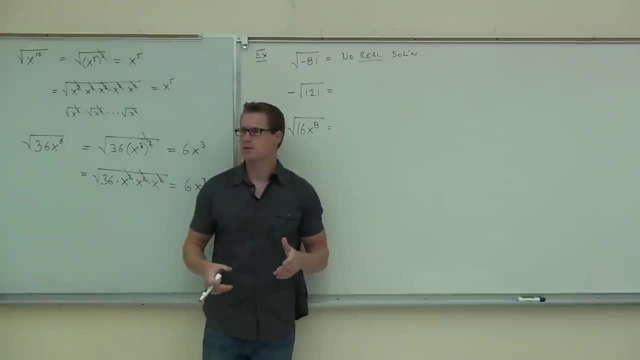 numbers at least Negative. square root of 121, how much is that, folks? Yeah, that's exactly right. And 16x to the 8th. we're going to do this process over here, one of these processes. So we know the square root of 16 is how much. 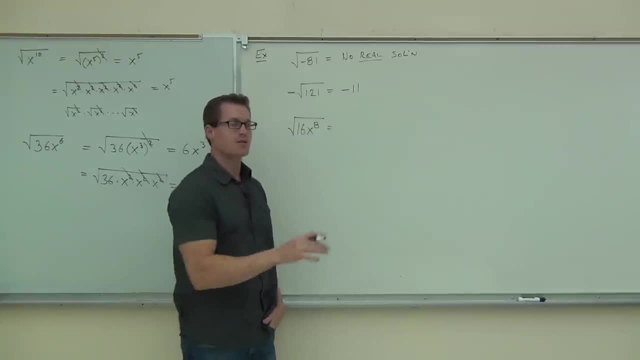 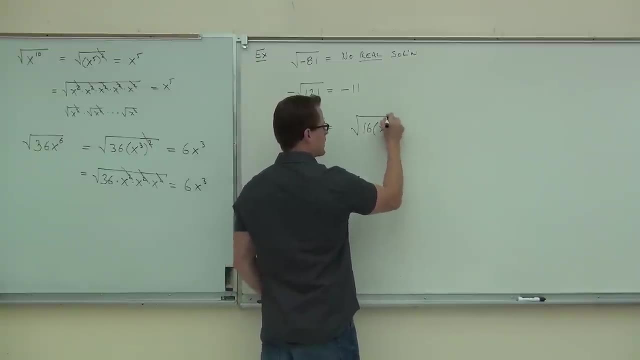 One. Okay, that's not bad- The square root of x to the 8th. we have to write this a certain way. Either you're going to write this as 16.. X to the 8th. X to the something raised to the second power. 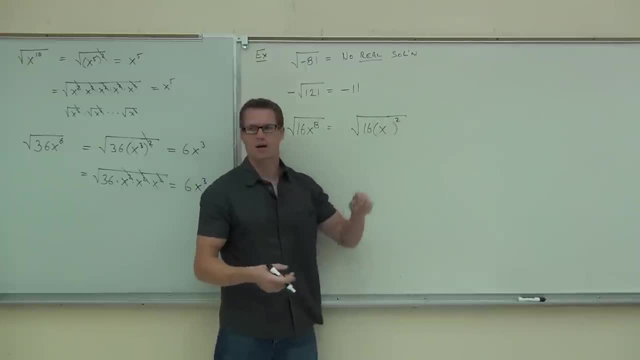 We're choosing the second power because we know a square root and a square are inverse operations. That allows us to simplify that. I'm not sure if you're with me on that. So we're choosing the second power because it's a square root. 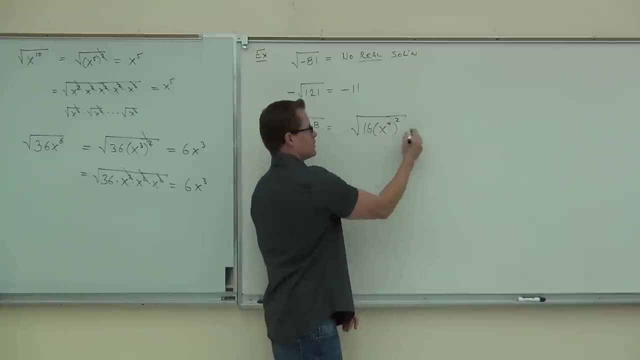 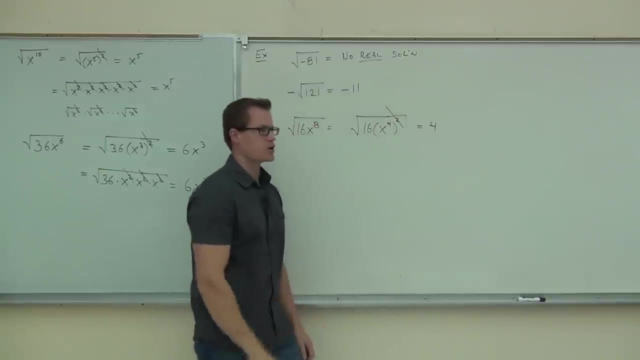 What has to go in here to make that true? So we do. square root of 16 is 4.. Square root of x to the 4th to the 2nd. that's going to simplify out of our expression. We're going to get x to the 4th left over. 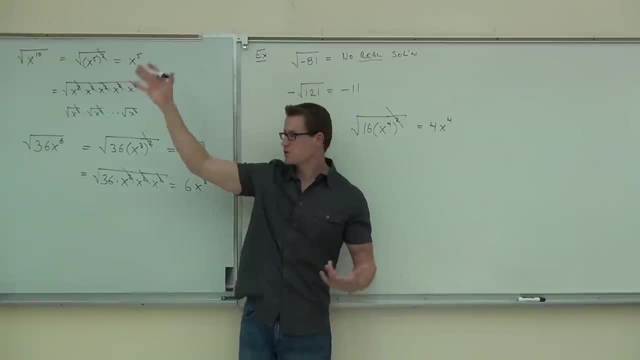 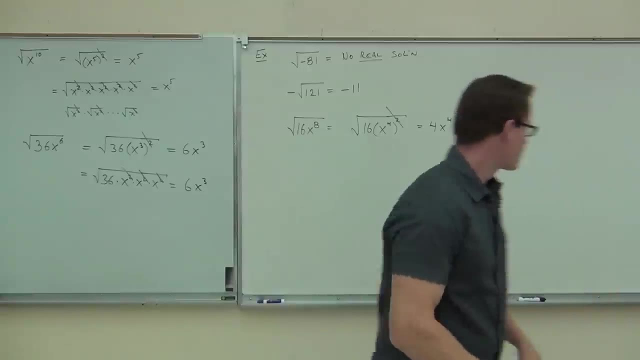 Raise your hand. if you got that, Okay, Good. If you want to do it the other way, that's fine. If you want to do it the other way, that's fine. What we're going to do is still write this as 16, except instead of x, to the 8th you. 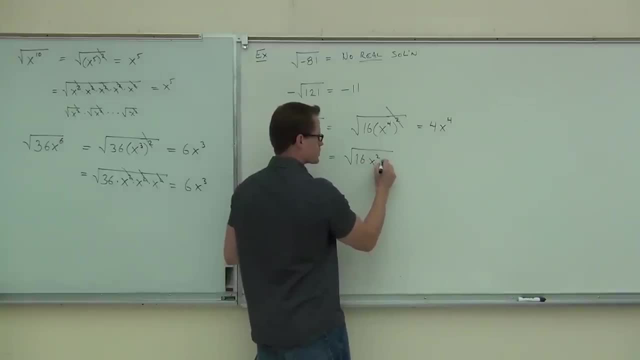 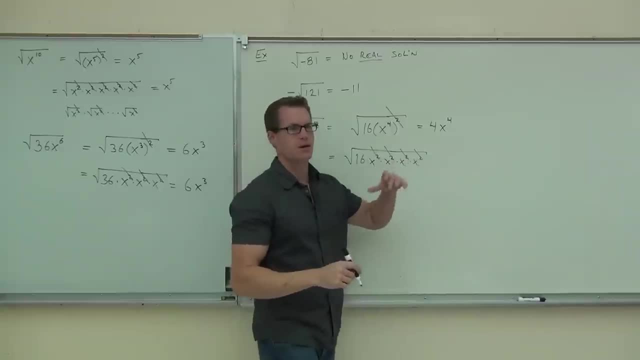 this as square root of x squared and square root of x squared, over and over again. So still, we get: square root of 16 is 4.. We have x, x, x, x, That's x to the 4th. 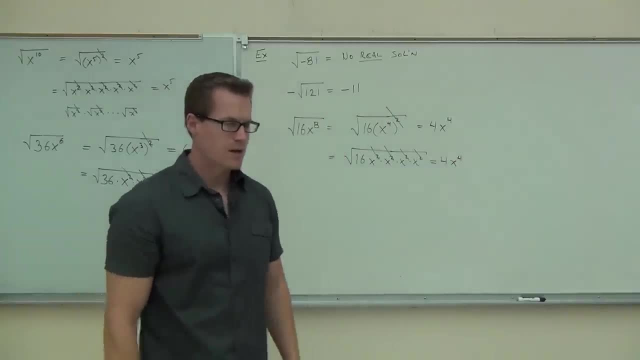 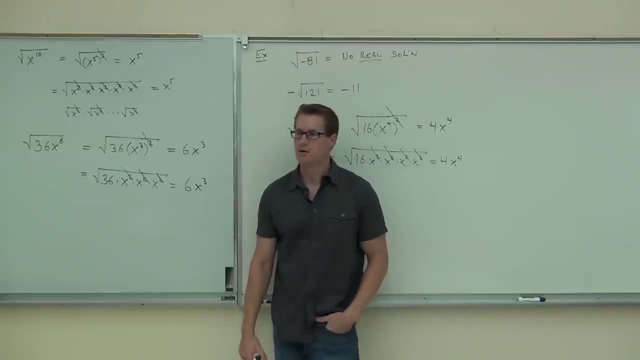 Either way we do that, we get the same answer. Hey, by the way, let's do a little practice on this. What's the square root of 81? Nine? How about the square root of 64? Eight, Twenty-five. 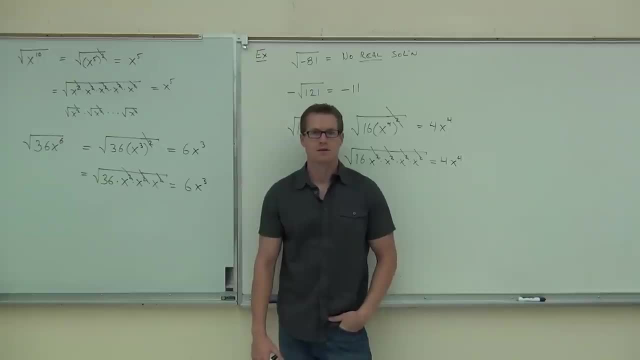 Five, Forty-nine, Seven, Thirty, Thirty, Does it exist? Yeah, Okay, So it's not just that there's only like ten square roots for the first hundred numbers, right? I mean, is it just that you take square root of 1 and 4 and 9 and 16 and 25 and nothing else? 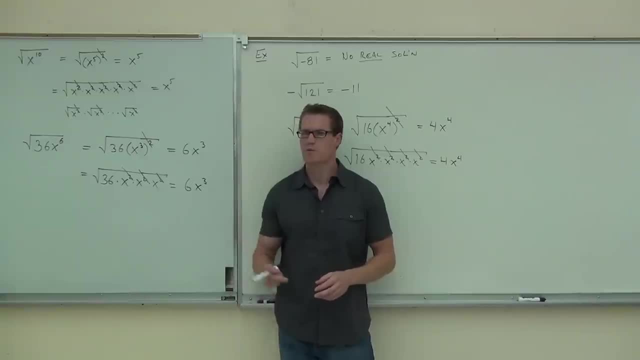 No, no, no. It's just that when you take the square root of those numbers, you're able to give me the whole number, which is why you're able to do it quickly. right? You go with square root of 25, you go 5.. 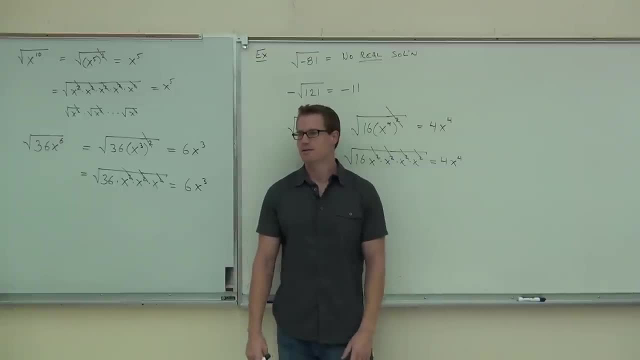 With square root of 49, 7.. Square root of 30.. I have no idea, I don't know Why, Because it's not. what is that number known as? where it's 1,, 4,, 9,, 16,, 25,, 36,, 49,, 64?? 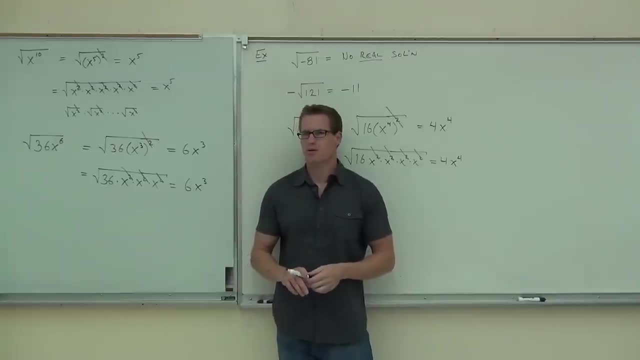 What are those numbers? What are those? Well, why? Why do those ones work? Think about it. Why do those numbers work? Okay, what's that known as in mathematics, When you multiply a number by itself and it gives you something? 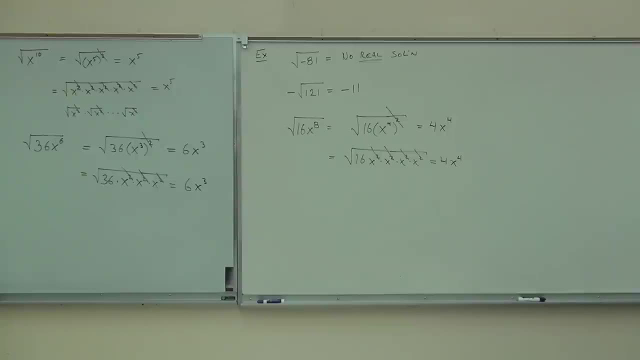 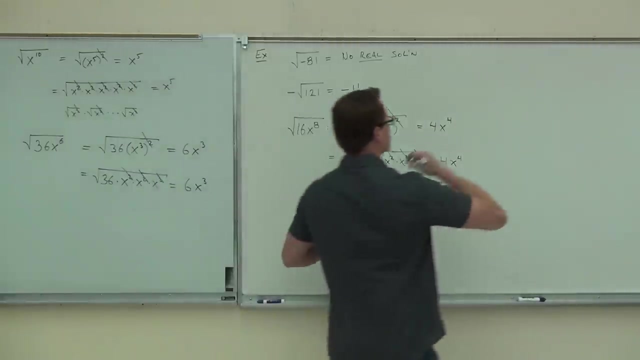 Say it again: No, not a prime number. A prime number would be a number where only 1 and the number itself divides it. So the number is 1.. Can you take the square root of 1?? Sure, it's 1, yeah. 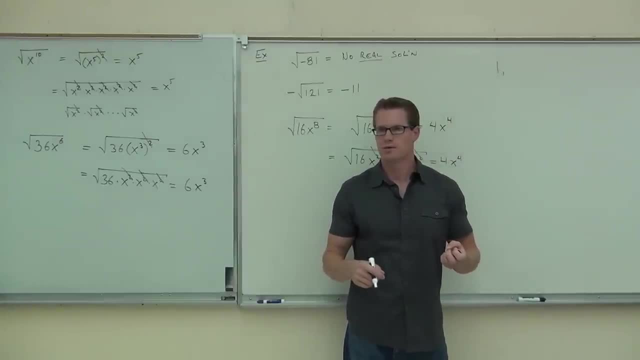 What's the next number? you can take the square root of, and it's a whole number: 4.. Yeah, not 2, right, Square root of 2.. Square root of 2 is, I don't know how- about 3?? 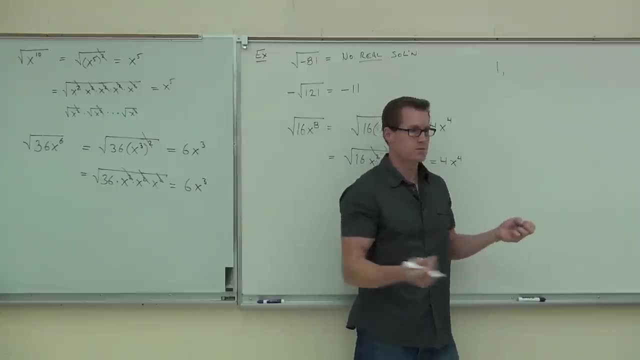 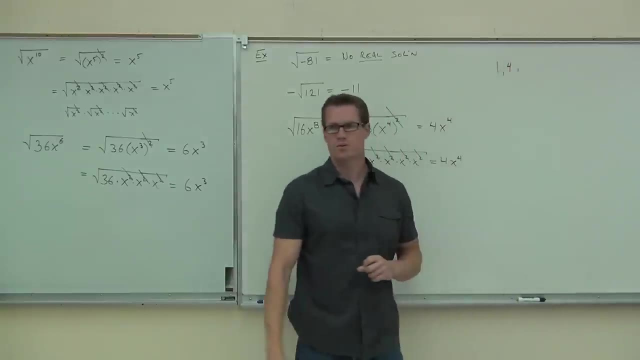 I don't know How. about 4? 2. Great, okay. What's the next number you can take the square root of easily: 5?, 5? No, 6?, No, 7?, 8?, 9?. 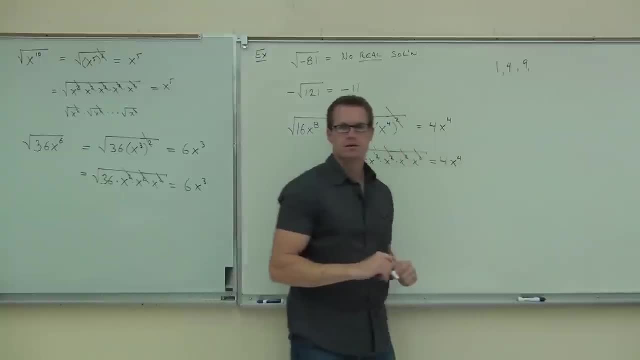 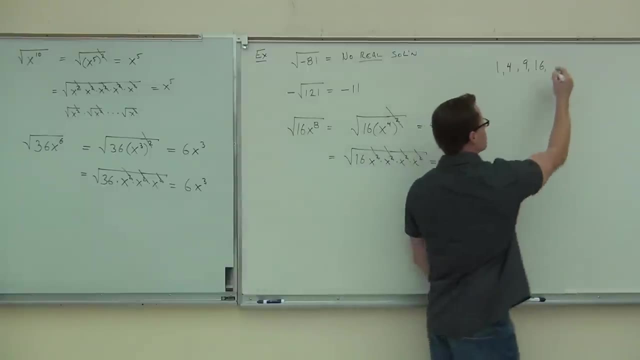 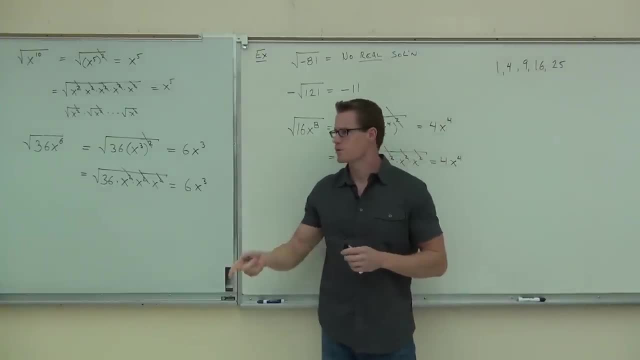 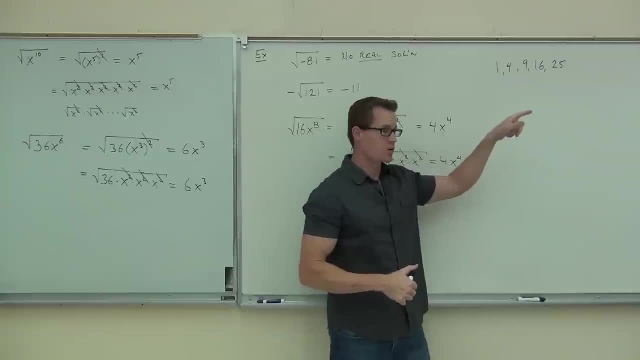 How are you determining that? Are you just guessing and checking, or is there an easier way? By the way, what's the square root of 1? 1. Square root of 4? 2. Square root of 9? 3.? 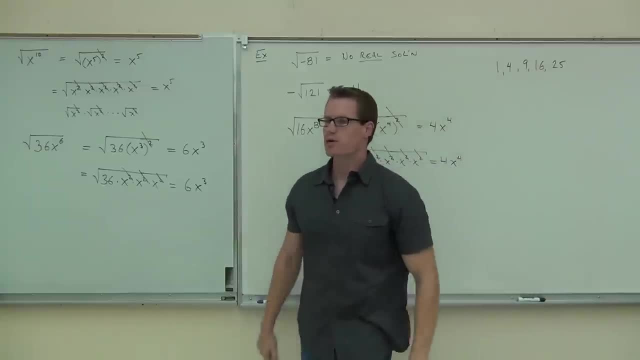 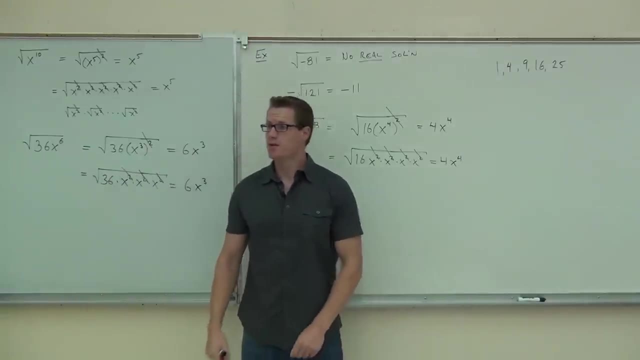 4., 4.. 5.. Okay, what are those numbers? How are you getting those numbers from 1,, 2,, 3,, 4, and 5?? How are you getting those numbers? Multiply them together, Okay. in other words, instead of just multiplying them together, how else could I say that? 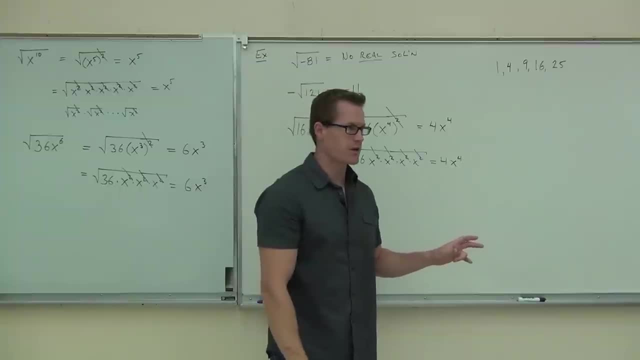 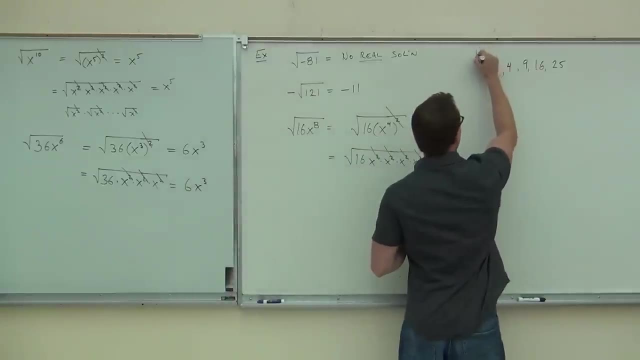 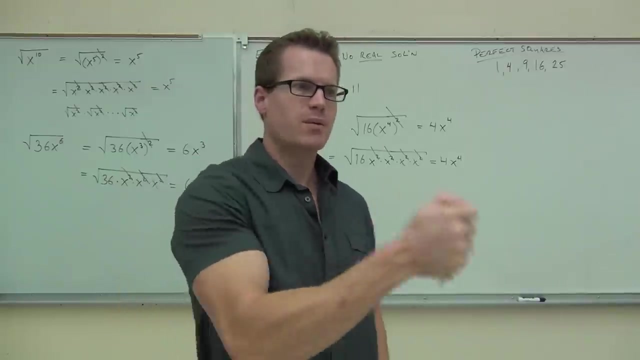 Squaring it. These numbers are called perfect squares. Have you never heard of that before? A perfect square is a number that is an integer times a self- Perfect squares. So a perfect square that's that number where you take a number times a self. 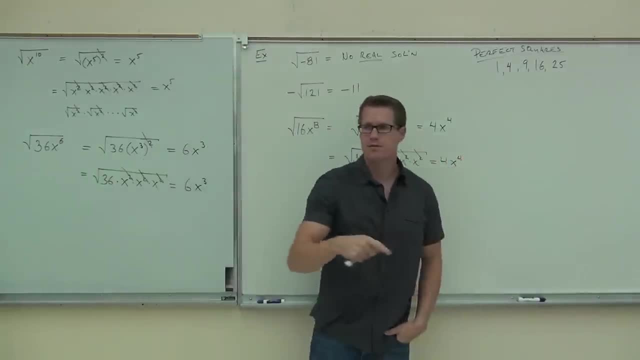 You get one of those right, You get 1,, 4,, 9,, 16,, 25,, 36, and so on, and so on, and so on forever. Those are also the numbers where I can take the square roots of easily and it gives me 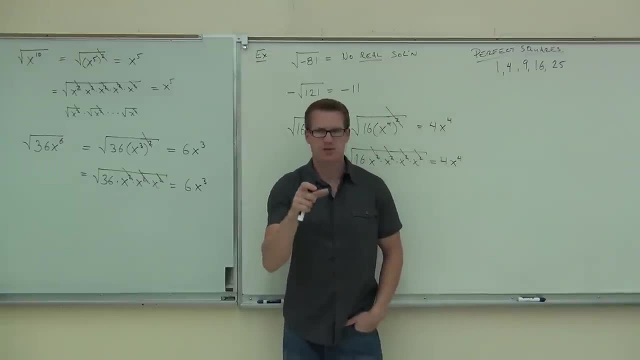 a whole number answer. The reason why is because we know that a perfect square is a number times a self right, So if I'm undoing that, it's going to give me that number back again. And a square root and a square are inverse operations. 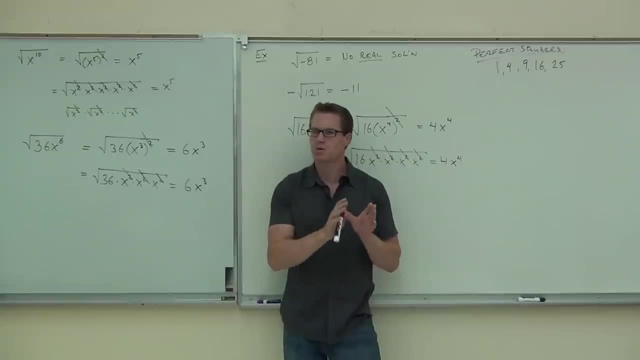 So these are the only numbers that you can take a square root of and it gives you a whole number answer If you don't have a perfect square, such as when I said what's a square root of 30 and you all went: I don't know. 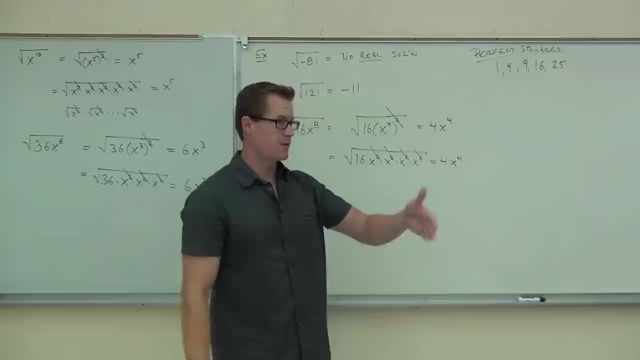 It's somewhere between 5 and 6, probably between 25 and 36, right, So it's somewhere between 5 and 6. But I don't know exactly how much it is, and that's because it's an irrational number. 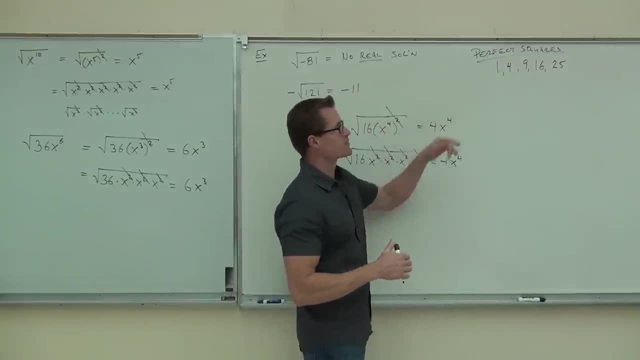 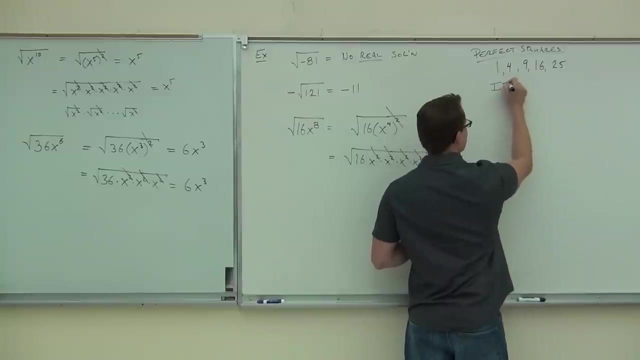 So every time you take the square root of a number that is not a perfect square, you're going to get an irrational number. That's a number that is represented by a decimal. that's not ending and not repeating. If you take the square root. 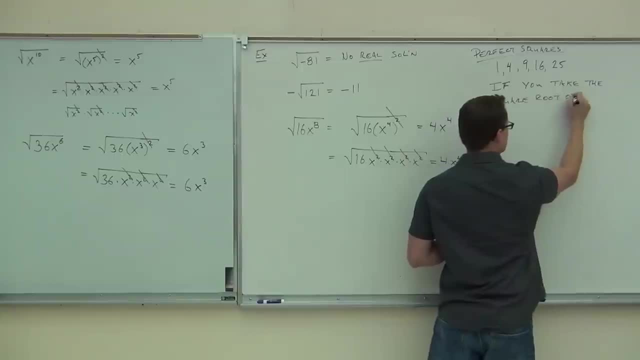 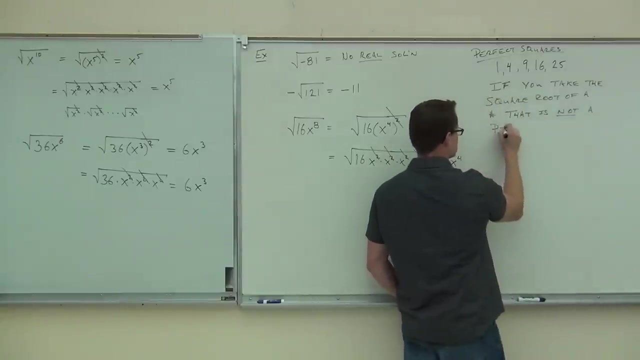 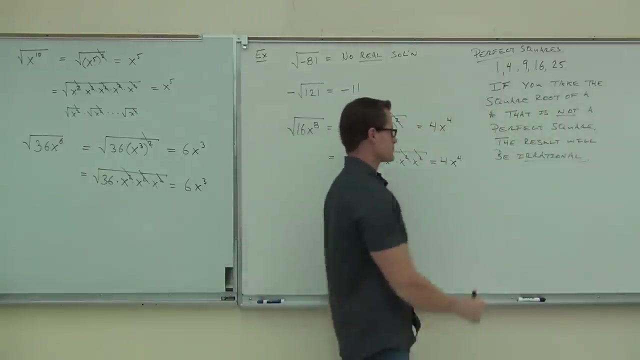 Of a number that is not a perfect square. It's a number that is not a perfect square. So what does that mean? It's a number that is not a perfect square, So Okay, The result will be irrational. Let's look at the square root of 30.. 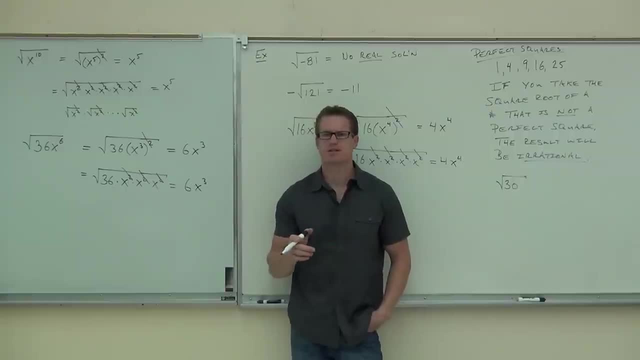 Seriously. I said that this number is between 5 and 6, and how did I know that? Well, let's look at that. Do you know the square root of 25?? Do you know the square root of 36?? If this is between 25 and 36, then we know that the square root of that number has to be between 5 and 6.. 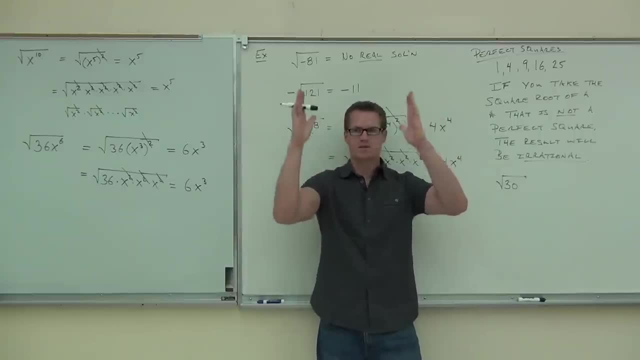 Does that make sense to you? So it's kind of squeezing that. It's squeezing it between two bookends. It's saying: well, this one equals 5,, this one equals 6.. If there's something between there, the answer has to be between 5 and 6.. 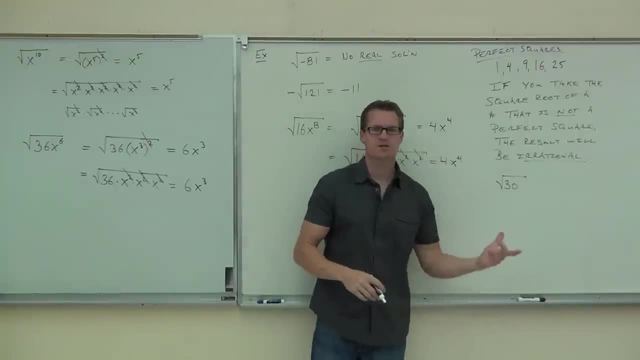 That's the way that works. So I know this is between 5 and 6.. This is somewhere between 5 and 6, but I don't know exactly how much it is. There's methods to do this, like by hand, to find out exactly how much the square root of 30 is to whatever decimal place you want. 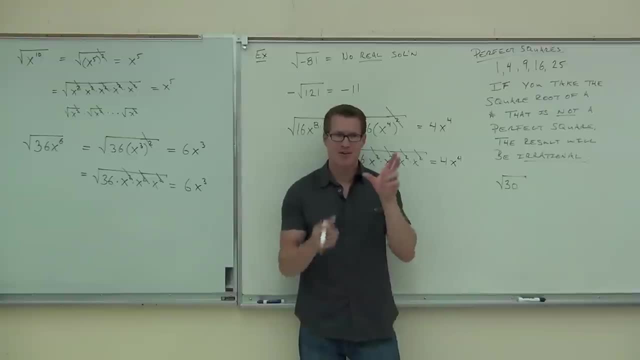 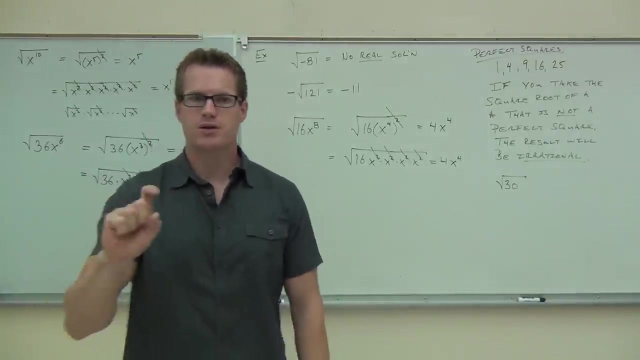 but it's very hard to do and we have these nice little things called calculators which do it for us. Take out your calculator. if you have, one Square roots can be found on your calculators. Now I've got to warn you that when you find a number on your calculator, that's a square root. 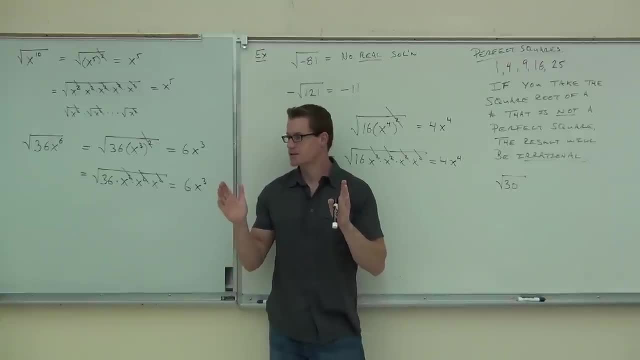 it's given you, like the first, 10 or 12 digits. That's not everything. This number will go on literally forever. It does not end, It doesn't repeat. You cannot represent it as a fraction. That's what irrational means. 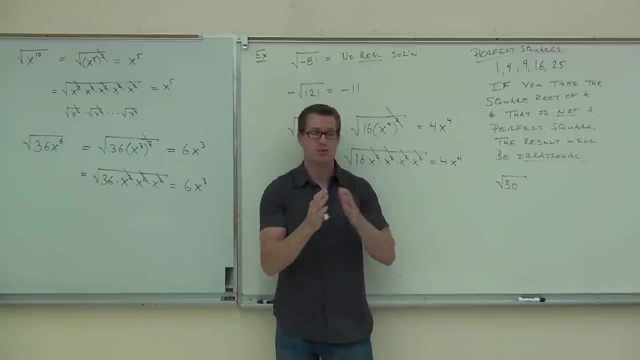 Rational means fraction. Irrational means cannot be represented as a fraction, So this thing doesn't end. It goes on to millions and millions and millions of digits long. okay, It's not a huge number, It's only between 5 and 6, but the decimals go on forever. 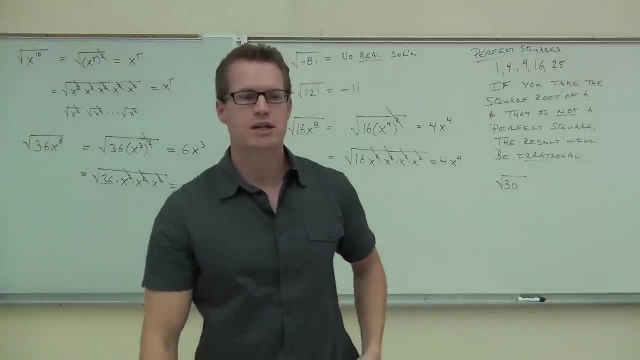 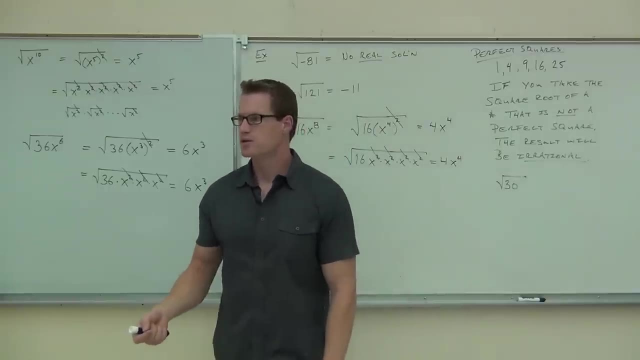 So here's how you find your calculator. The first thing I need you to do: find the square root. Find the square root button. It looks like that It might be a second or a shift button, So find that on your calculator, if you have a calculator. 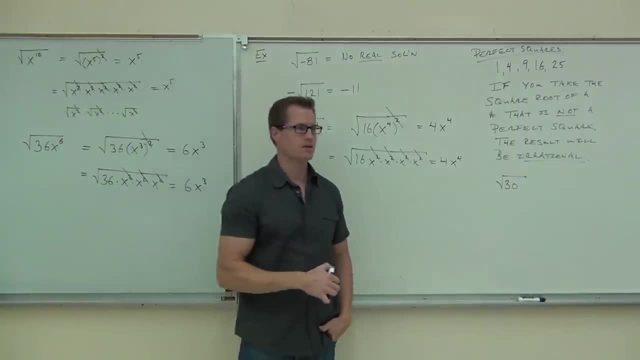 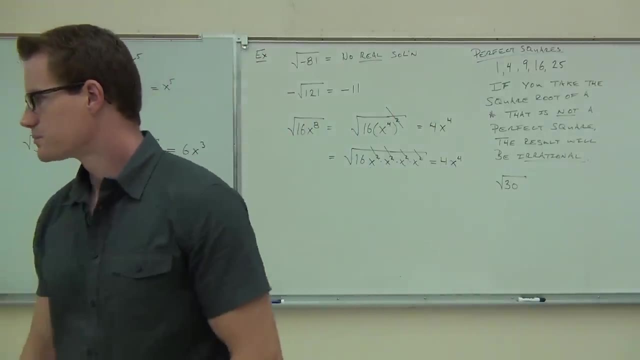 If you don't have a calculator, look at someone who has a calculator right now. You need to be seeing a calculator, okay? So if you don't have one share, Find your square root and what it wants you to do is press your square root button. 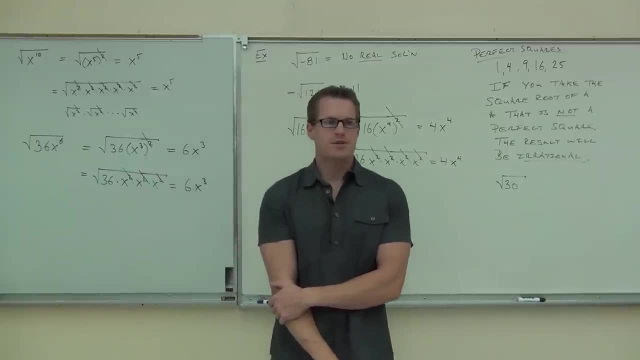 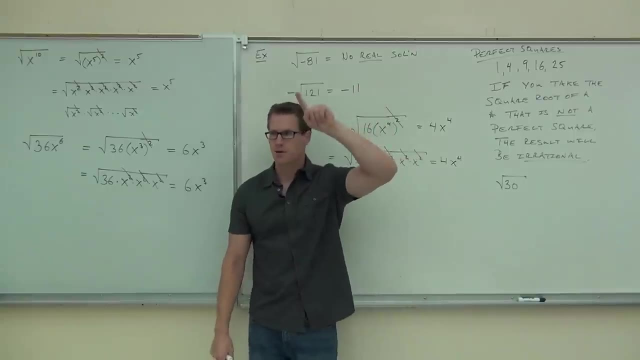 Press your square root button right now. When you press your square root button, if it came up and you have now a square root on your screen, that's great. If you are one of those people, raise your hand. If you press the square root button, you have a square root on the screen. 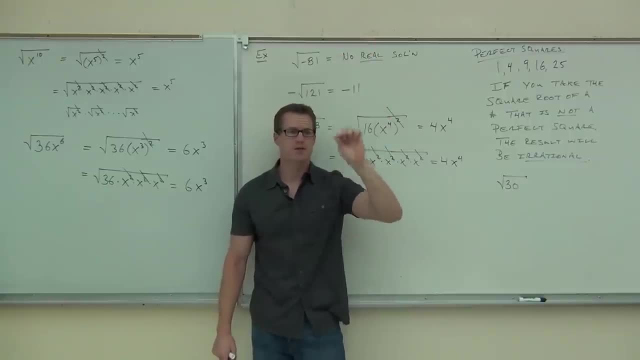 Okay, you people are going to press a square root first, then your number, and then press equals. Okay, that's what you people are going to do. So you press your square root, The square root will pop up, Then you press your number. 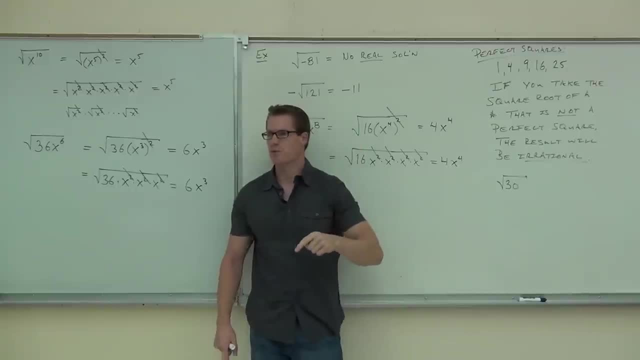 Press some 30 right now and then press equals. You should get 5 point something. Do you guys have that? if that was you, Okay, If you press your square root and then it still popped up zero, You are one of two cases. 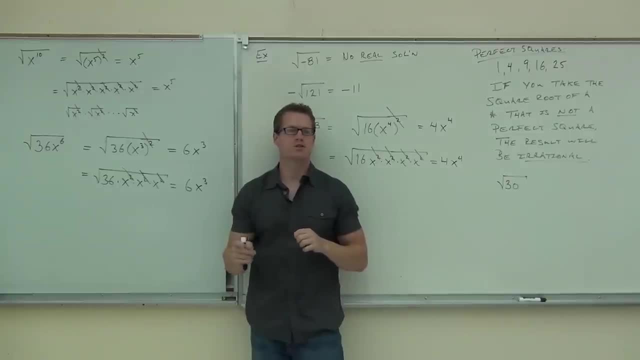 Okay. so if you press that and it popped up zero, what you have to do is press your number first and then press your square root. So press zero and then press- it's probably a second button or shift button- and then your square root. 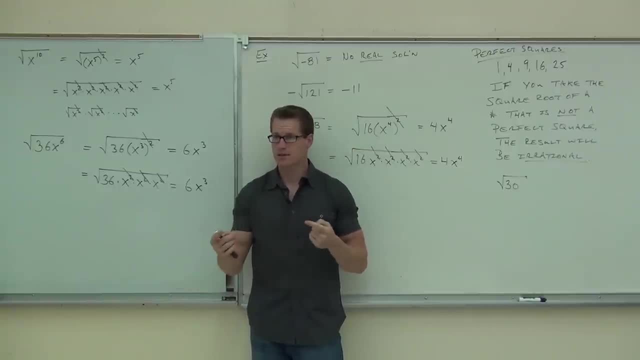 And you should get the 5 point, something on that. In either case, did you guys get that Okay? how many people have a calculator? Raise your hand, And how many of those people were able to find the number Okay, good. 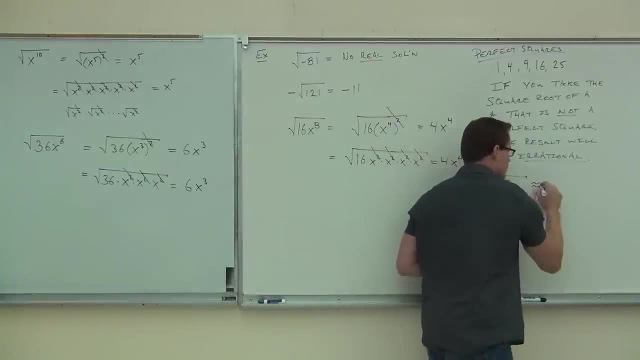 That's everybody. That's fantastic. Now tell me to the third decimal place, what is square root of 30? 5.477.. 7, 7, what 2, 2, 5.. Okay, so we do need to round appropriately. 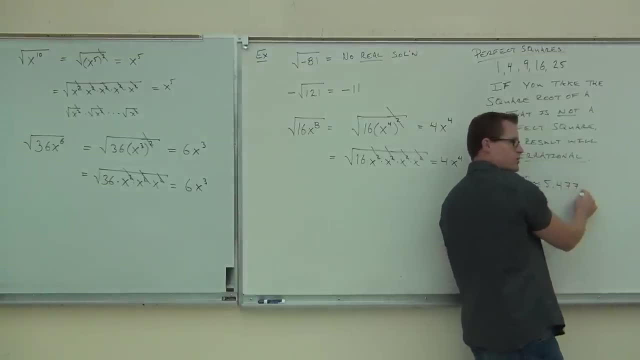 So if I say third decimal place, I mean 5.77.. If that number is a 2,, then we leave that number alone. If this was 5 or more, then we would have moved that to an 8,. yeah. 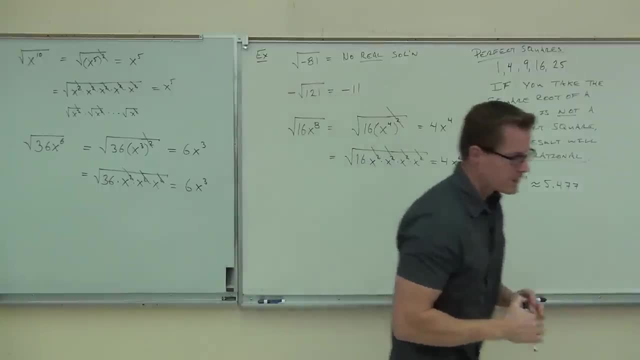 Okay, so round that appropriately. Try one more for me. Let's do the square root of 45.. Before you do this on your calculator- I want you to, unless you've already done it- I want you to think of what number this is between. 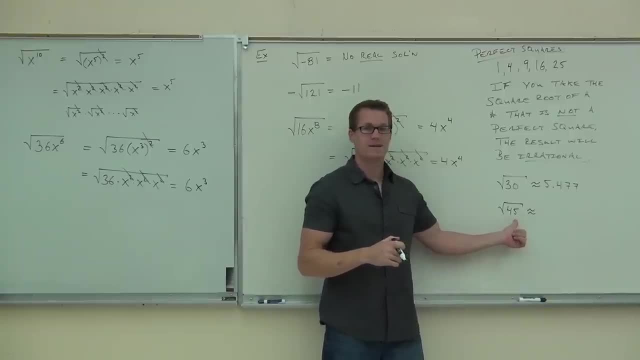 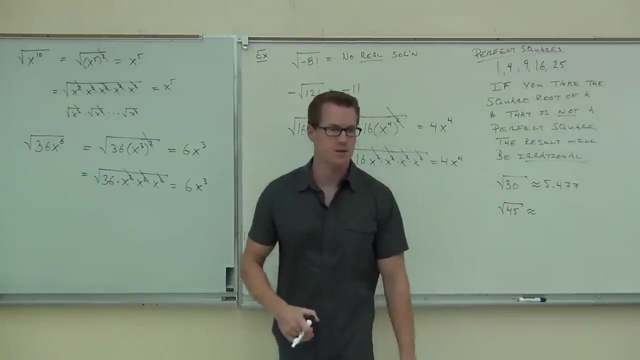 What number that is between. Why 6 and 7?? Perfect, yeah, This is between those two values: 36 and 49.. Square root of 36 is 6,, 49 is 7.. Therefore, it has to be there. 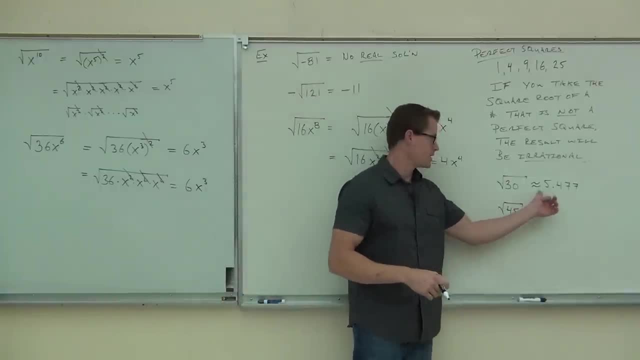 Very good. How much is that? Not exactly because we are approximating. By the way, that's what that squiggly equals means. It means it's not exact because we're rounding, we're approximating here. How much is that? 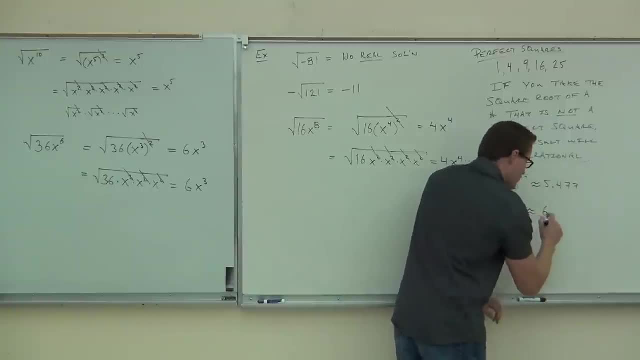 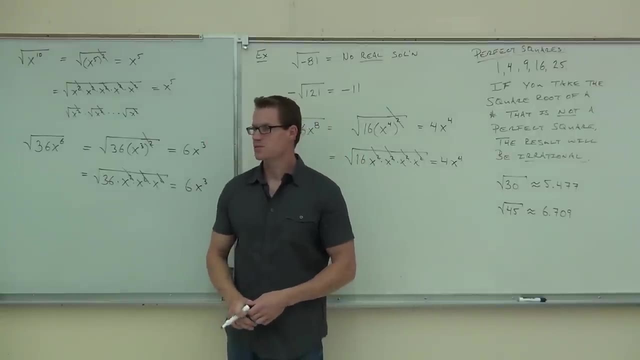 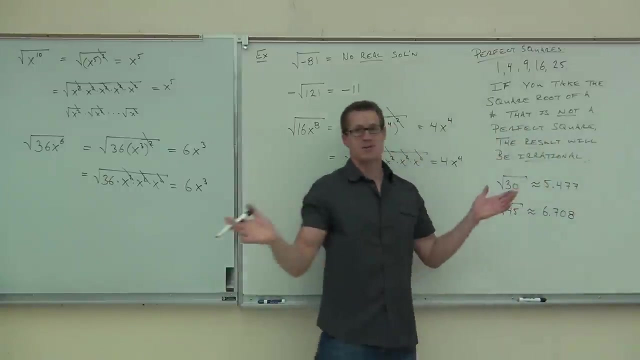 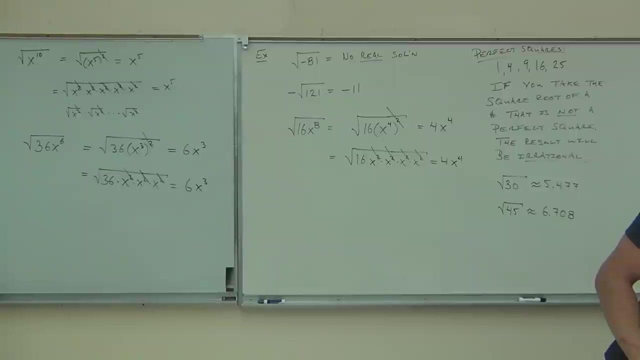 6.9. 6.. what? 7.9. 7.9,? all right, Hey, I just write what you guys say. all right, That's what my job is. That's it. How many of you feel okay finding this on the calculator? 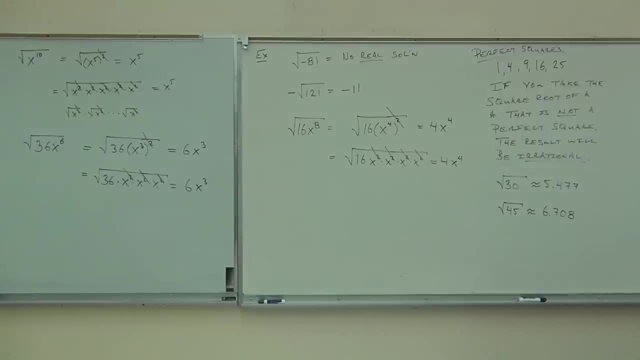 Good, good deal. You know we've covered square roots. Do you feel okay about square roots? At this point you should be able to find the square root of any number I give you. If it's a perfect square, it's pretty easy. 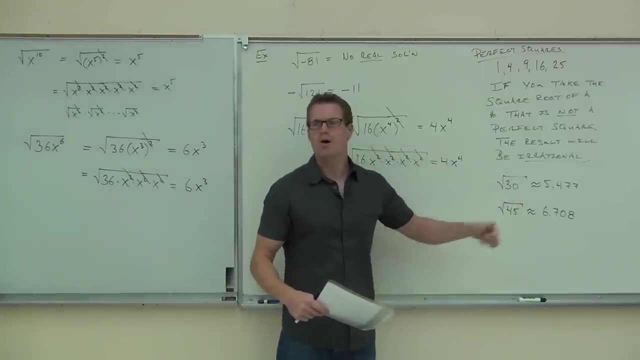 It's just like 4.. If it's not a perfect square, right now all we have is a calculator method. Now I'm going to teach you a method in a little while, a couple of sections from here where we can simplify these numbers to get something that's still radical. 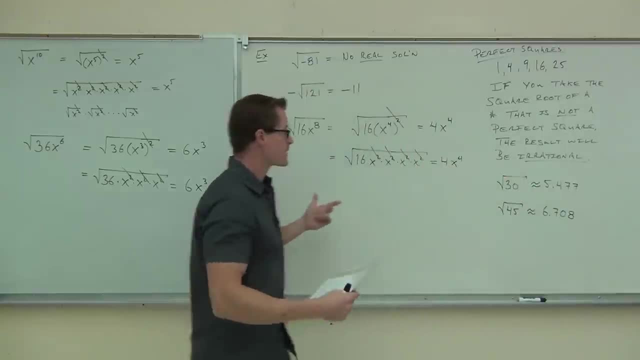 but we can make the radicand smaller by simplifying. very similar to this idea and very similar to that. You also should be able to simplify any variable that I give you in there now: x to the 10th, x to the 6th, x to the 8th. 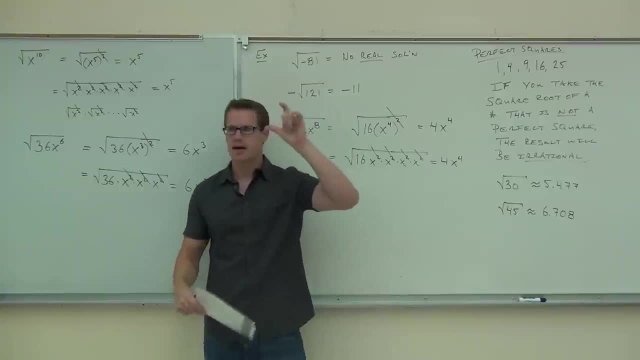 Right now we haven't done any odd power yet, but we'll get to that. This is the method that we would use for that. That's why I kind of preview that information. We should be feeling pretty good about these square roots. 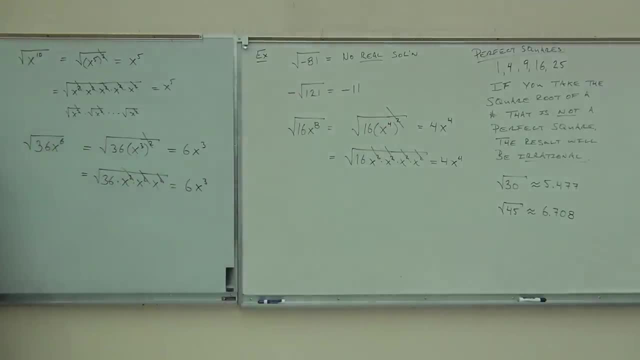 However, there are other roots besides square roots, and we're going to talk about those for a while. today, Specifically, we're going to talk about cube roots and then move on from there. First, let me tell you what a cube root even looks like. 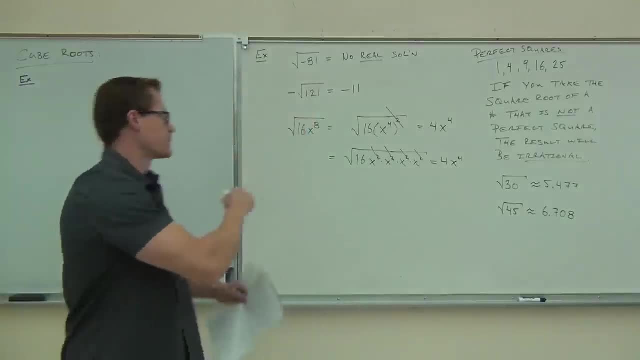 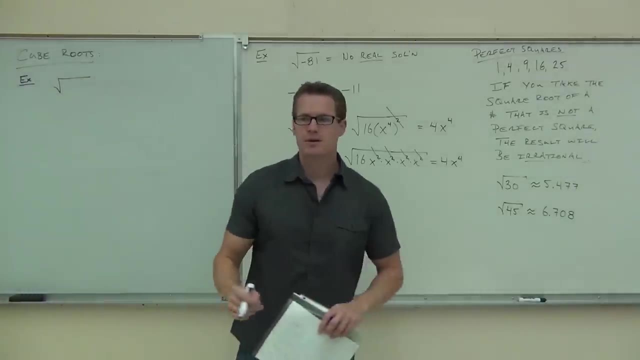 All your roots are going to have a radical. That's that shape like this, That's that shape like that. Every root you ever see is going to have that. However, there's a little space for a number right here in the index portion of our root. 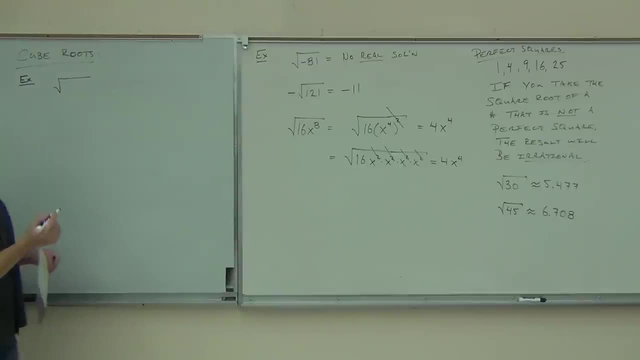 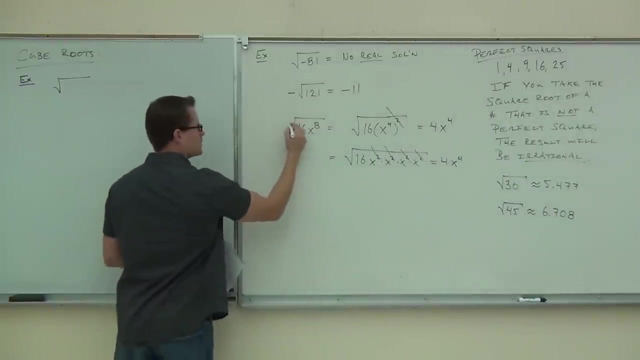 where a number should go. Now, typically we have a square root, We don't write the number, but you need to know that what's implied here is that when we have a square root, there really is a little number. here It's a 2.. 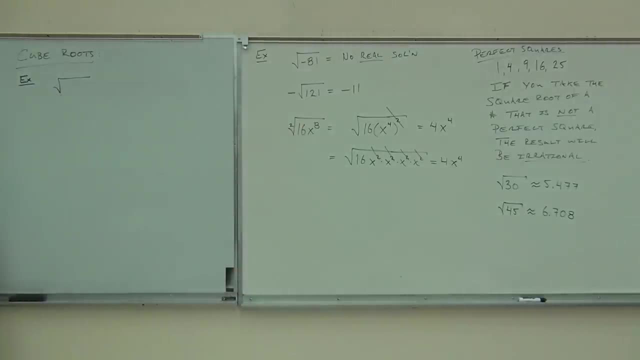 We just don't write the 2. That 2 says we have a square root and it says what we're going to do is, every time we see a square, the inverse operation. lets us simplify that. So: square root and square inverse. 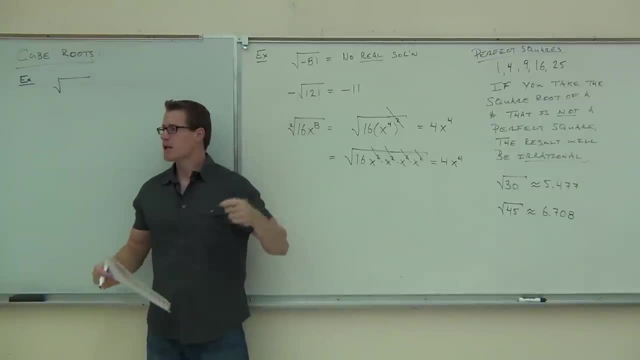 That little 2, we never write it, We never see it, It's just implied. like You know how x is actually 1x. Do you ever write the 1? x to the first power is x to the first, like that. 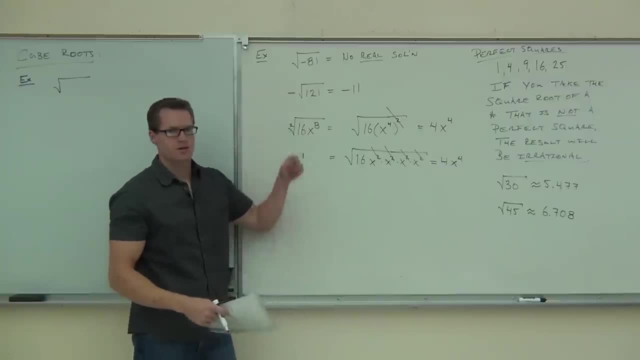 but we never write the 1.. We never write the 2 here either. It's just implied that you know that. Does that make sense? So that is That right. there is a square root, because I don't have a number, right there. 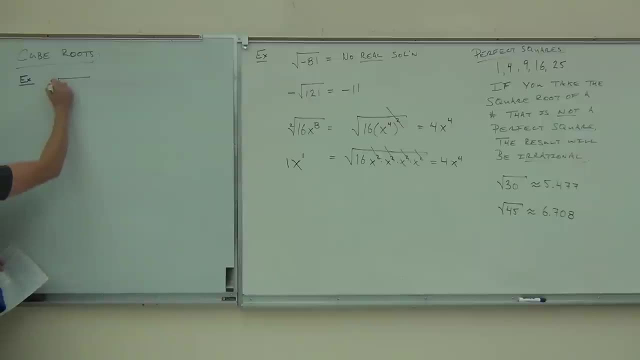 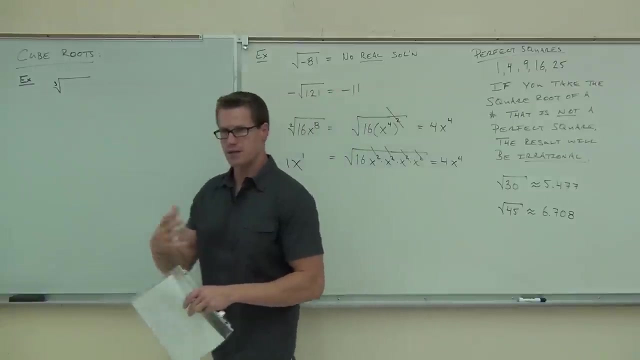 It's implied that that's a 2. If I want to show a different type of root, I just have to put a different number there. So if I put a third, a third root or a cube root, same thing. 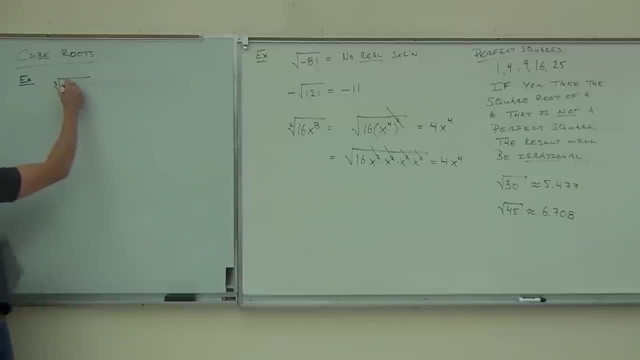 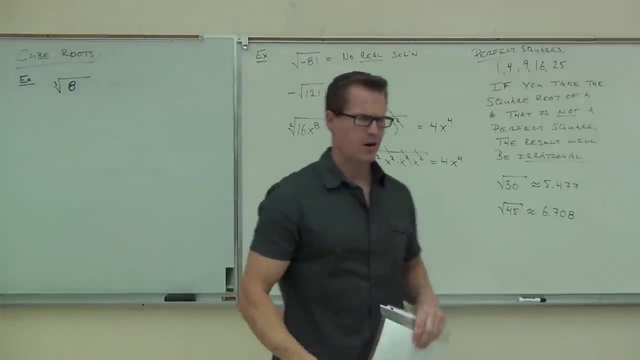 What does that mean? Let's say the cube root of. I want you to think of it. Don't say it out loud, Just think of it. Think of what a third root would mean. A square root means a number times itself gives you the radicand. 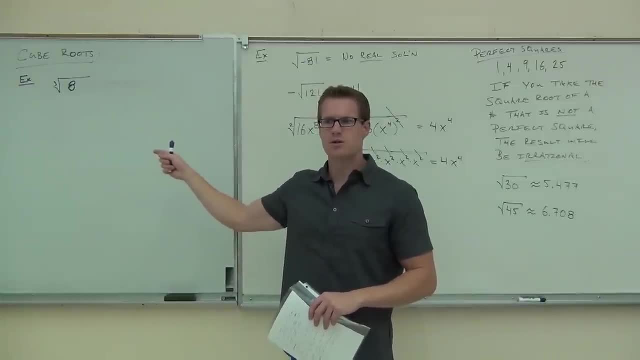 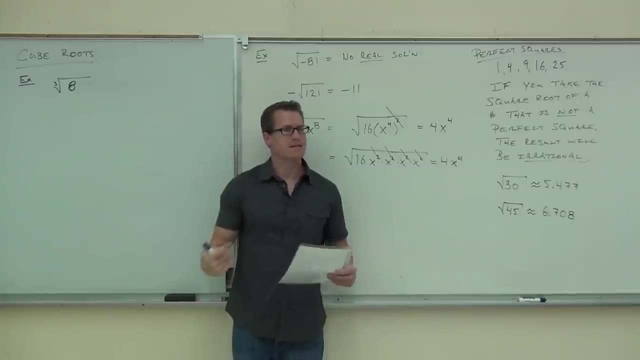 What is our radicand here? No, what is our radicand 8.. The number inside the radical is called the radicand. The radicand here is 8 for sure. What we're asking now is, instead, of a number times itself. 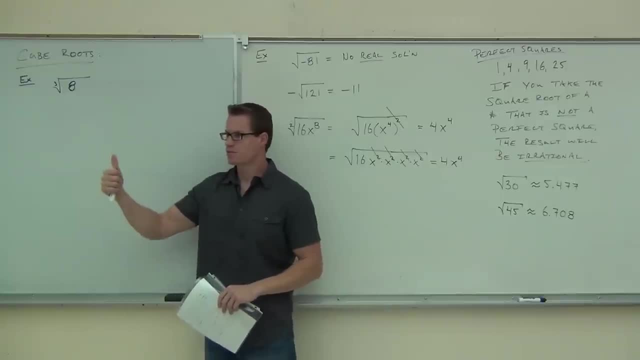 that's giving you 16, we're asking for a number times itself, times itself, So that's three times. So a number times itself twice, or a number times itself times itself, What number would give you 8? 2.. 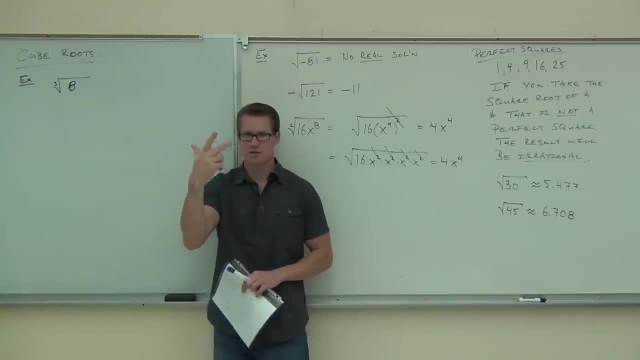 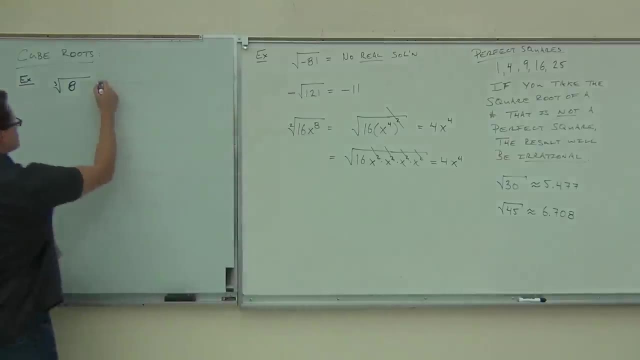 Yeah, because 2 times 2 is 4.. Times another 2 is 8.. That's what we're asking. What number? times itself three times will give you the radicand if you have a cube root. So in our case, yeah, that's equal to 2.. 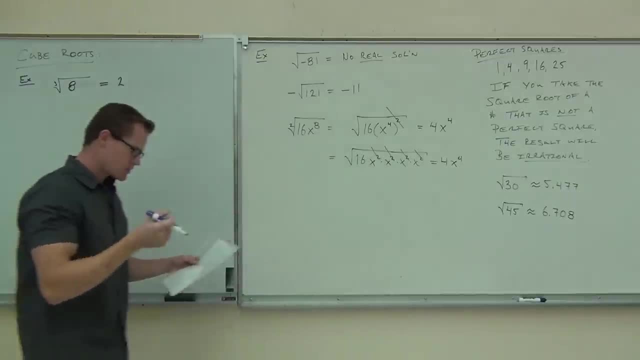 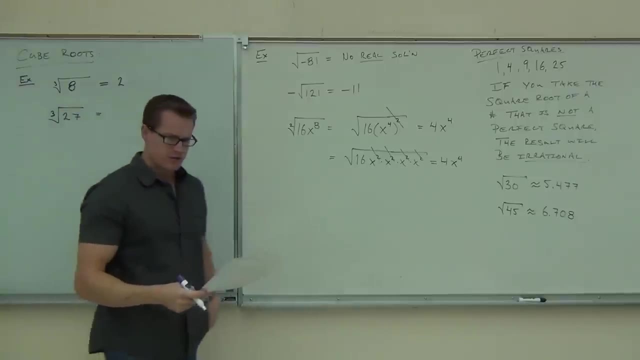 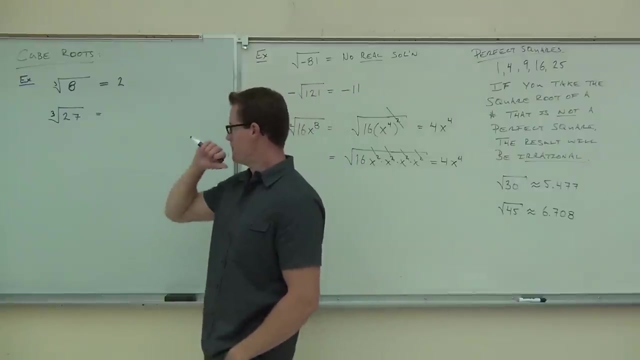 That's what the cube root means. Let's try a few more Cube root of 27,. just think about it. Just think about it. Don't say it out loud. I want you to think on these things. Cube root of 27 means it's not a square root, right? 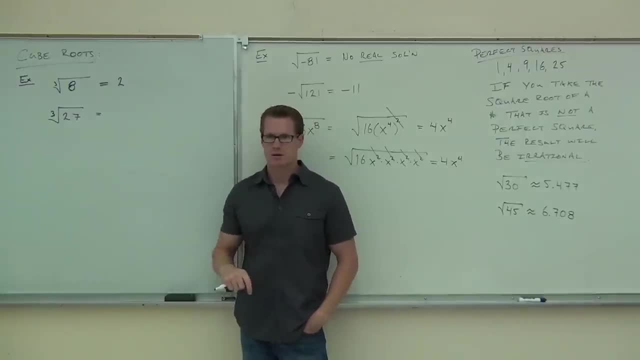 Hey, by the way, can you even take a square root of 27?? Boy, you can. on a calculator. It's not going to be a whole number, though Can you take a square root of 8 and get a whole number? 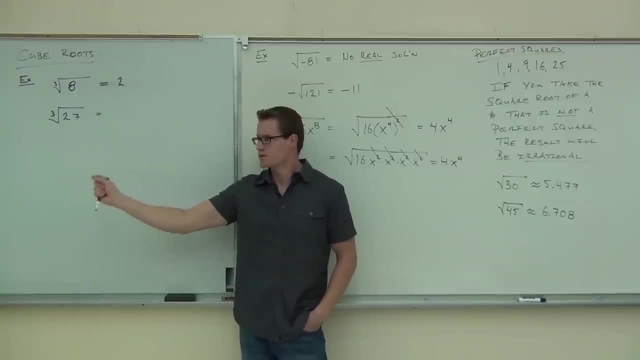 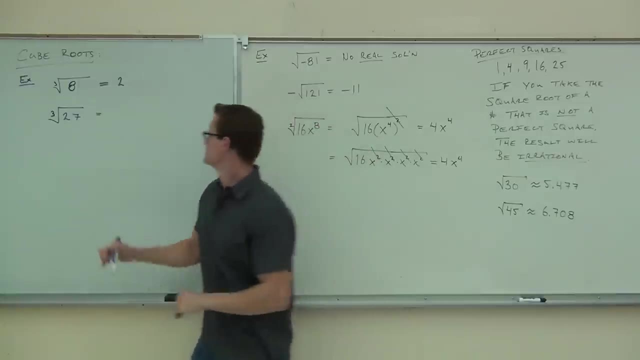 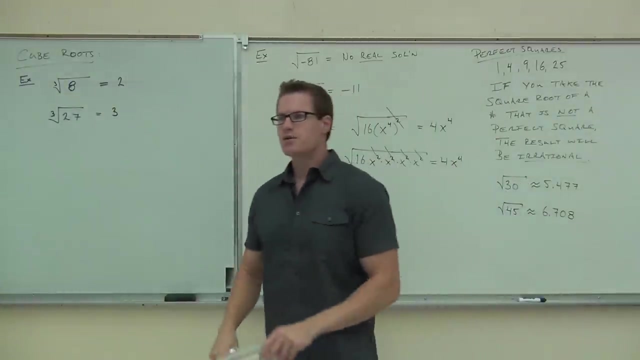 Not a square root. Cube roots are different. All right, cube roots ask one more multiplication in there. So what number times itself? What number times itself? three times will give you 27? 3. Yeah, Do you think there are more square roots that you can take a square root? 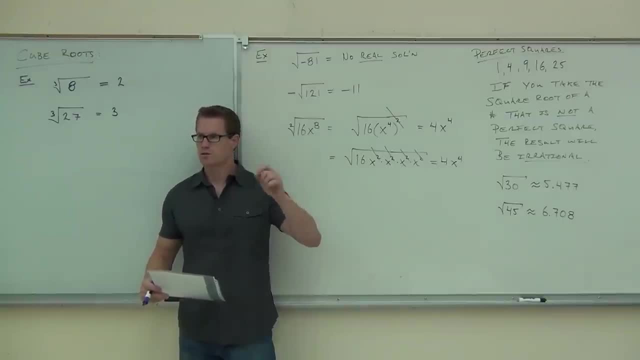 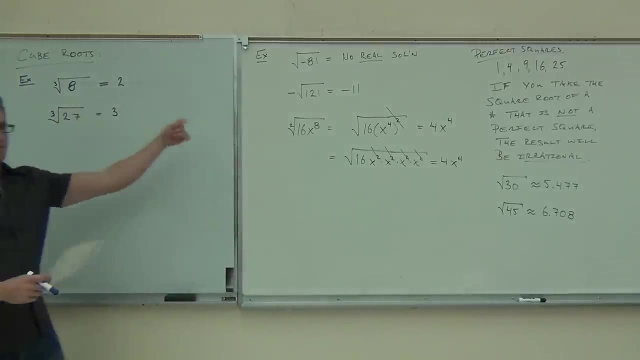 and get a whole number between 1 and 100, or more cube roots. you can take a cube root of and get a whole number between 1 and 100?. Square root of 2.. Look at this: The first square root I can take and get a whole number is 4, right. 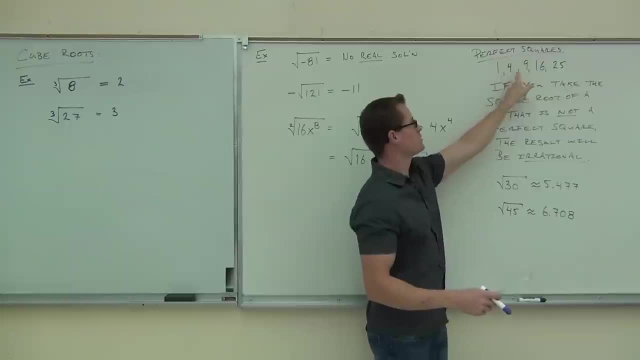 I can take a square root of this number and that number and that number You're thinking in your head: 2, 3,, 4, 5, aren't you? The first number I can take a cube root of besides 1 is 8.. 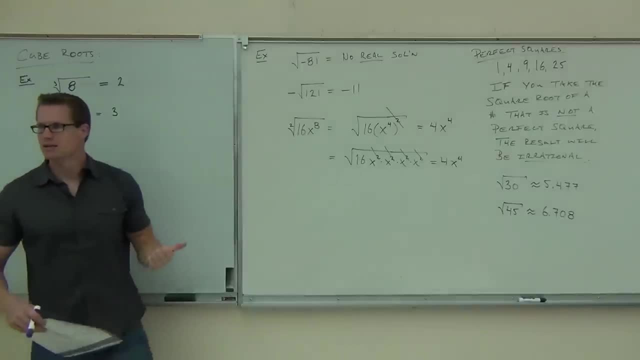 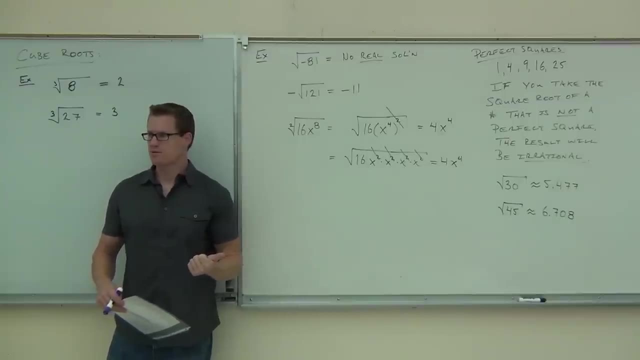 The next number: can you take a cube root of 9?? Cube root of 9.. Square root: yes, Cube root: No. How about 10?? 11,, 12,, 13,, 14,, 15,, 16,, 17,, 18,, 19,, 20.. 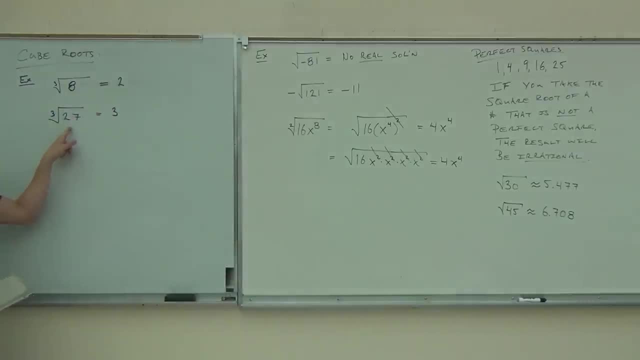 No, The next one is: look at that. The next one is 27.. That's the next number I can take, Because, look at that, that's 2, that's 3, right, There's no whole number between 2 and 3.. 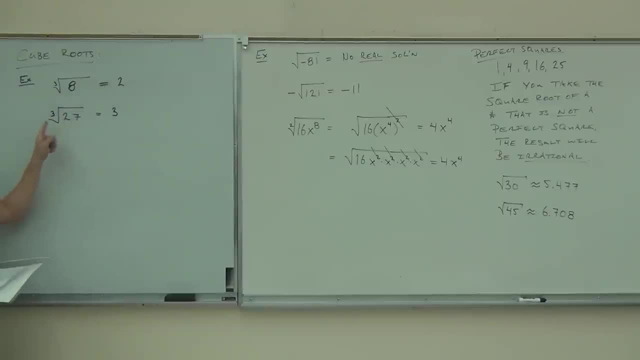 So if I can take a cube root of 8, it gives me 2.. Cube root of 27 gives me 3.. There's nothing between there I can take a cube root of and it will give me a whole number, And I don't know if that makes sense to you. 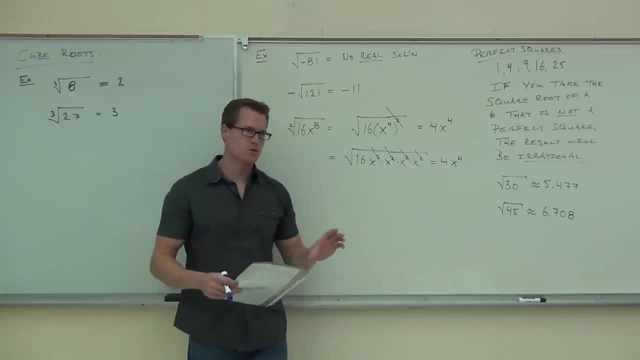 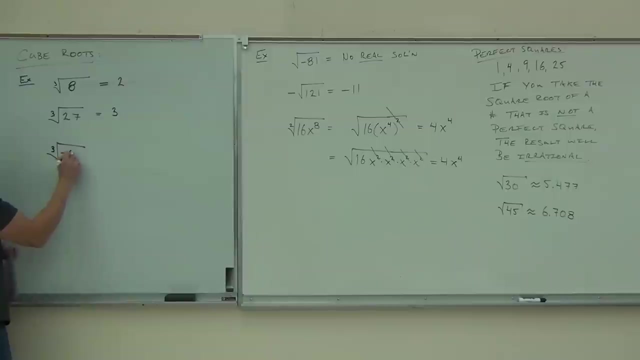 So there are going to be less perfect cubes between 1 and 100 than there are perfect squares. There's going to be less perfect fourths to the fourth power than there are perfect cubes or perfect squares. Let's do one more. Let's do the cube root of negative 64.. 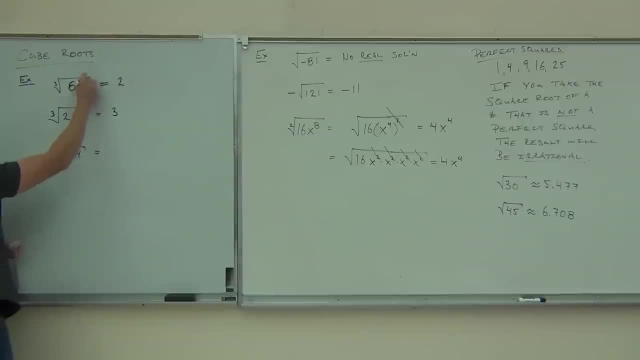 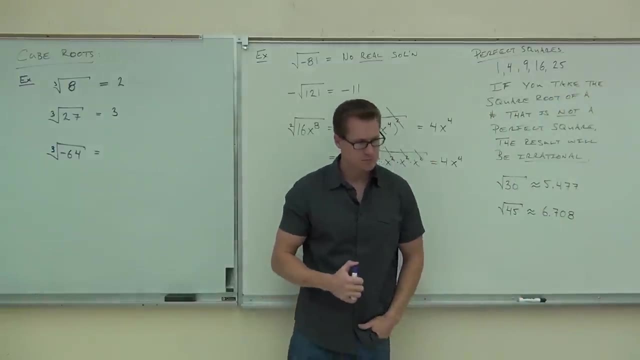 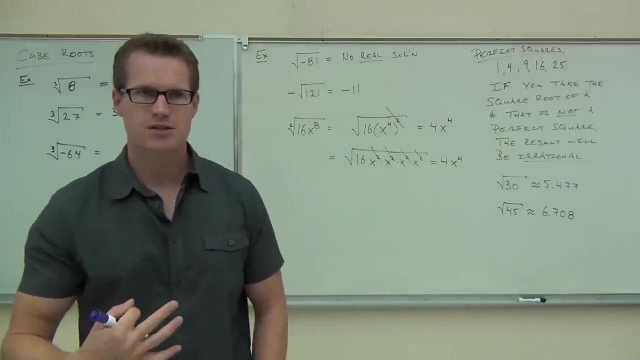 Cube root of negative 64. Let's think about that Again. I don't want you to answer out loud on these ones. I want everyone to think on this Cube root of negative 64. But this asks us: what number times itself three times gives you negative 64?? 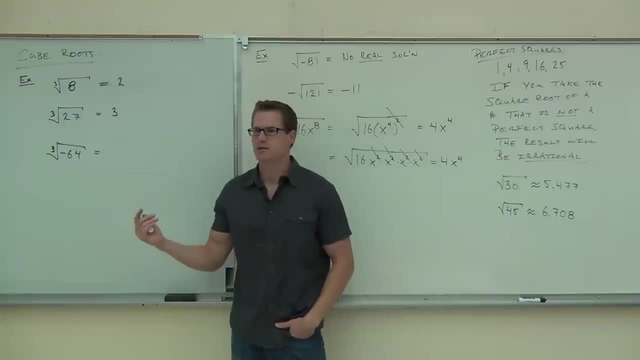 And we go: oh, there's a negative inside. No solution, right, No real solution. One of them is a negative, One of the numbers is a negative. It has to be the same number. They're all negative. Negative is positive. 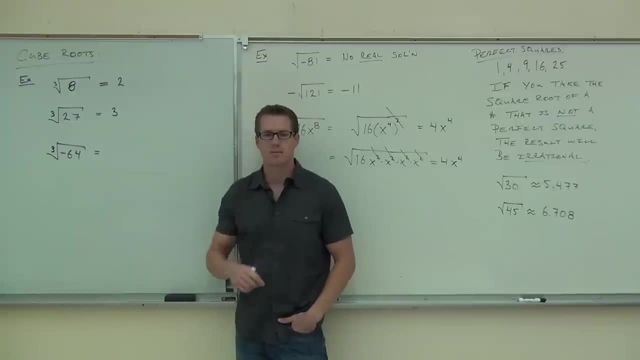 Positive times negative is negative. Say that one more time. Negative times negative is positive. Positive times negative is negative. So can we have a negative inside of a cube root? Yes, It's different than square root. A square root says a number times itself. 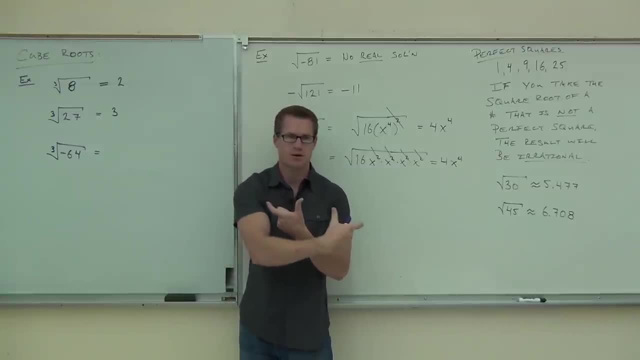 A cube root says a number times itself, times itself. Is a negative times a negative times a negative equal to a negative? Yes, Then these are possible. There's nothing you can't take a cube root of. It's different than a square root. 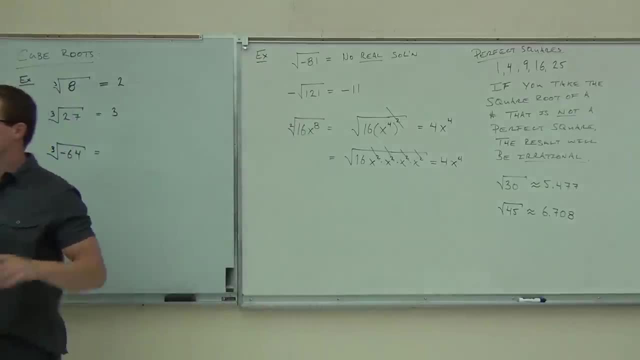 So are negatives possible? Are negatives possible inside of a cube root? Absolutely. What is this value? What times itself three times gives you negative 64? Negative 4.. Negative 4.. Yeah, it's not positive 4.. It's negative 4.. 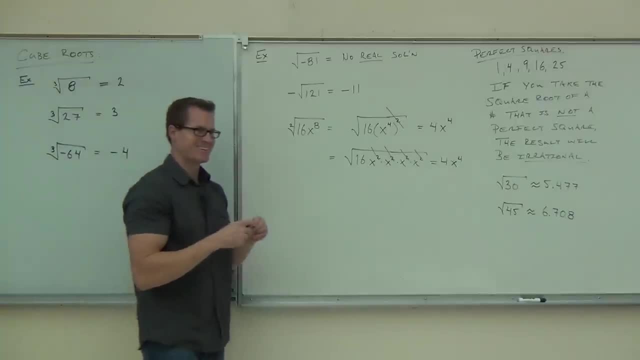 Plus you. That was an interesting one. I liked it All. right Back to math. So it's negative 4 because if you think about it, what's negative 4 times negative 4? Negative 4.. Right, So what's negative 4 times negative 4?? 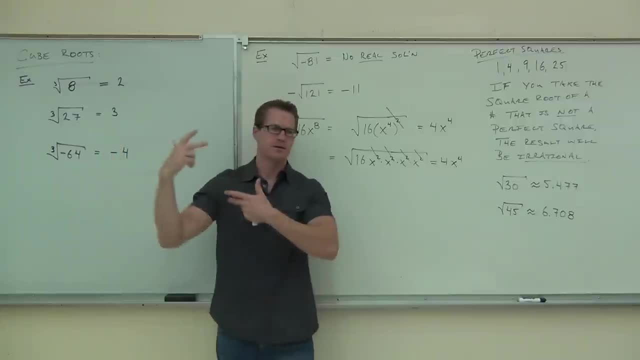 16.. Positive: 16 times negative, 4, again Negative, 16.. That's where we're getting that from. So that is possible. Is this possible? Cube root of y to the third power. Cube root of y to the third power. 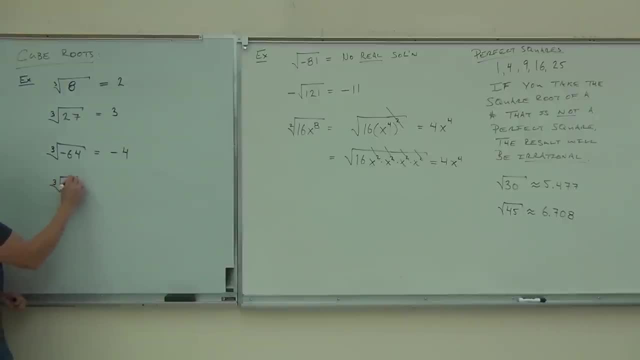 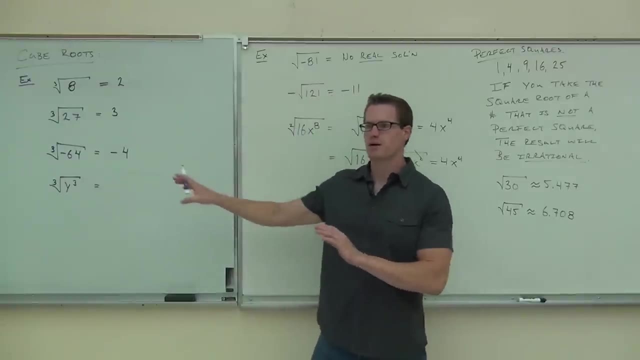 I want you to compare this to what we did over here. What we did over here is: every time we saw- please watch up here for a second- every time we saw a square root of x squared, we understood that the square root of x squared is a square. 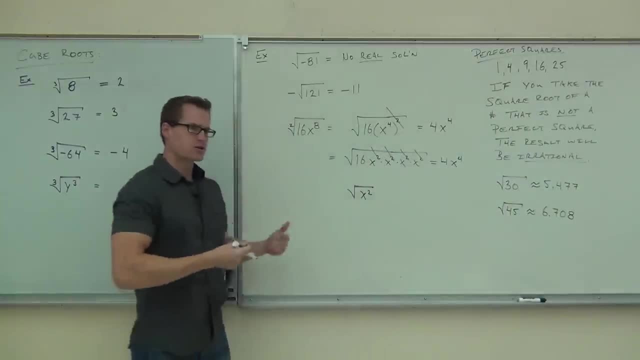 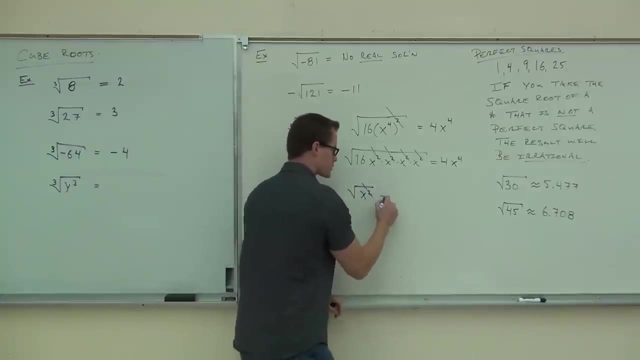 root of x squared. We understood that the square root and the square, those things are eliminating each other because they're inverse operations. and we go: oh yeah, yeah, Square root of square, that equals x. Why did that work? Look at the board here real quick. 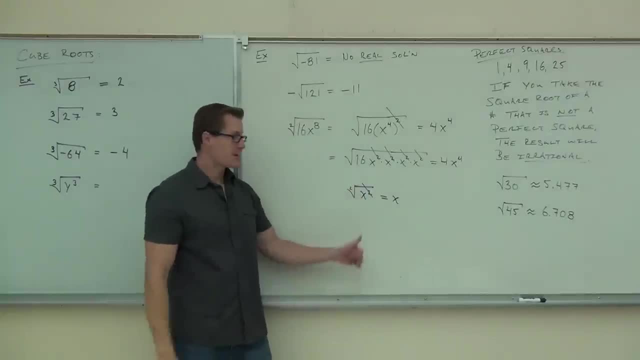 Remember there's supposed to be a little 2 here- If we match up the power with the root- say that again: if we match up the power with the root, no matter what it is, if we match up those numbers, they are inverse operations. 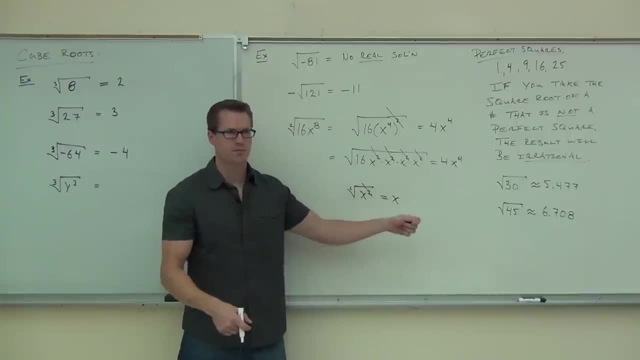 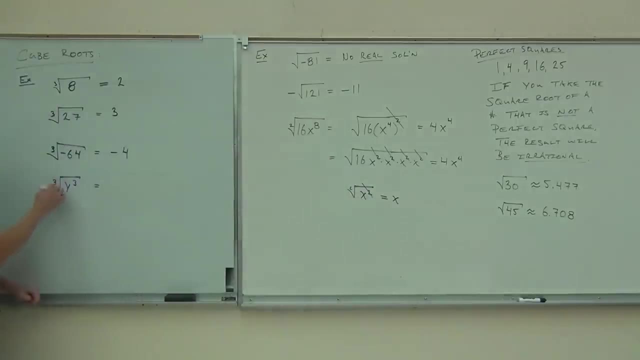 So a square undoes a square root and a square root undoes a square. A cube undoes a cube root and a cube root undoes a cube. So what is the answer on this? Y, Exactly, We've matched up the power and the root, right. 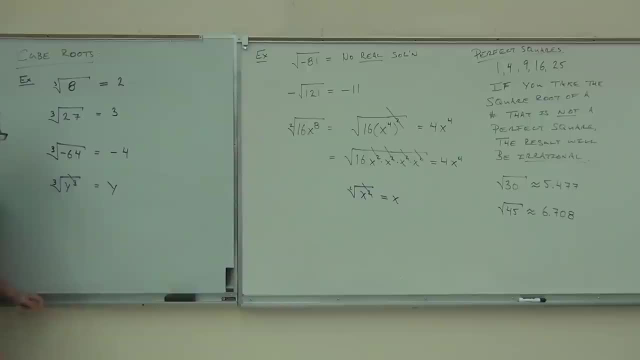 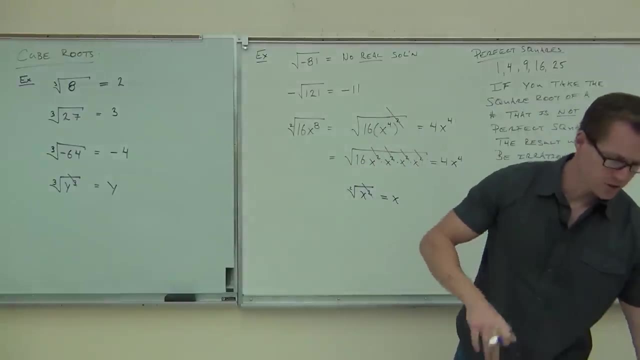 Those are inverse operations. We're going to get y. So, just like we can simplify squares inside square roots, we can simplify cubes inside cube roots. That's kind of cool And that works for every root. we're going to find out in just a little while. 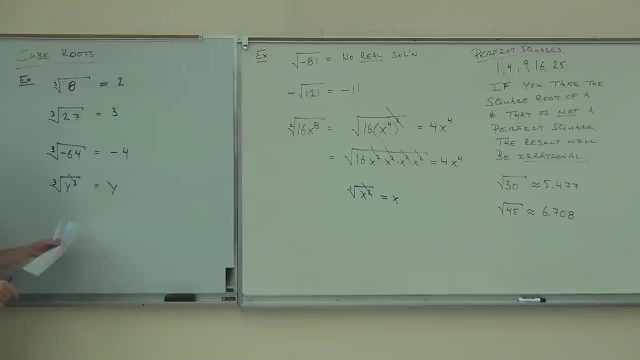 Let's try some more. We'll go through a few of these things and then I'll have you do a couple on your own. We'll talk about nth roots, And that should do it, Thank you. So then we're going to do a little bit of calculus. 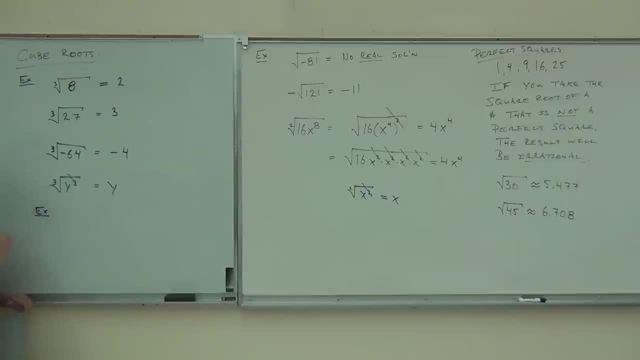 It should be about it. We might get to a little bit of graph. Cube root of zero, Zero, Yeah, zero times, zero times, zero, and that gives you zero. How about the cube root of negative? That's how many I can pick from. 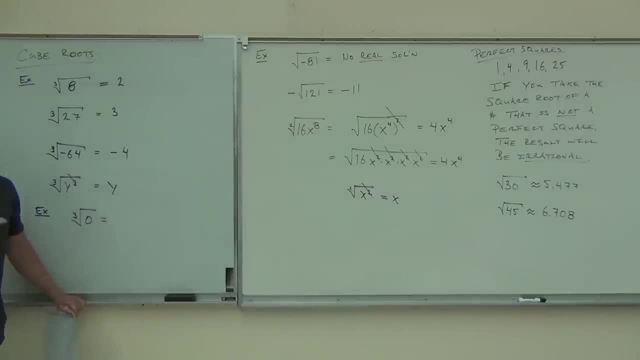 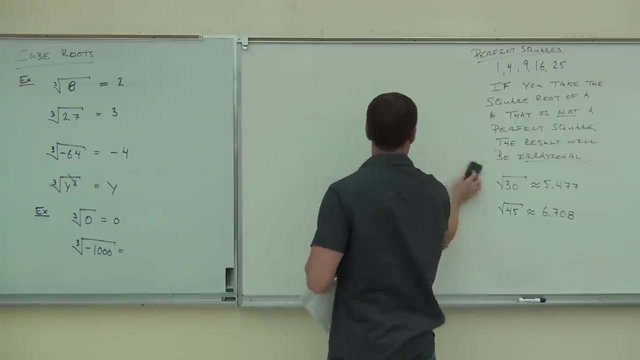 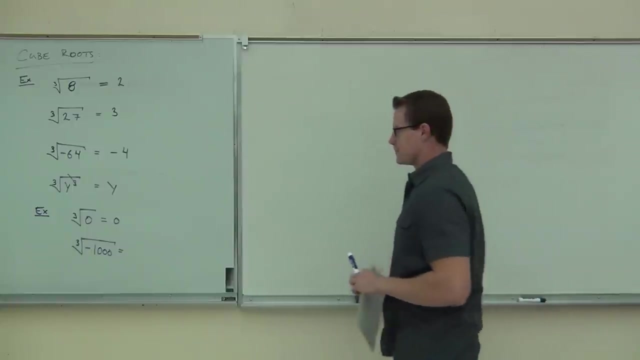 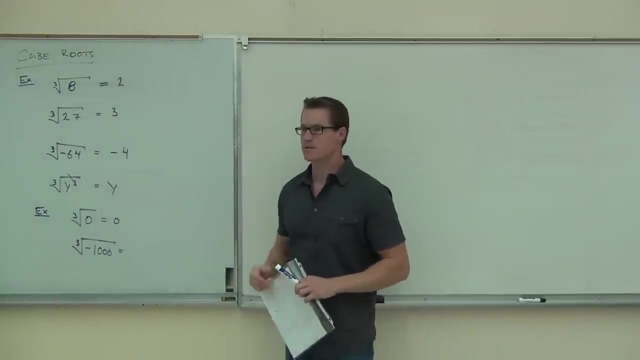 Let's see if you're really good at this. Just think of it: 1,000.. Don't say it out loud. Get rid of negative 1,000.. What times? what times? what itself gives you 1,000, or, in this case, negative 1,000? Negative 10.. Very good, Notice how a cube 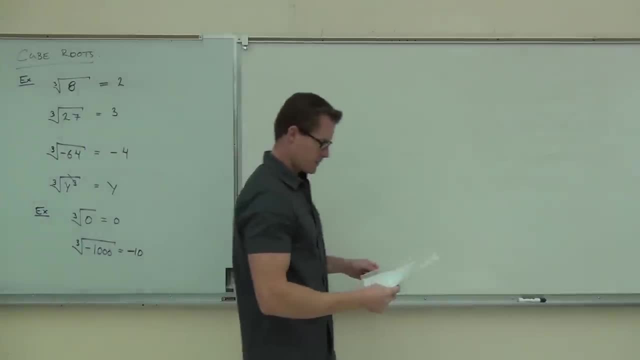 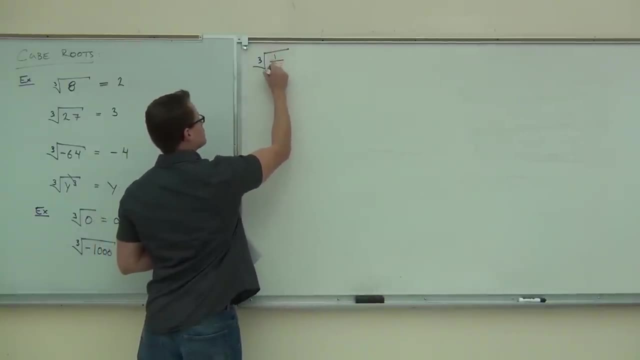 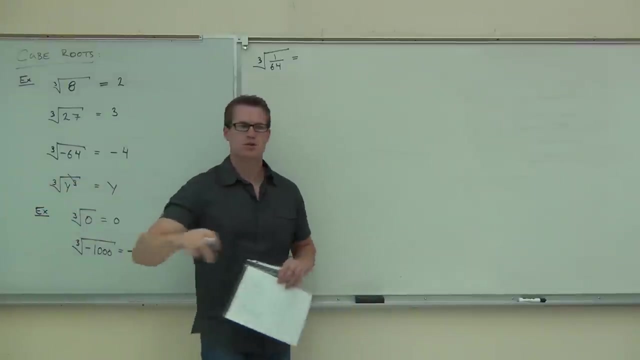 root of negative 1,000 is only up to negative 10. at this point It's kind of cool. Can you do fractions? Cube root of 1 over 64, that means we're taking the cube root of the numerator and the cube root of the denominator. What's the cube root of the numerator? 1. Cube root. 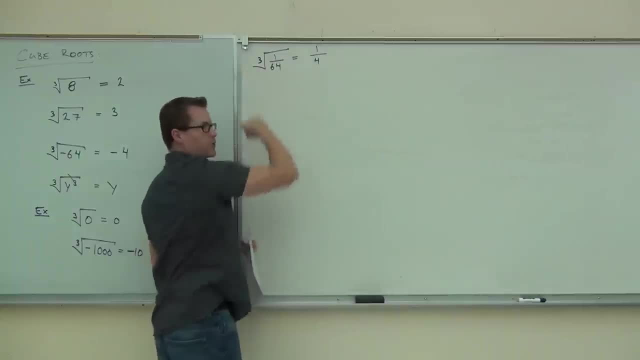 of the denominator 1.. Cool, So this is actually equal to 1. fourth Interesting right Looks a lot bigger than that. It really is Cube root of x to the ninth. We're going to do the same basic idea that we did for our square roots, only this time instead of writing this: 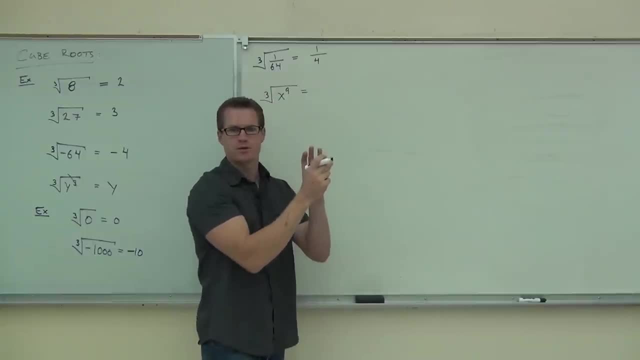 as something to the second power. I'm going to write this as something to what power? folks? I'm going to try to match up the power with the root. So again, there's two options. I'm going to show you both options until we get down to the section where this is applicable. 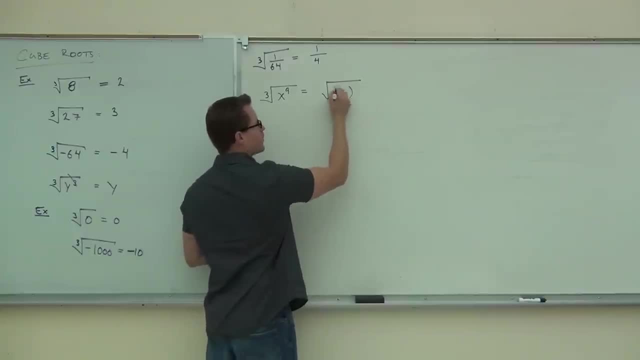 One way that you do this is write this as x to some power. Don't forget that little 3 there, by the way. You cannot forget that, Otherwise it changes the cube root into a square root, and we can't have that happen. We're going to want to write this as x to. 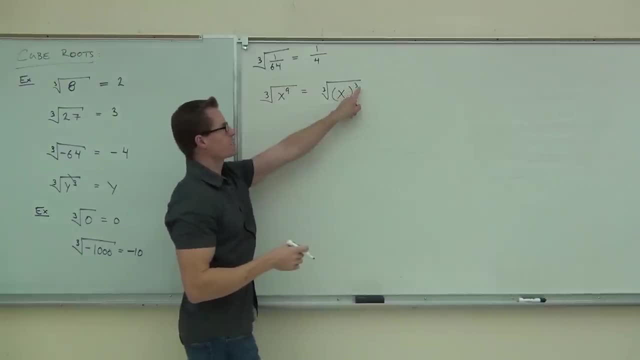 some power to the third. The reason why we're choosing third: we're trying to match up the power with the root, because we know those are inverse operations. What needs to go in there in order to keep that as x to the ninth power? 3.. Good because 3.. 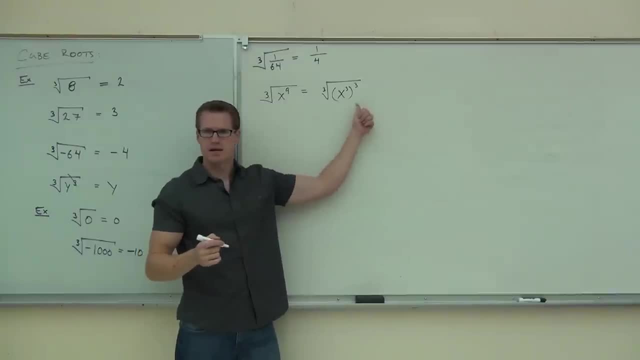 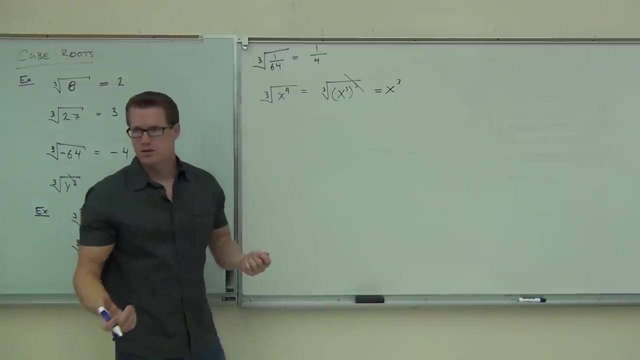 To the third power. we multiply those In your head. is it still okay that that is x to the ninth? I bet you're okay with that. That's still x to the ninth. We multiply that. Look at power root, just like with the squares. that simplifies The other way you could do. 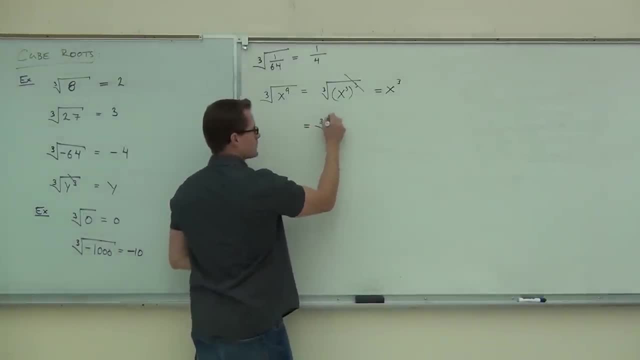 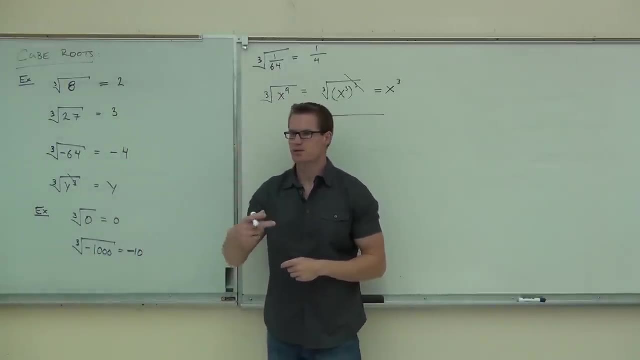 this. check this out. You could have a cube root. x to the ninth is the same thing as now. I'm not going to write this as x squared times, x squared times, x squared. Notice: if I multiply x squared times x squared does a square cancel with a cube root. No, a cube. 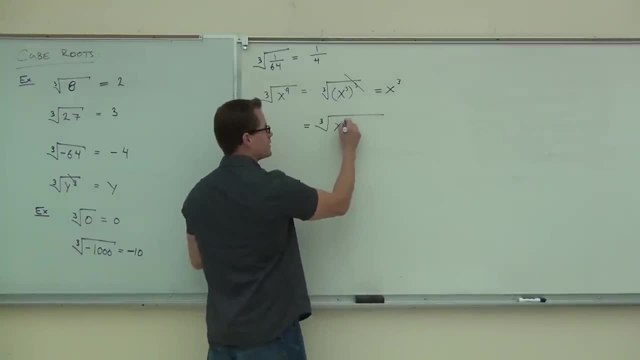 cancels with a cube root. I'm going to write this as as many powers of x to the three as I can: x to the third, x to the third. that's x to the. let's see 3,, 6,. here's 9.. That's. 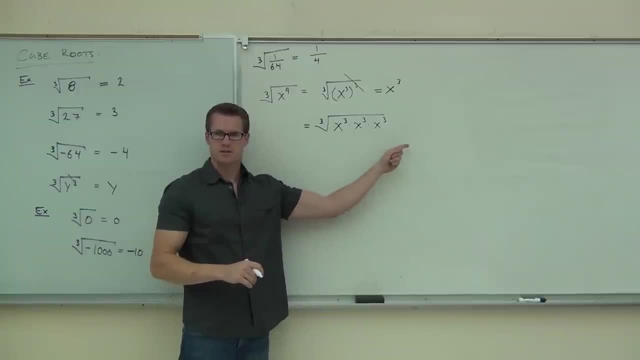 still x to the ninth. It's still x to the ninth. Yes, no, Every time you see a cube root and a third power, those things are inverse operations again, because I can split those roots up, So I'm going to write this as the cube root of x to the third times. a cube root of x to 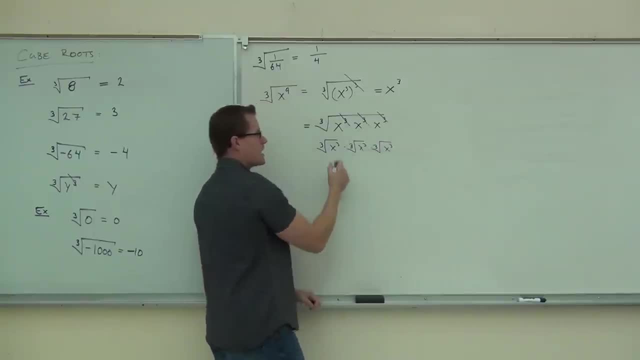 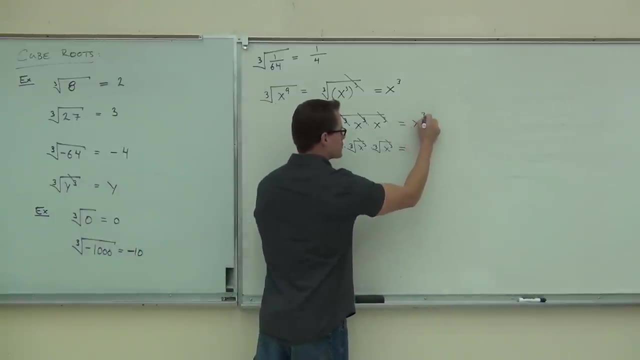 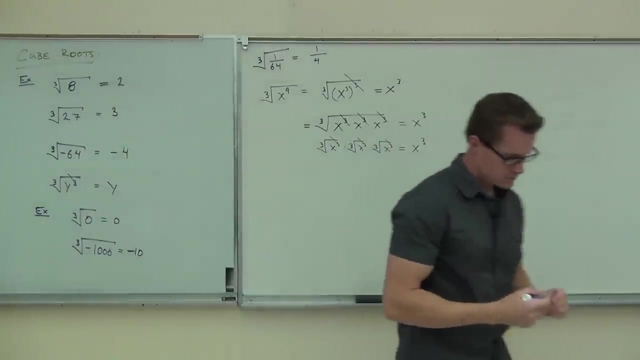 the third times a cube root of x to the third. Every one of those matches up just like that example right there And we would get in either case x to the third. So again, there's two ways we can do that. You okay with that one? 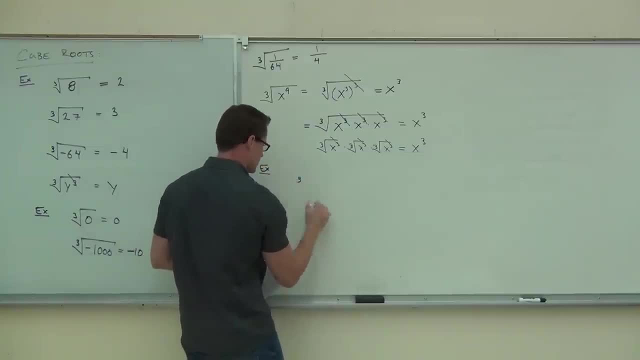 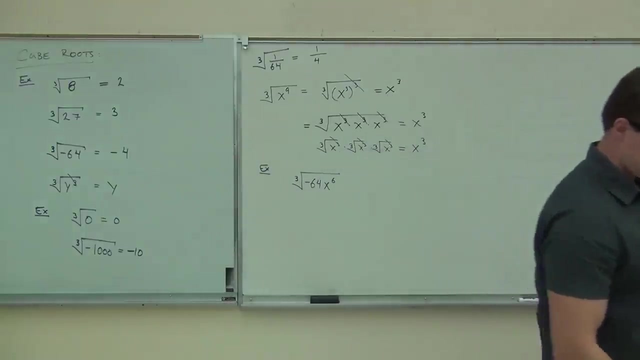 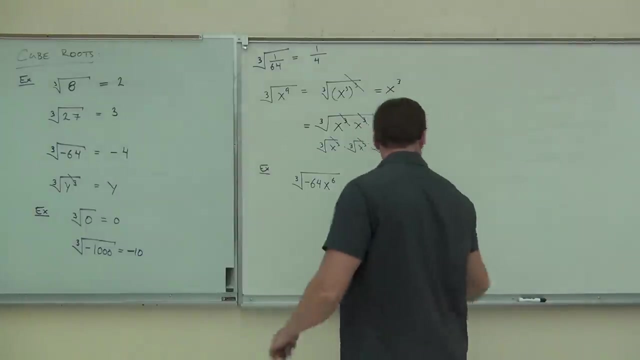 Okay, 좌 Exec. So cube root of negative 64x to the sixth: even though it's negative, it's a cube root. So we can't take the cube root of that Right Z fuck for the wholeArgo. 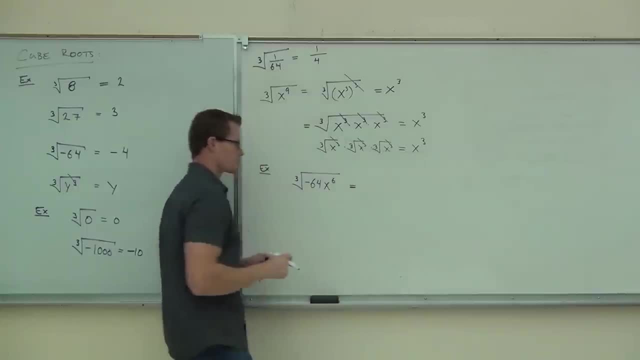 thing to do in square. So if you compute x And therefore have six p Between Z, Bye bye. Let's show both ways here again. First the way you'd write this: can you take the cube root of negative 64?? 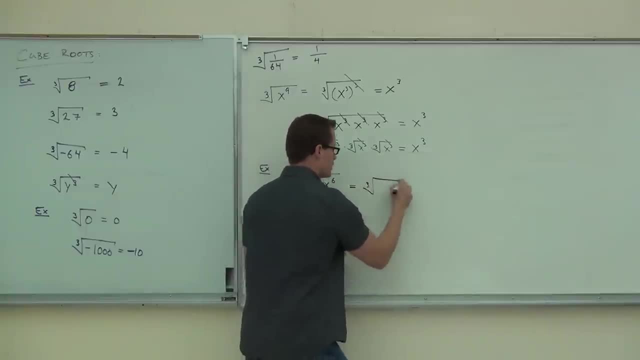 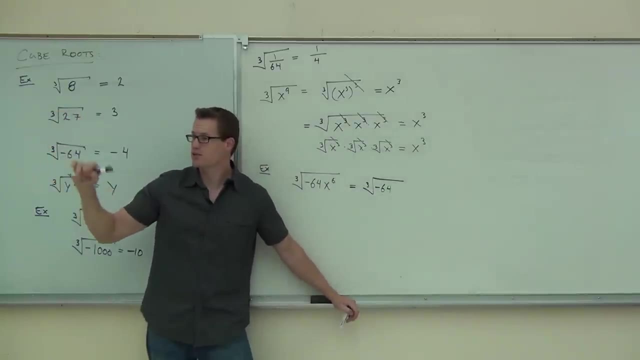 Yeah, Sure, So we're going to leave that alone for now. Negative 64.. However, I do need to write this variable as something different. Give me the first option in writing that variable. How can I write x to the sixth so that I can simplify it with a cube root? 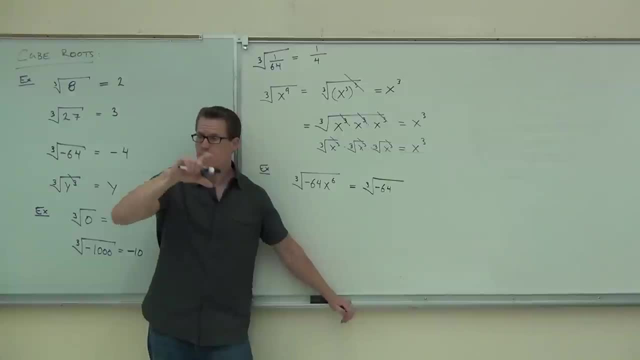 X squared times. cube root: X squared first or x cubed, X squared. You have two options, right. One of them is for a square root and one of them is for a cube root. You're either going to write this as x to the second, to the third or x to the third. 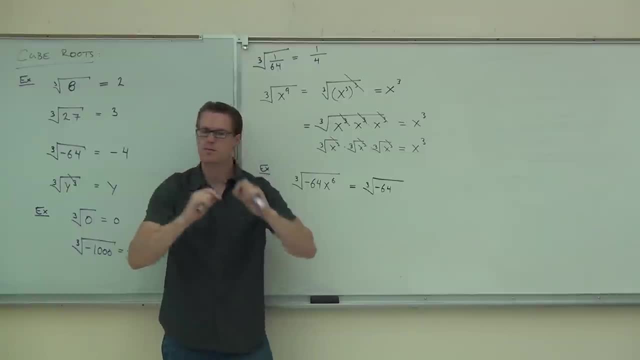 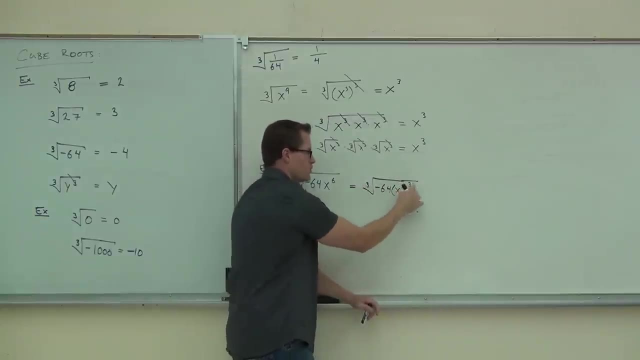 to the second. Which one's going to work here? X to the second to the third, Perfect. X to the second to the third. Why? Because we're trying to match up the cube with a cube root. That's what we're doing. 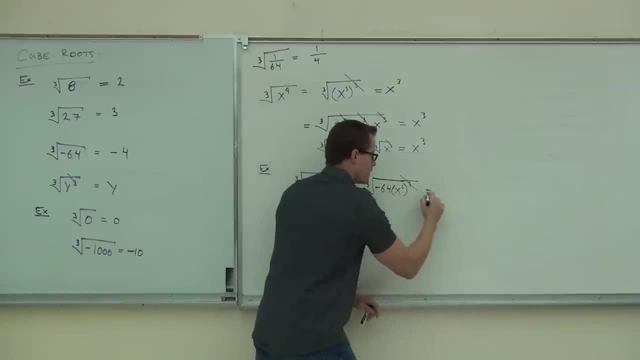 Notice how this power has to match that in order to simplify Cube root of negative 64, we already know that's negative 4.. Cube root of x squared to the third, that third and the cube root they'll simplify out and we get x squared. 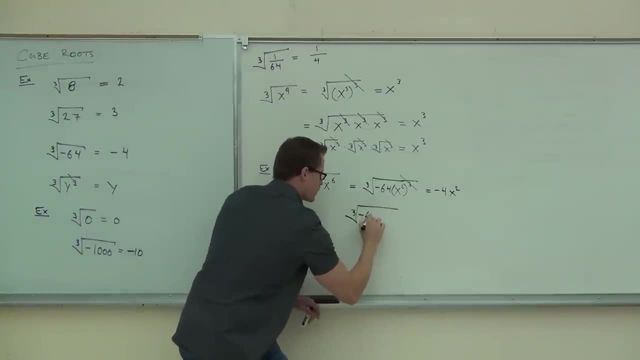 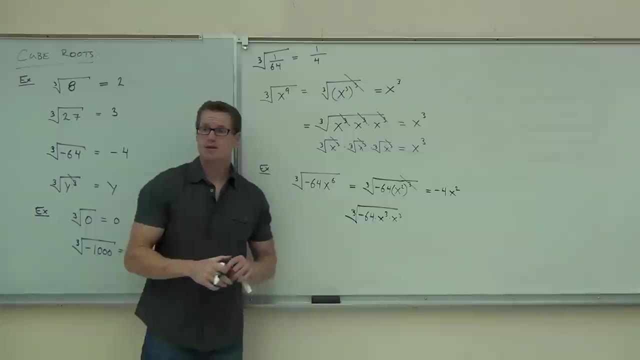 The other way that you could do this: negative 64, and you could write this instead as x to the third times, x to the third. Do you see that those x to the thirds are going to simplify? Yes, Which way do you like better? 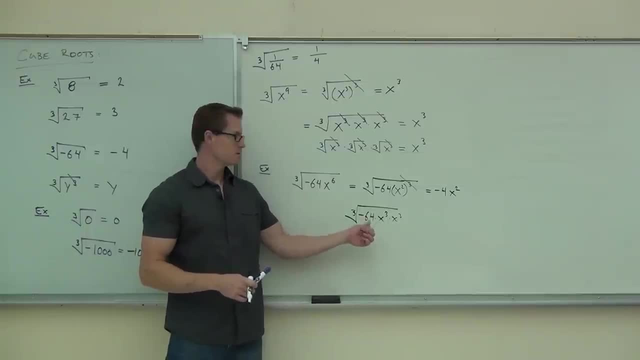 The first way or the second way? Which do you think? The second way Like the second way. First way. First way works great for even. It doesn't work so good for odd. You can't do that, So hopefully you get comfortable. 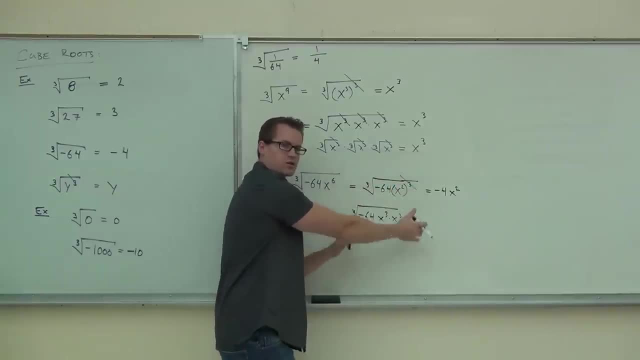 If you're comfortable with this one, great. I need you to be comfortable with this one as well later on. In either case, those simplify out and you get x squared to the third. That's the other way that you could do this. 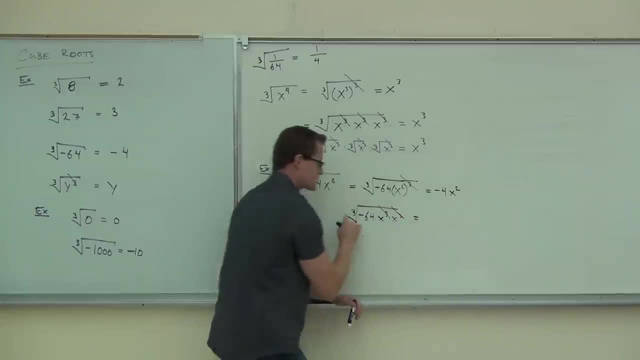 Negative 64.. Negative 64.. Negative 64.. I still take the cube root of negative 64.. I have two x's that I was able to simplify out of that radical Negative 4x squared is our answer. I'd like you to try a few of these on your own. 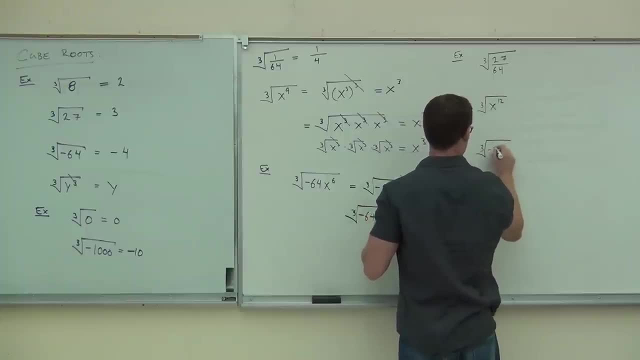 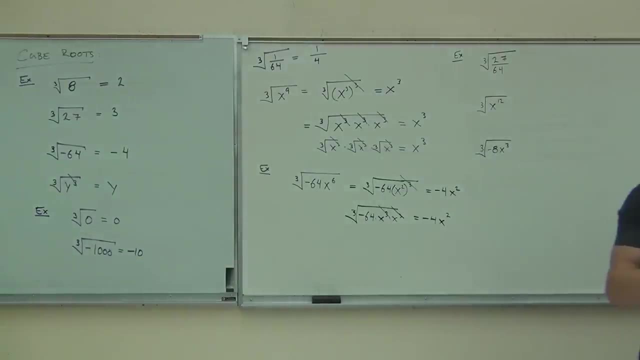 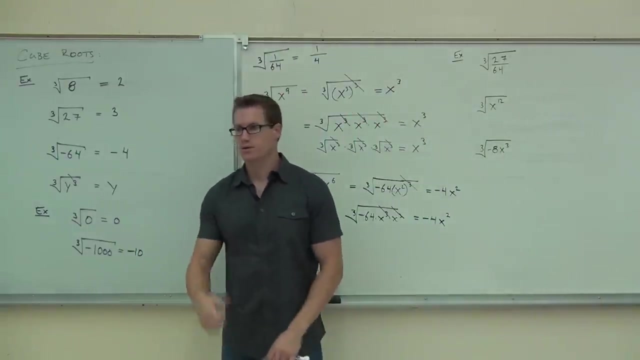 By the way, there's not a whole lot of numbers I can give you right now that you can find the cube root of, Because if you think about the first five perfect cubes, well, if there's one, then there's eight, There's 27,, 64,, 125.. 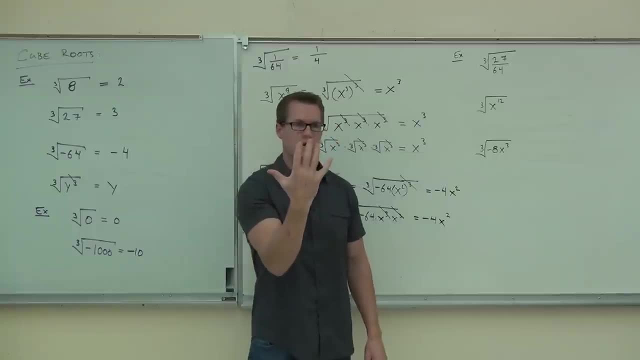 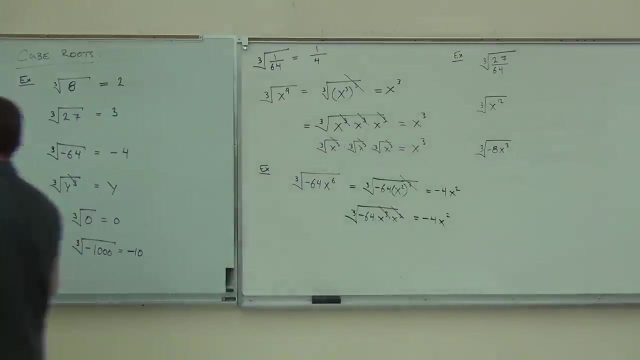 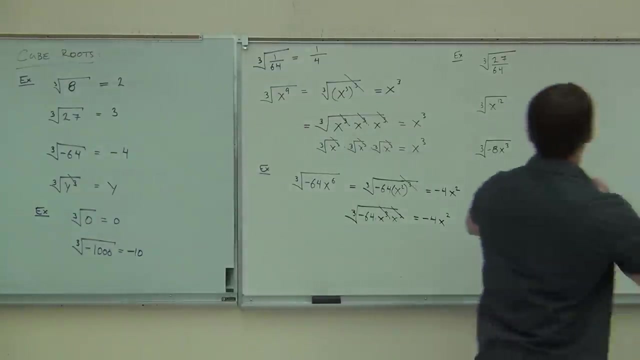 That's already. that's the first five perfect cubes. So you can only take the cube root of those five numbers that are between 1 and 200.. Two hundred, Two hundred. Okay. so first example: we have cube root of 27 over 64, we're going to take the cube. 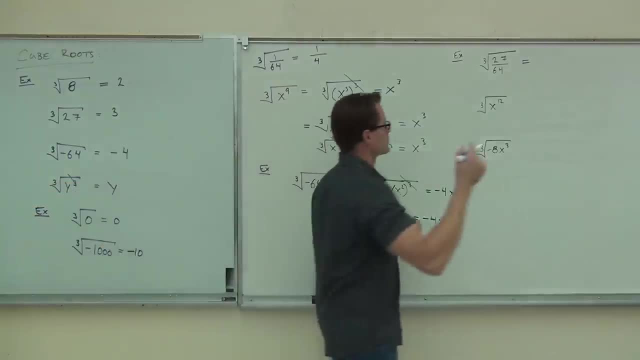 root of the numerator and the denominator cube root of 27 is: these are going to be very familiar numbers after a while because again, there's only five of them. I can have you do 1,, 8,, 27,, 64, and 125, that's it, and if it's not one of those numbers, you 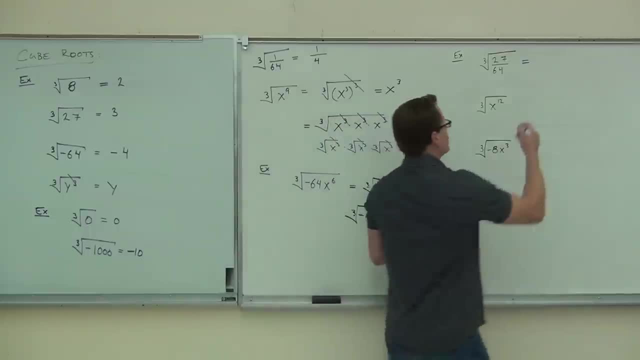 can't take the cube root of it and get a whole number out of it. So here we go. yeah, 3 over, it's 3, fourths for sure. cube root of x to the 12th. you're going to do this one of two ways and either way, first way you do something, you're going. 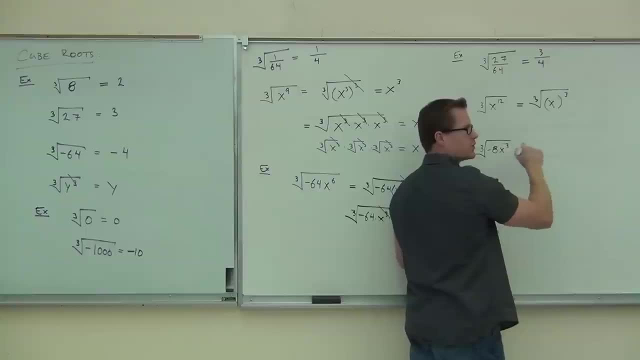 to do something to the. we want third power. we want to match up the power on the root. what number has to go there? We would get x to the 4th. if you do it the other way, you're going to get the same answer. 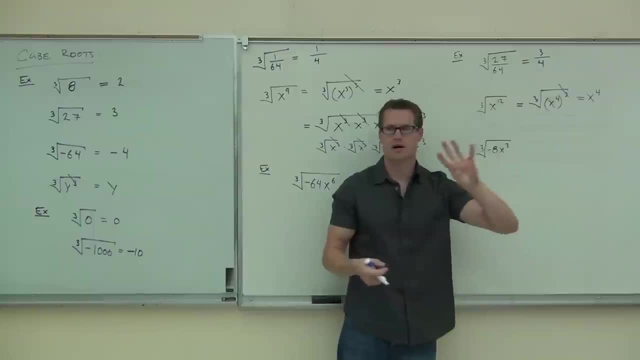 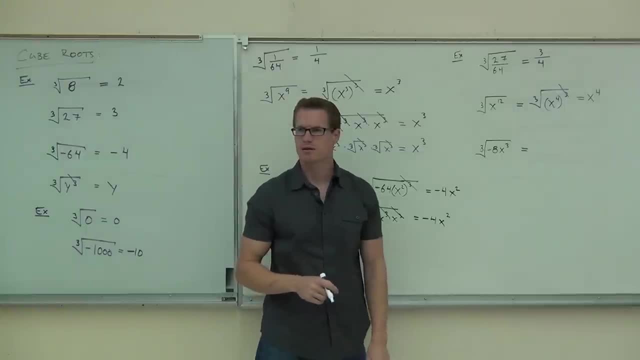 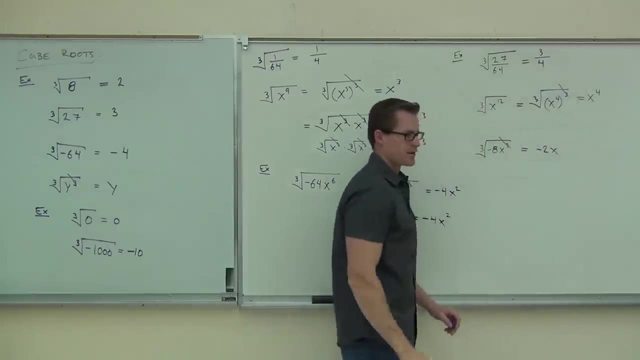 Here the cube root of negative 8,. what's the cube root of negative 8? Good. And the cube root of x to the 3rd, those simplified we get. just, Let's get some x out of that. Raise your hand if you feel okay with these cube roots. 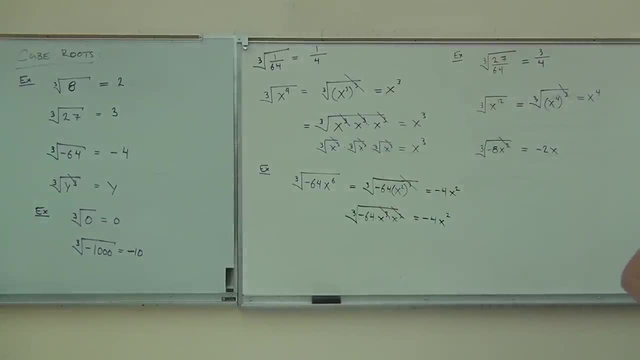 Good deal, You guys on the right-hand side. Okay, Let's move it up one more time. We're not going to talk about square roots now. we're not going to talk about cube roots now. we're talking about any root that I want. 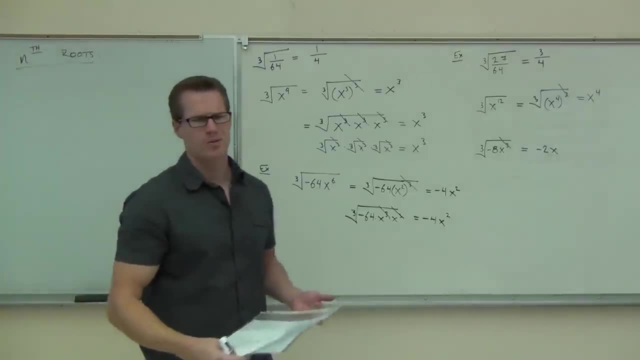 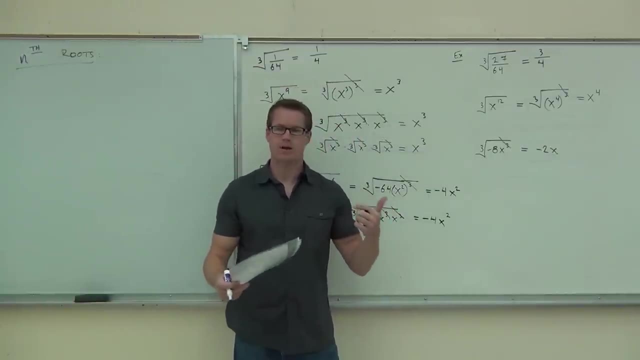 And we say any root that we want is an nth root. You know what's the n doing there N stands for any integer number or any whole number that you want: 1, oh that's right, not 1, you can't take it out. 1th root, square root, 2,, 3,, 4,, 5,, 6,, 7,, 8,, 9,, 10,, forever. 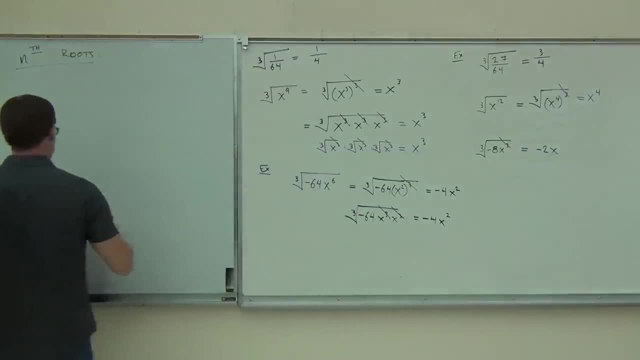 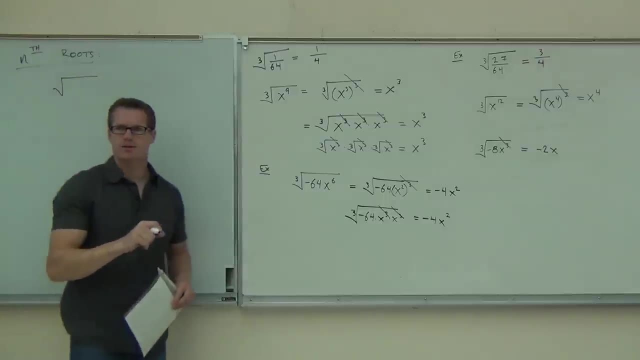 and ever number Whatever type of root that I want to talk about. Here's how every root looks. we know we have a radical and we know we put a little number up front. that index, that indices, right there is typically, if I don't write anything, what's? 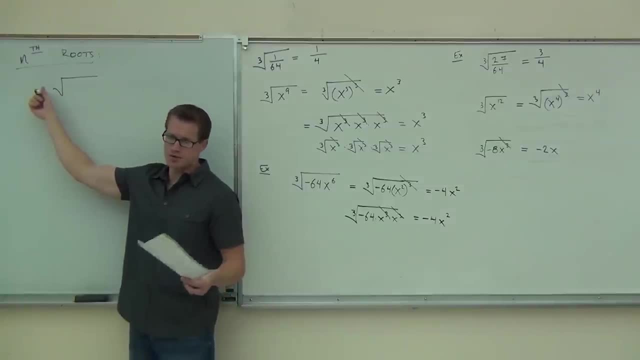 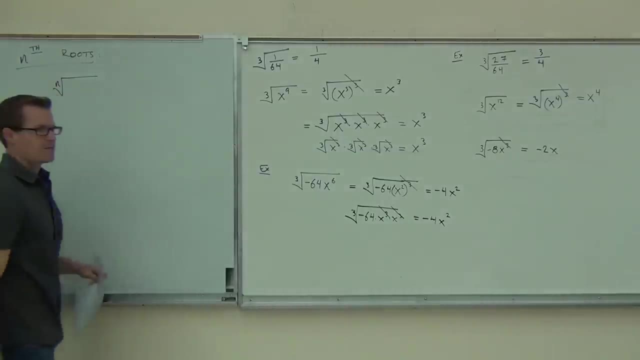 that index: 2. 2. Good, If I put a 3, it's a cube root. if I put a 4, it's a 4th root. 5, it's a 5th root. whatever number I have there, it's that type of root. that's how we're getting the nth root. 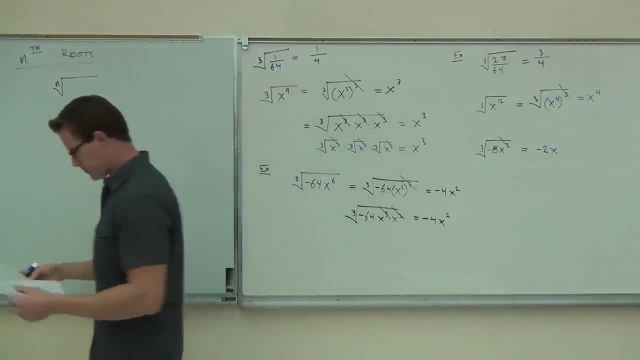 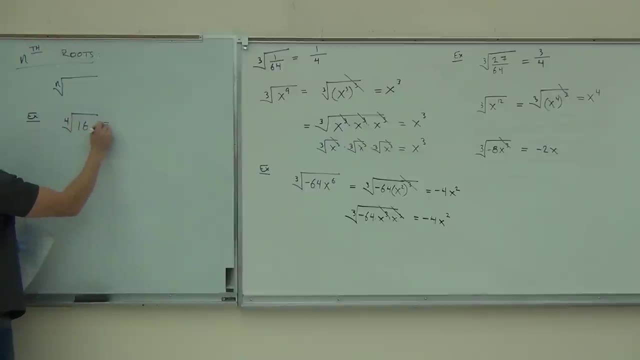 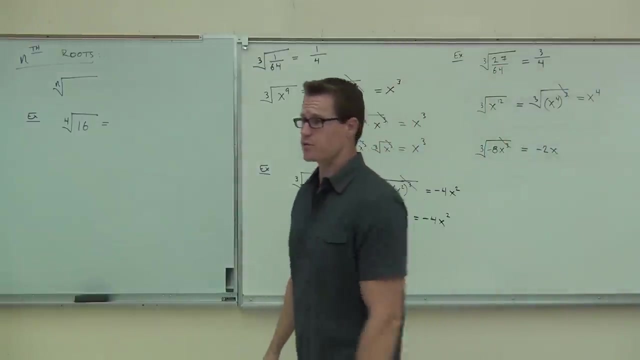 2nd root, 3rd root, 4th, 5th, 6th, that type of root, For instance, can we think about what the 4th root of 16 means? What's the 4th root of 16 mean that you're looking for? 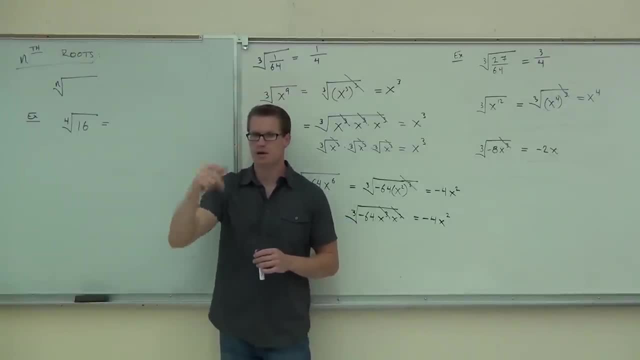 We know a square root is a number that's equal to 1.. We know a cube root is a number times itself, right? A cube root is a number times itself, times itself. What's the 4th root mean? 4 times itself. 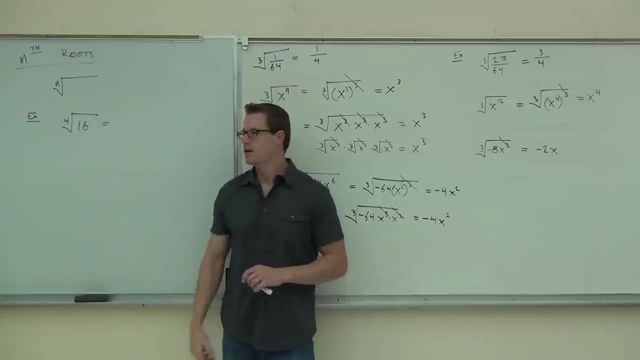 Again. yeah, that's all it means. same idea. Can you think of a number times itself? 4 times, that gives you 16? 2. 2., 2. 2. That's all. an nth root is it's whatever I give you. it's the number times itself. 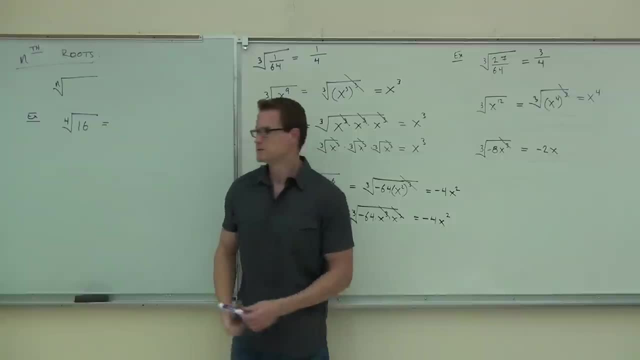 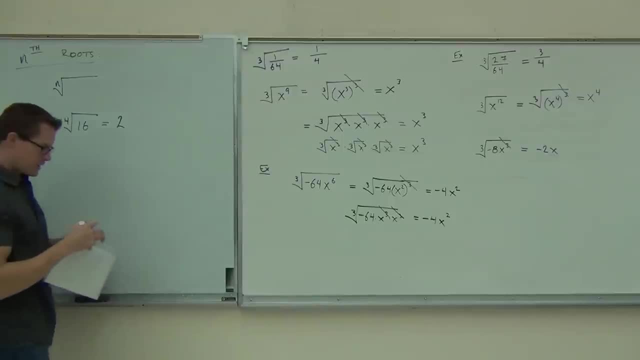 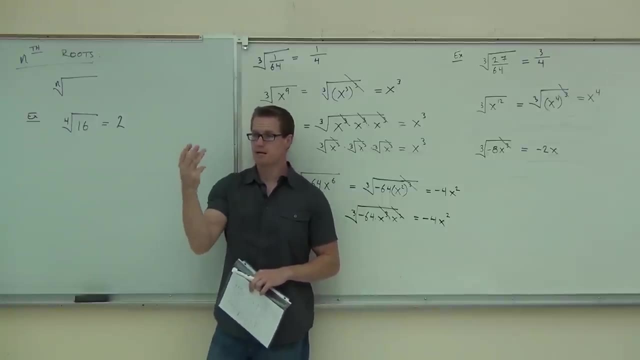 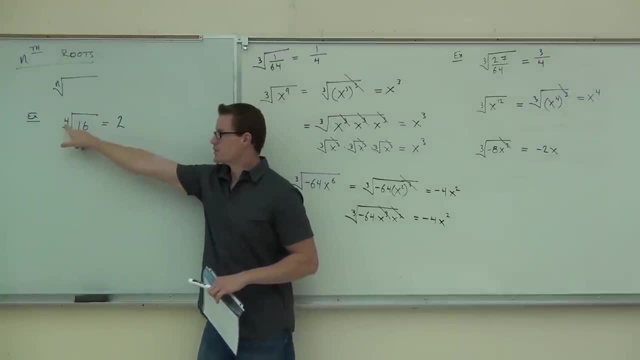 Positive? Oh no. Do you think that you're going to get any kind of negative inside of any even root? No, That's impossible. If you have an even root, that means a number times itself, an even number of times. So 2, or 4, or 6, or 8 times. if you have a negative that many times, you're going to. 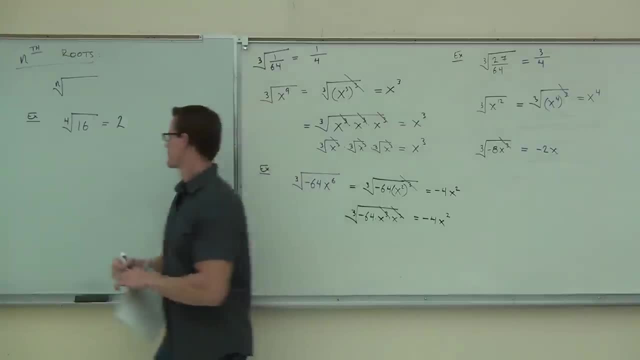 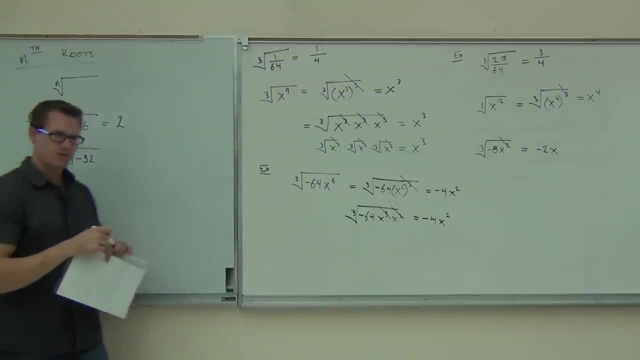 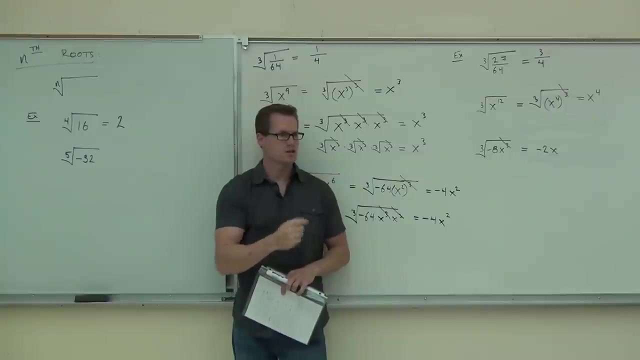 get a positive number. There's no way to get a negative number. Okay, How about inside of a 5th root? Is it okay to have a negative? inside of a 5th root? You have the extra time right. The extra time where it doesn't match up evenly, 2 by 2, is going to make your answer negative. 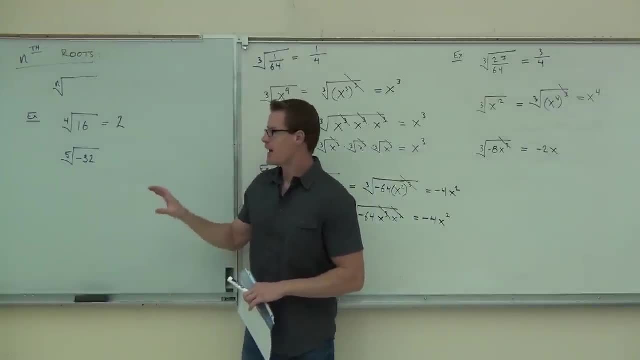 Or potentially you could get a negative inside of that root. Is it okay to have a negative inside any odd-powered root? For sure That's okay. That's okay Because you have the extra negative tacked on. that's going to change your answer to negative. 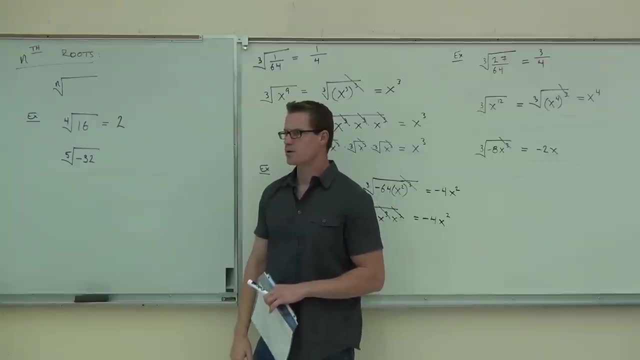 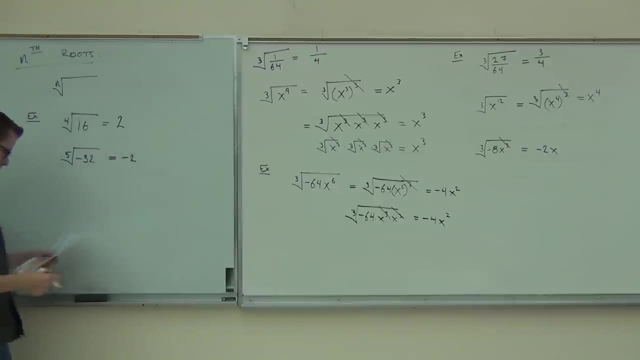 How about the 5th root of negative 32?? What do you think on that? one Good, because negative 2 times, negative 2, 5 times is going to give you negative 32.. Again, is this possible? We have a negative outside of the square root, is that okay? 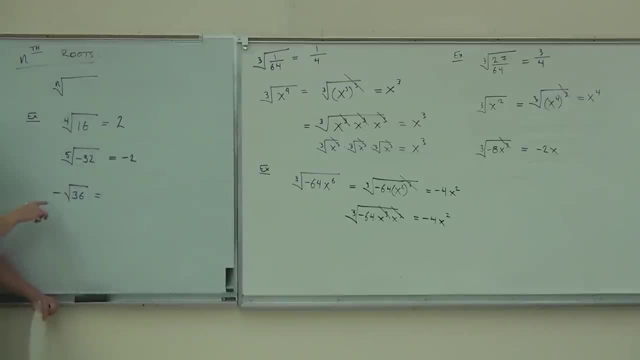 That's how much. What's our n here, by the way? What's our n? Good? okay, And that one is: Why no real solution? Yeah, it's an even root. That's right. We can't have a negative times, a negative times, a negative times, a negative, and still get a negative. 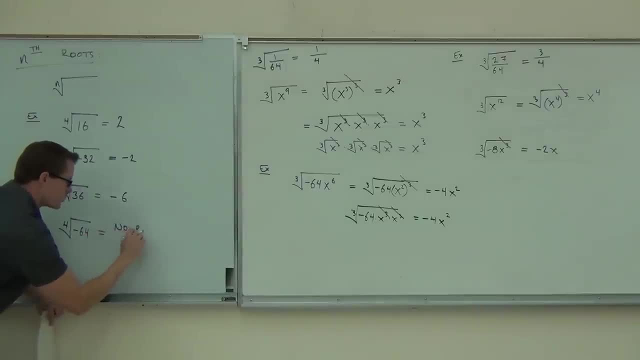 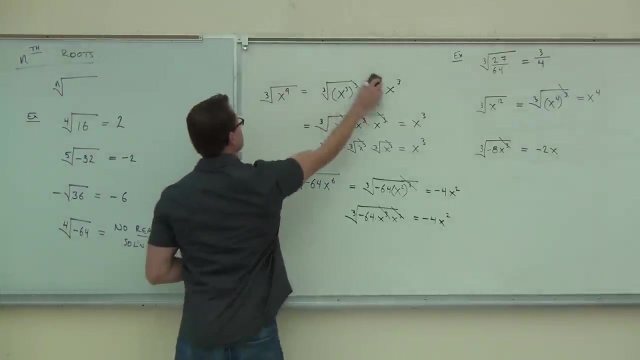 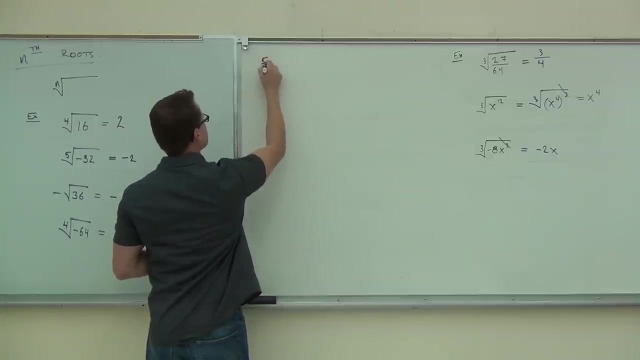 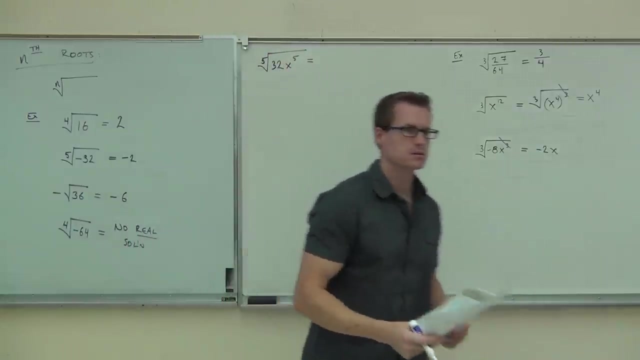 That doesn't work. So we're not going to write just no solution. it's no real solution Actually. no, No, Okay, We won't go that far. How about that one? Can we do that? Can you deal with variables inside of any type of root? 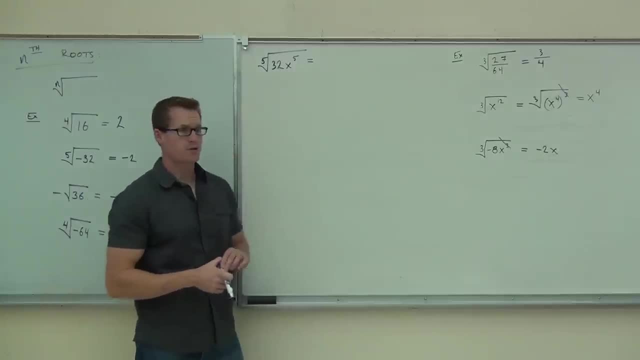 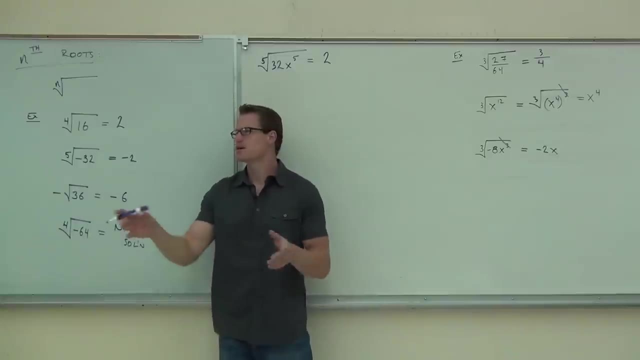 Mm-hmm. Sure, okay, What is the fifth root of 32?? How about the fifth root of x to the fifth? Can you do that? How much do you think it is x? Exactly The same principles apply. 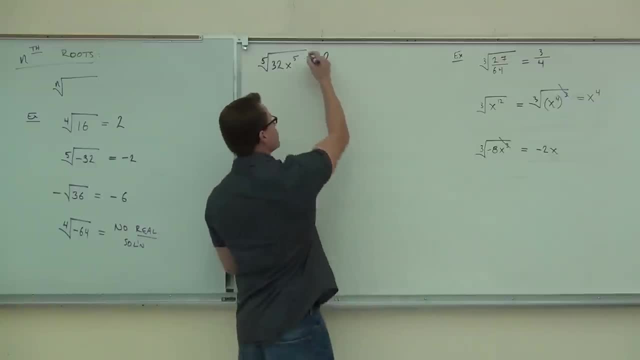 So fifth root, fifth power, those things are also inverse. No matter what your n is, if you have that power inside of your radical, then you're also going to be able to simplify that. So that's just 2x. There's just 2x. 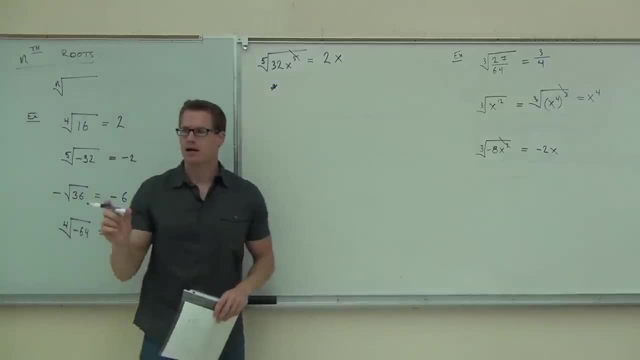 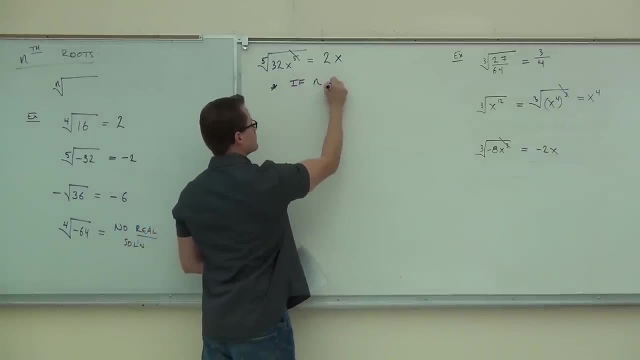 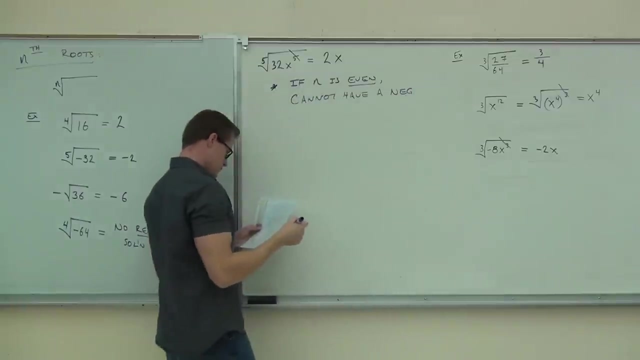 So a couple notes that we just learned: If n is even, you cannot have a negative as part of your radicand or inside the radical. If n is odd though, that's fine. 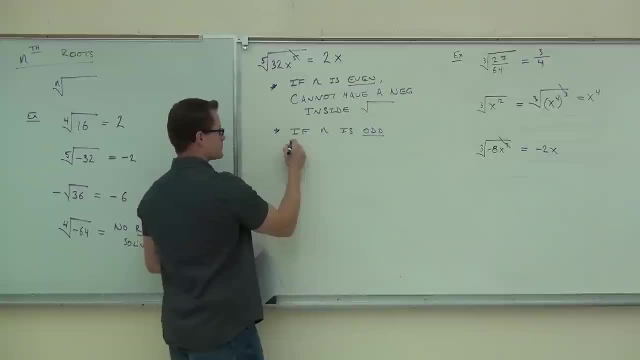 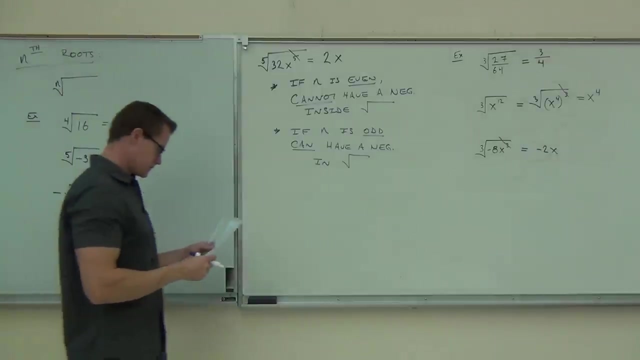 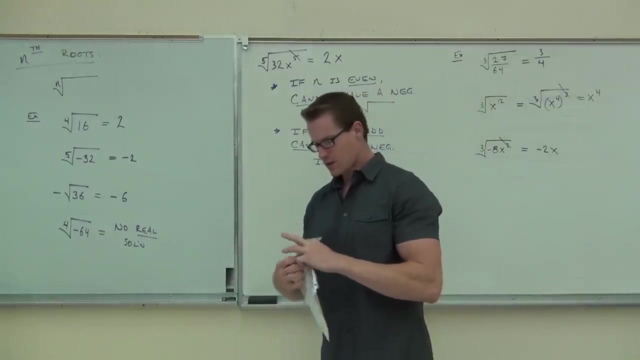 the last thing we're going to talk about. we won't get into the graphing today. I just want to show you one more thing. the graphing actually is just a refresher on a previous topic that we've covered. 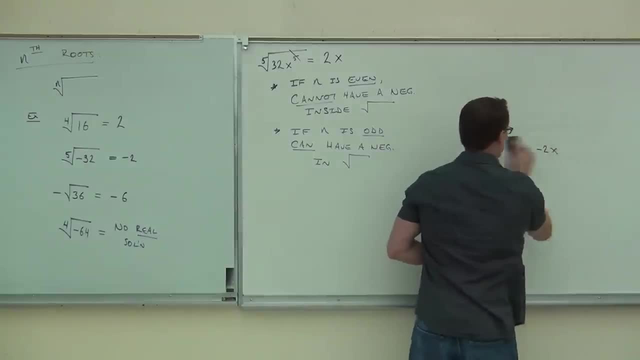 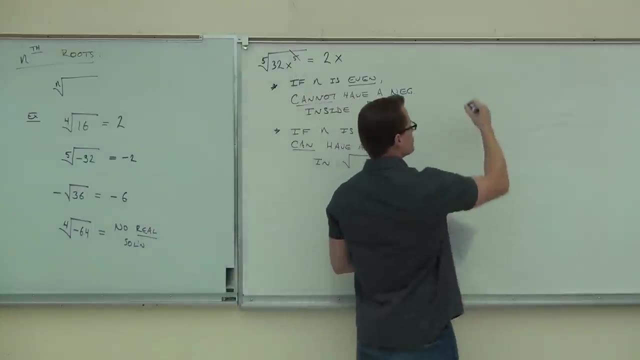 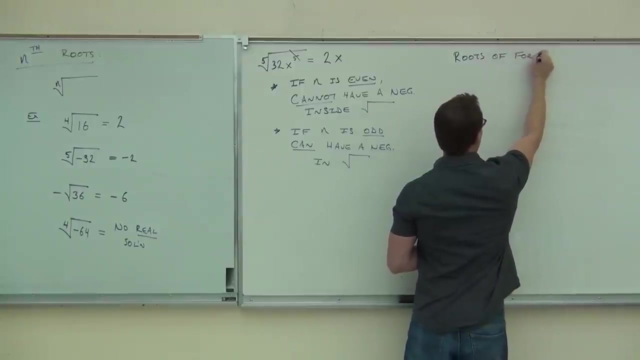 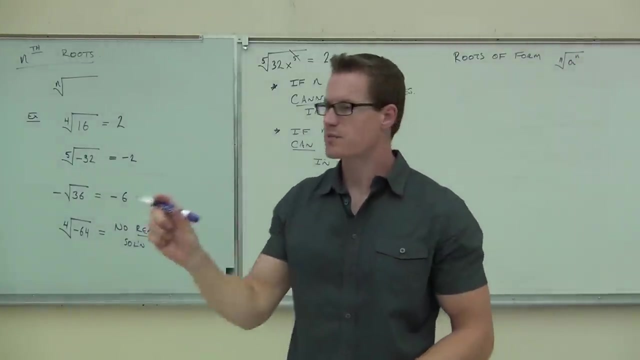 the last thing I want to show you. we're going to talk about roots of the form, nth roots of something to the nth power, where the nth power and the nth root match up. you see, there's one little I don't want to say like a catch. 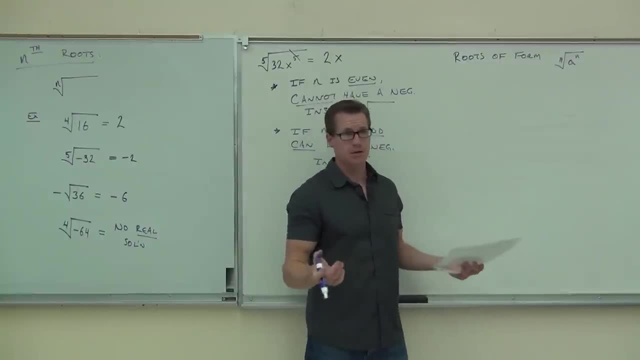 like this is trying to trick you or something. but there's one idea that you need to be aware of when we talk about these type of roots, and here's the idea: let's say that I have a root of something to the nth power. let's say that I have. 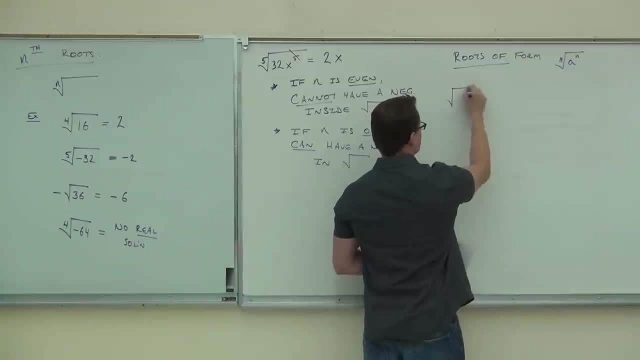 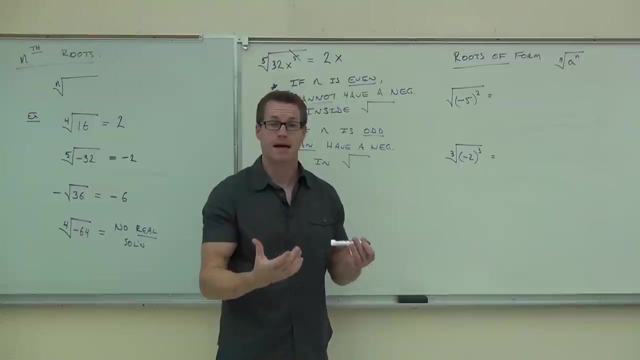 a square root of negative 5 squared and I have a cube root of negative 2 cubed. here's the issue. I need you to know why this is kind of a problem for us in one case and not a problem in another case. watch on the board here real quick. 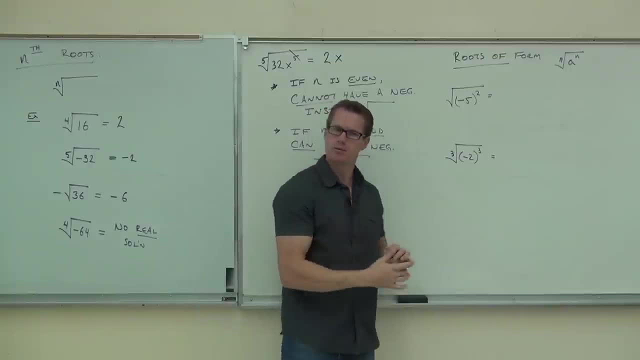 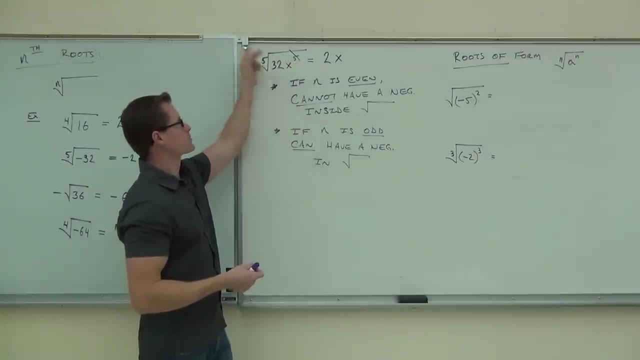 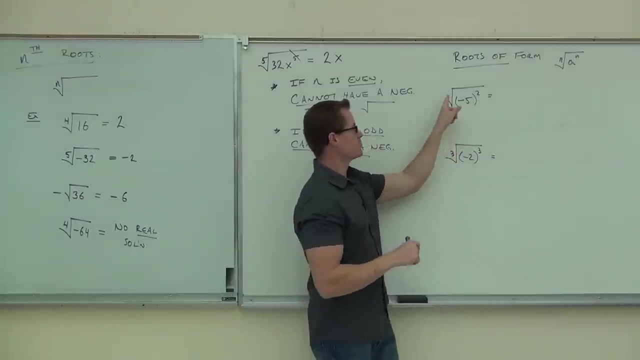 if you understand what I'm saying. I need you to get this little point down. firstly, you are okay right that whenever a power matched the root, we can just cross it out, understand? so in this case, I want you to look at the board. in this case, we should be able just to say: 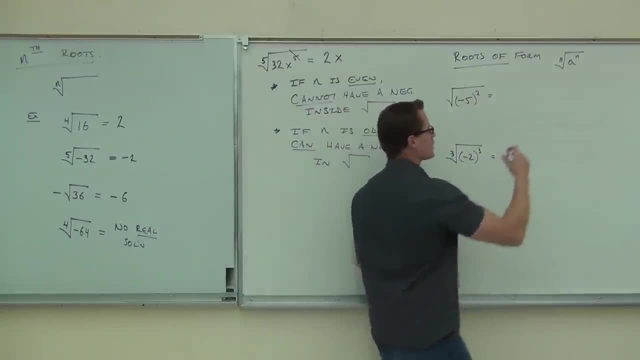 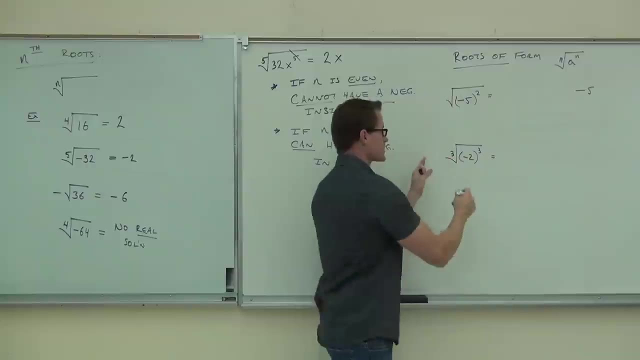 oh, that's a square root, that's a square. I should be able to cross that out and we should be able to get negative 5 out of that. do you understand that we should be able to do that? if that's true, in this case, we should be able to cross out. 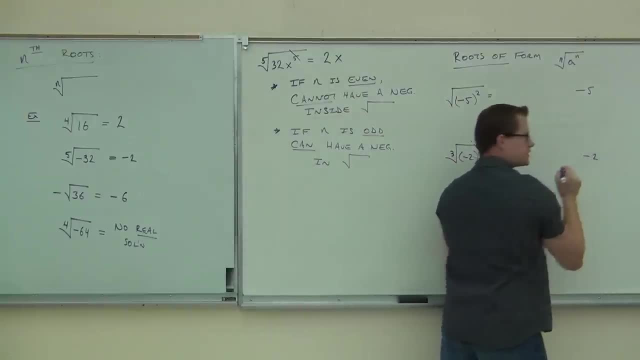 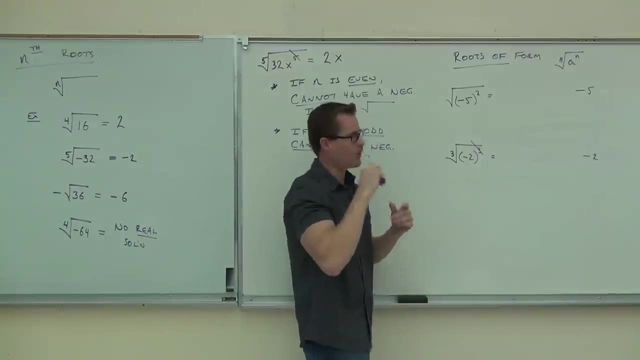 the root of negative 5, squared the third power and the third root and get negative 2 out of that. are you with me on this? that's exactly what we just did. however, I need you to notice something. if you really do the order of operations and go: oh well, this is. 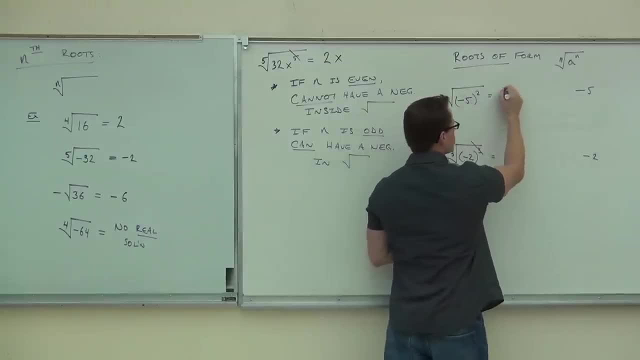 what's negative? 5 squared, actually 25, that's a square root of 25. what's the square root of 25? folks? now we know that one's true. right, because we just did it. are these things equal? no, that is what. why shouldn't it just? 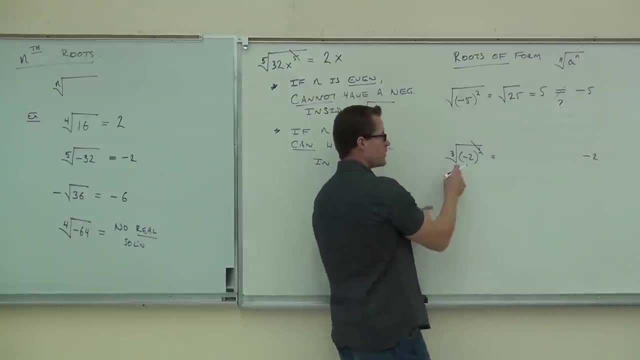 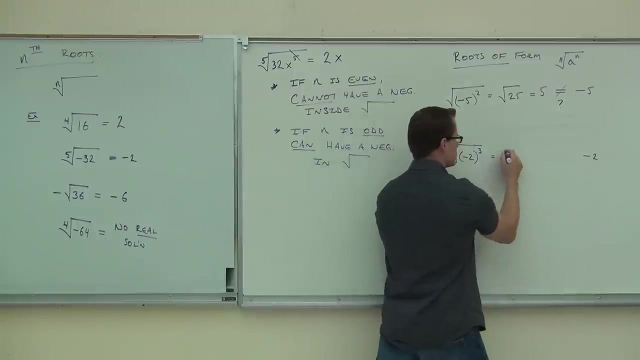 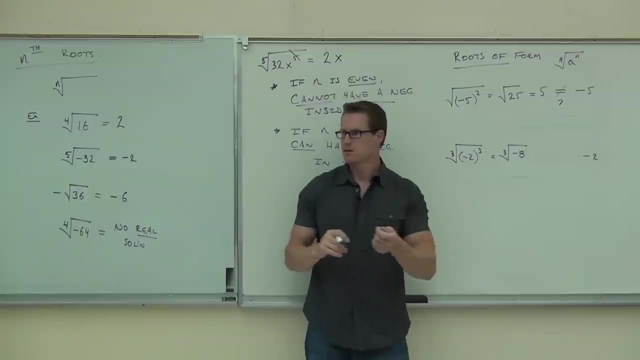 shouldn't it just do that? why does that happen? on this case, though, check it out: if we have a cube root, if we have negative 2 to the cube, what's negative 2? cubed negative 8, sure? what's the cube root of negative 8? 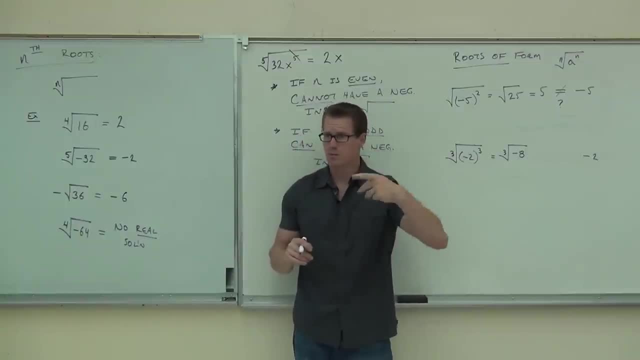 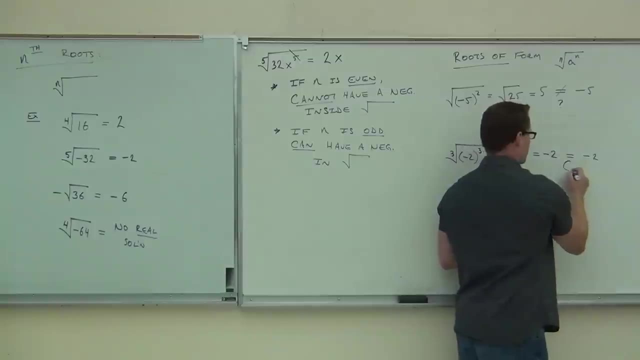 not just 2 right negative, 2 times negative, 2 times negative, 2, that's negative 2 over 2. are you with me on this, folks? these things cool, those do work out the way we want it to. happy face, right, this one. what happened here? 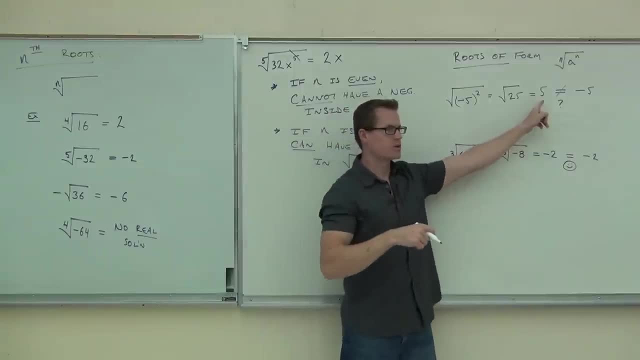 this one's fine, right, this one we can just cross it out, this one we couldn't. and Lily's over there saying, yes, this one's even one's odd. yeah, of course, that's actually the reason why, if you have an even power, what it does is it says inside your root. 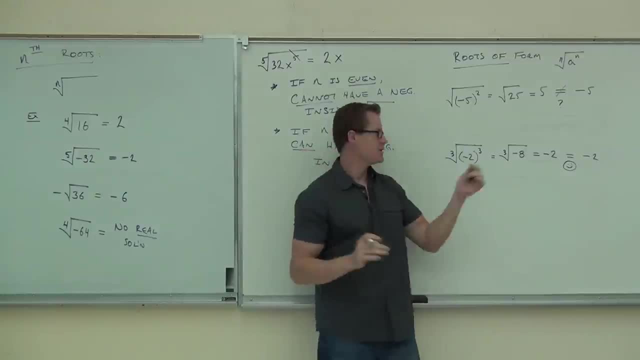 it says: oh, I'm going to make whatever you have positive right, no matter what the negative. the negative inside of a third power or 5th power or an odd power is saying: I'm going to keep that negative, that's fine. so what we get out of this thing. 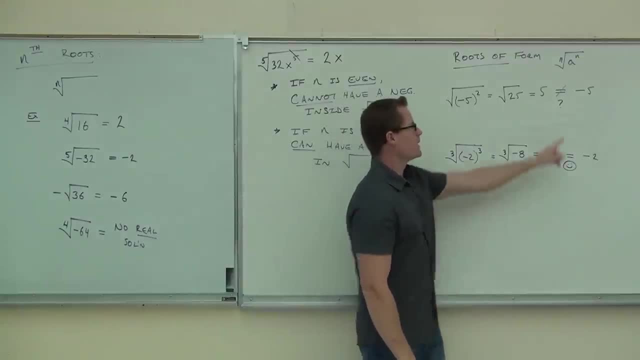 is that we can't just cross this out. how can I change, by the way, a negative, this one, to match up to what we actually know? how do I change this into this? what do I do to change this into this, something we've already used in this class? 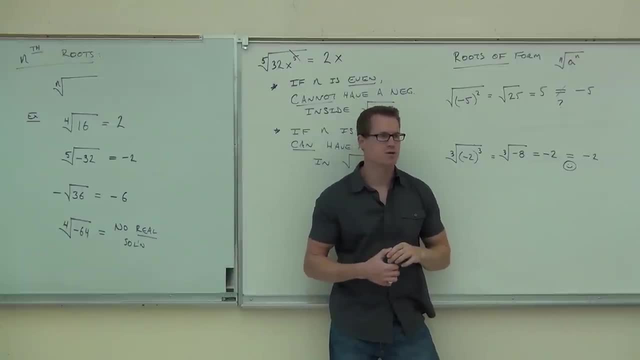 in the previous section, in section 9.3 and 9.2, what changes the positive to a negative, no matter what We could multiply- I don't want to multiply by anything, though, so another option to that is a good idea: Absolute value. 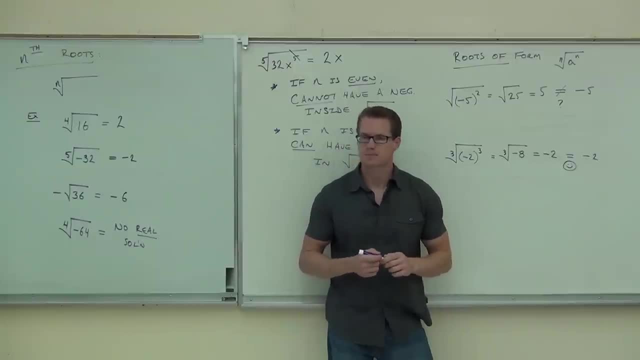 Absolute value. Here's what we need to know about this. When you take an even root over an even power, what we get out of this is not just that we can cross this out and get negative 5. What we do is we cross this out, sure. 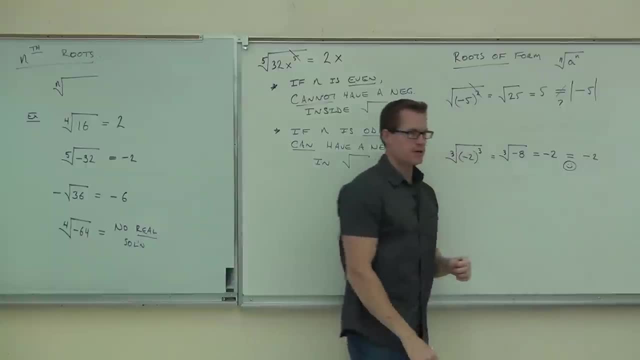 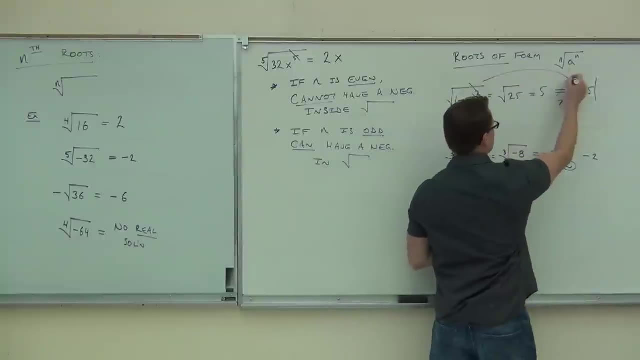 but what that actually equals is the absolute value of negative 5.. What's the absolute value of negative 5? 5. 5. That would make this true. Do you see that? That would make this true? Now we have something that's equal and we get another smiley face. 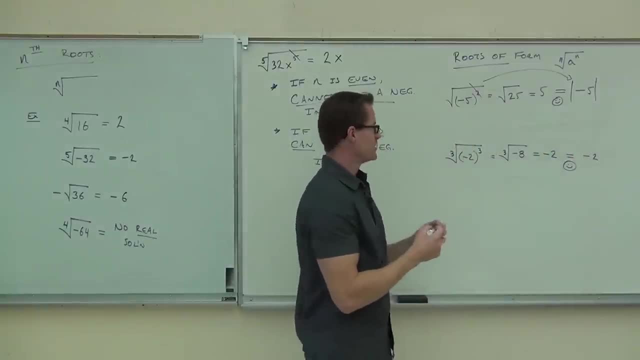 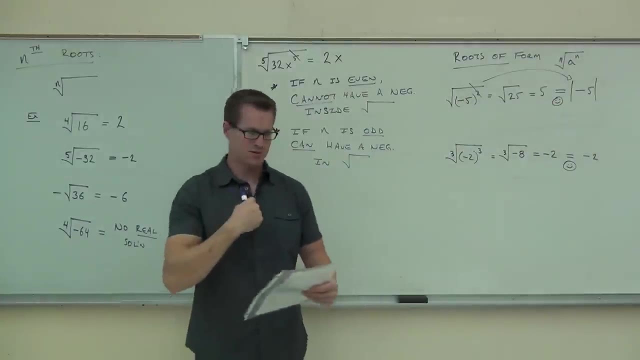 That's for some reason looks like a weird smiley face to me. kind of freaky. I wonder who came up with this stuff. It's me. Here's what we're just learning right now, The last thing we'll probably write down here. 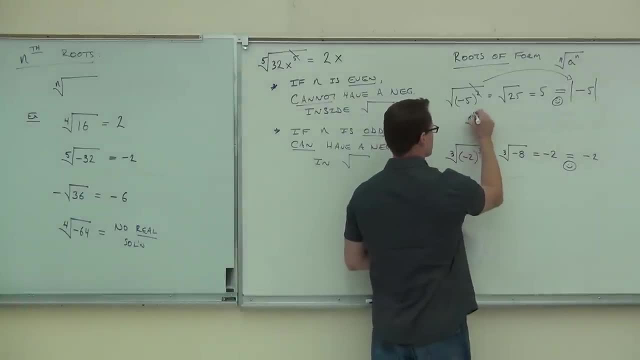 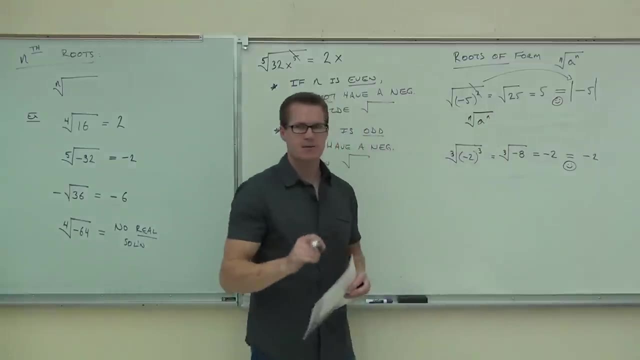 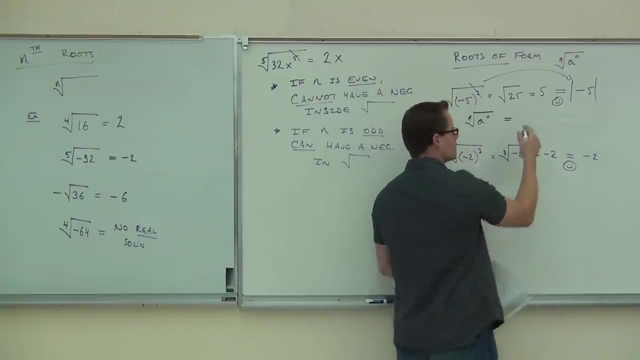 What we're understanding is that if n is, even if n is even like it is here, what this is going to equal is: you're still going to be able to cross things out. An nth root still matches with an nth power. You're seeing that right. 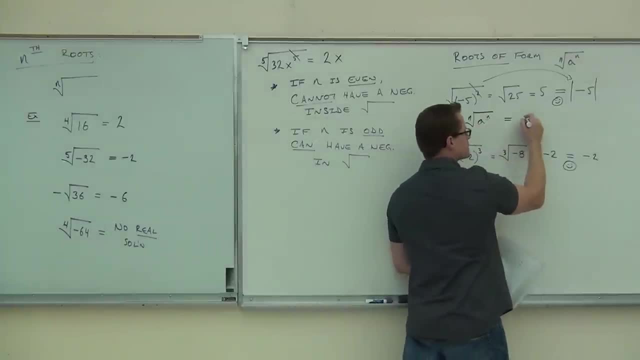 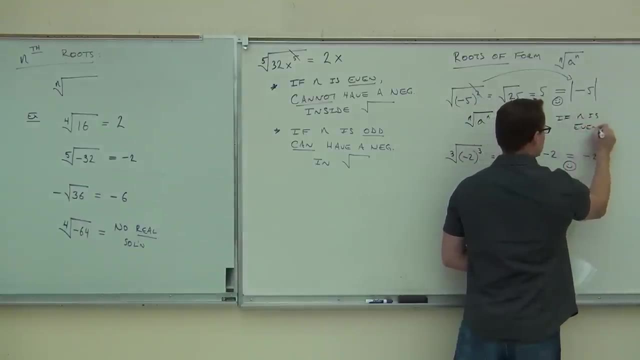 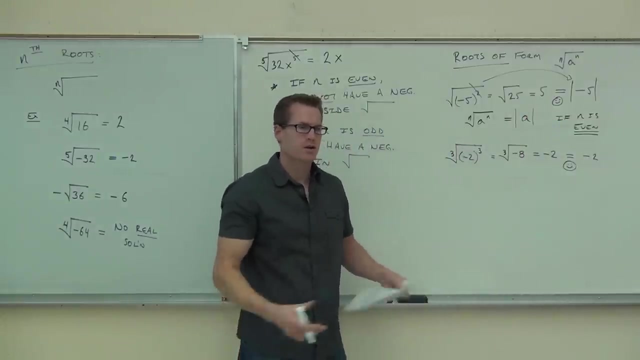 They still match up. However, if n is even, what you're getting is not just a. we're getting the absolute value of a, getting the absolute value of a, not just a right, Because we know that here our a is negative 5.. 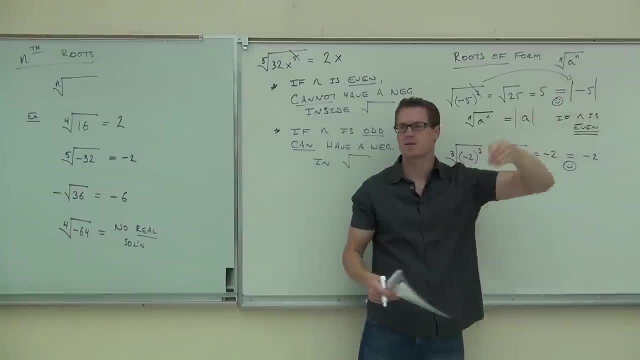 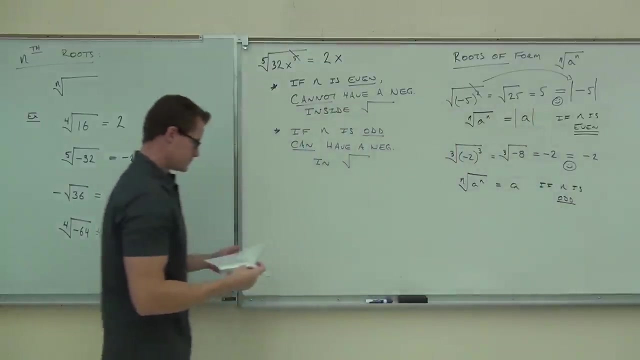 We're not just getting negative 5. We need to be getting positive 5. We're going to take the absolute value of that. If n is odd though, it doesn't matter, It doesn't matter. I want to show you a couple of examples in our last minute here, just to make sure that you guys really see this. 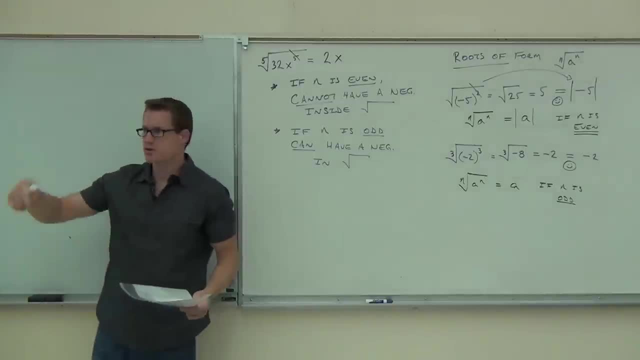 By the way, these don't take a whole lot of work. You're not even going to work on them. You're just going to cross stuff out and understand that one of them is going to have an absolute value and one of them is not. 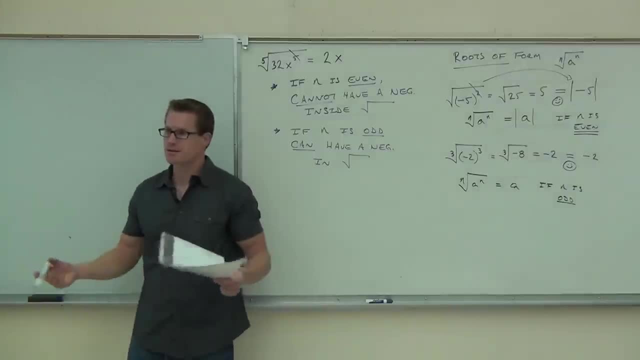 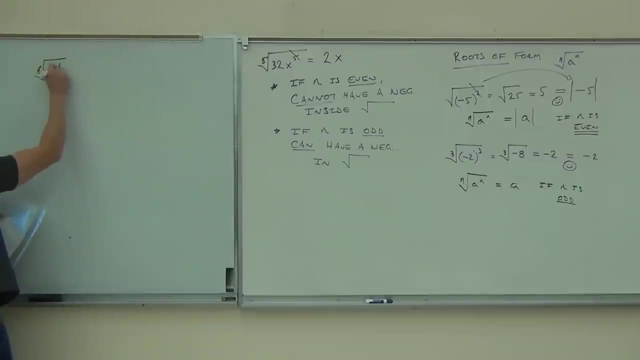 That's basically it. If it's even, it has absolute value around it. If it's odd, it doesn't. So let's do 6 through x to the 6th. Firstly does the power match. That's the root, ladies and gentlemen. 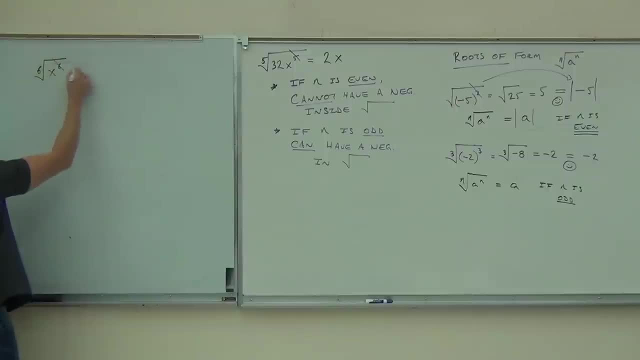 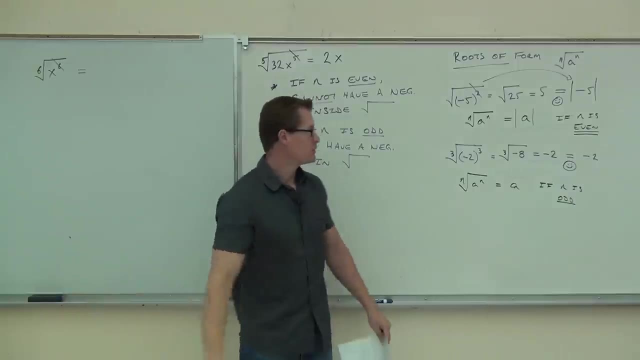 So I'm still going to be able to cross these things out. You just have to understand when I'm going to have to have an absolute value and when I'm not. Do I have an absolute value here? If it's even, if n is even, I'm going to have an absolute value. 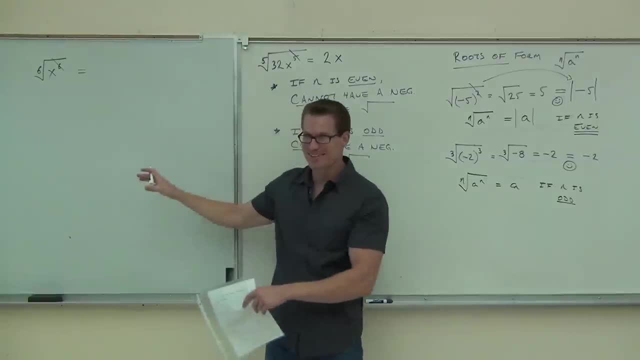 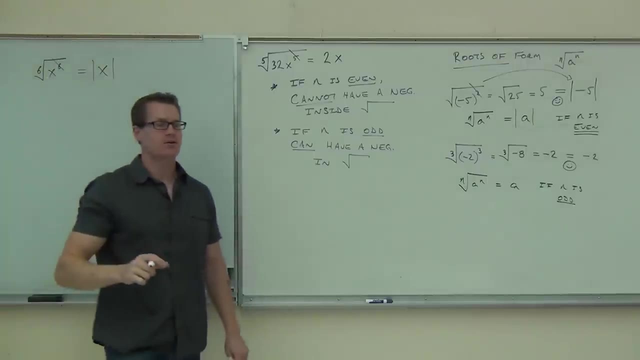 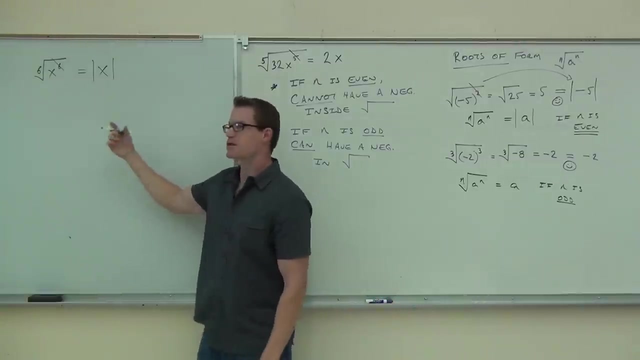 Is n even So, am I going to have an absolute value or not? What the absolute value means is that when you have an even power, even powers make everything positive. What else makes everything positive? Absolute value. So you can cross things out, as long as you have the absolute value. 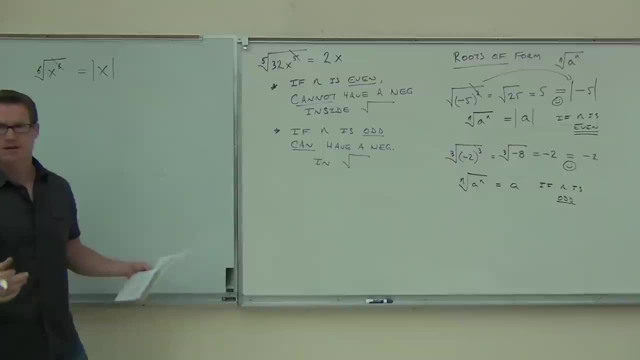 That's what even does. Odd doesn't make everything positive, It leaves negatives negative. Therefore, when I have an odd n, it doesn't matter, You can just write the n itself. So here's one. How about this one Cube. root of negative 3 in parentheses cube. 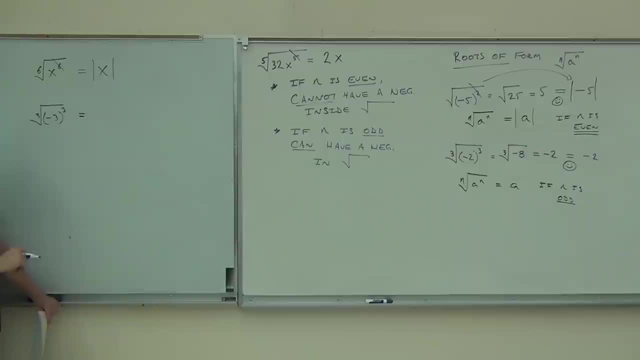 Am I going to have an absolute value or not? What's the n? What's the n here? There's only one number, It's a big one, right? Three, They're all three. Just say three. Yeah, That's your n, right? 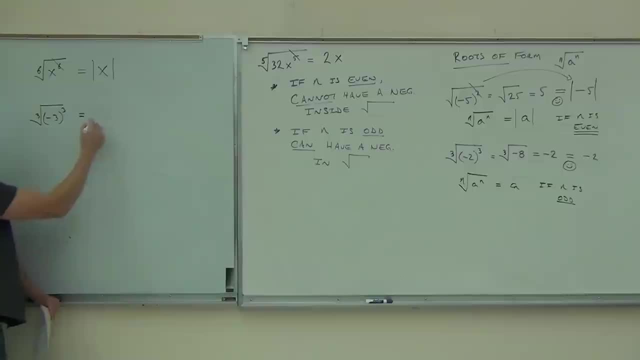 n is 3.. It's an odd Odds. don't make everything positive. Therefore, we don't need an absolute value. How about that one? Does the power match the root? Do we need an absolute value or not? So there's no work here, folks, if it matches up. 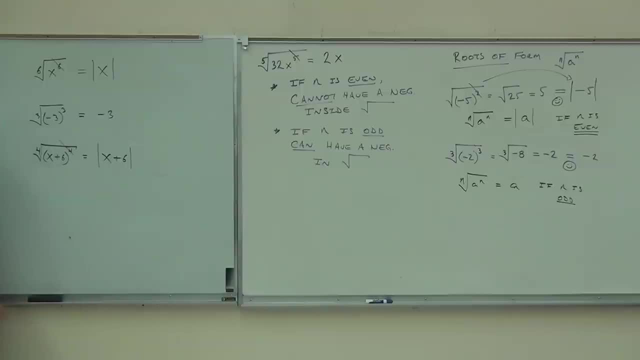 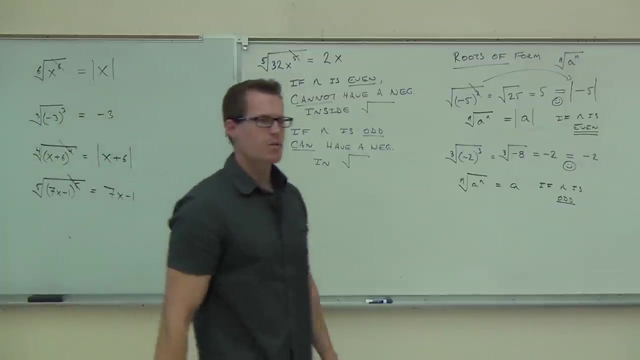 You know it's going to simplify. You just have to know whether you need an absolute value or not. What do you think on that? one Absolute value or not? No, Absolutely not, Because it's odd. you don't need an absolute value. 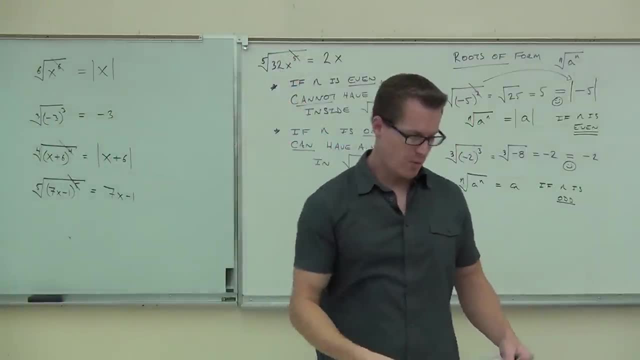 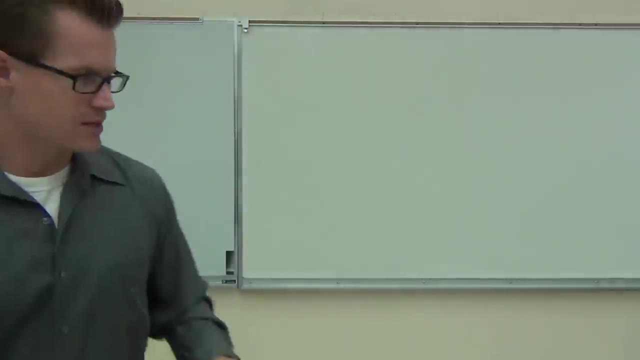 But you have to feel pretty good about this stuff. Okay, we have a couple more ideas on this, maybe about five minutes. We'll do this after our test on Wednesday. So the last thing we've got to do, we've got to graph some of these radicals. 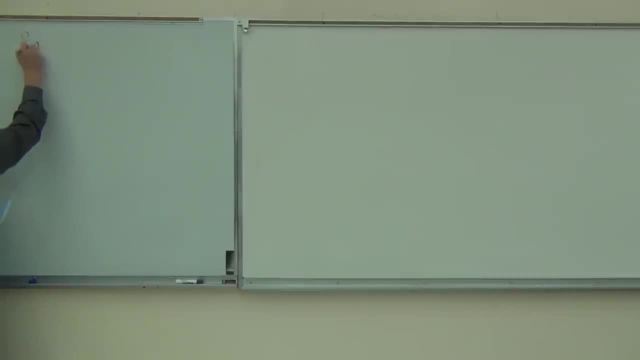 Again, I'm going to refresh your memory on how to graph just the square root of x, But then I also want to graph the cube root of x, And we're going to do this with a table, just to be thorough, because we really don't know how this one looks. 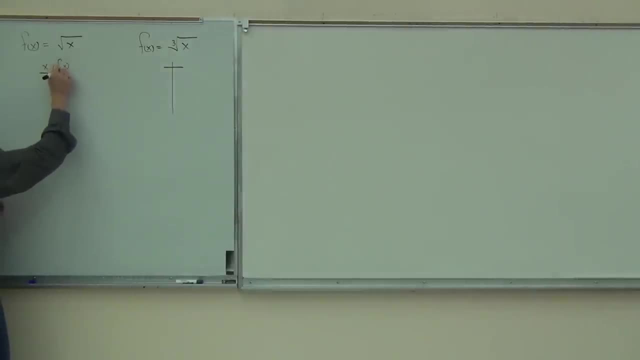 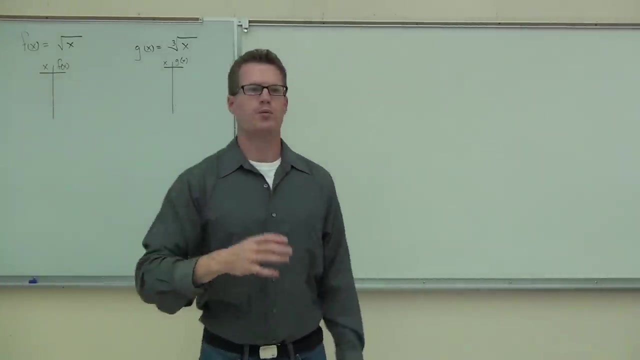 Let me change that to a g. Now. when we're graphing tables, we typically use just three points for lines. However, with these things we're going to use, like four points, four to five points to make sure that we're really thorough and understand what's going on. 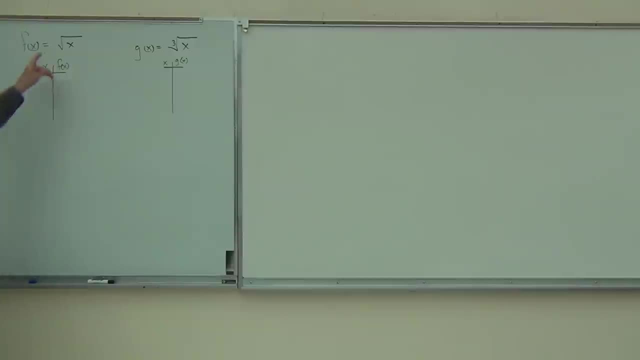 So let's go ahead and pick out some points for the square root of x. What points am I going to want to use here? What's one point? I always use Zero. Definitely one to zero. I'll put that right there. Another point I might want to check out is one. 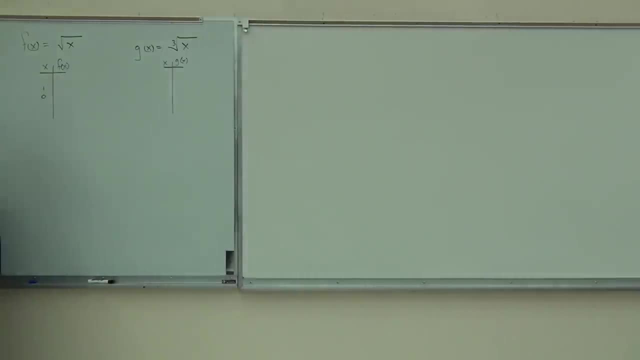 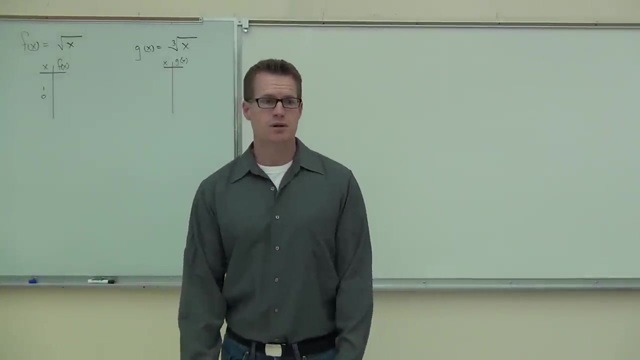 because it's easy to plug in. So let's find out what happens at one. How about two? Am I going to want to plug in the number two? No, Can you find the square root of two? No, You can. You can on a calculator. 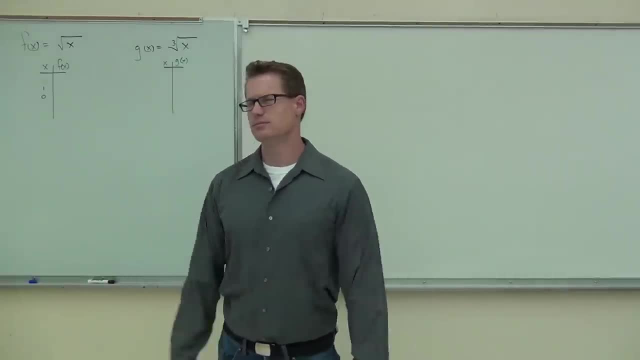 But if you just go square root of two, you go 1.41? I don't know. Yeah, it's 1.41.. But you're not going to probably know that. You definitely don't want to graph it on the graph, do you? 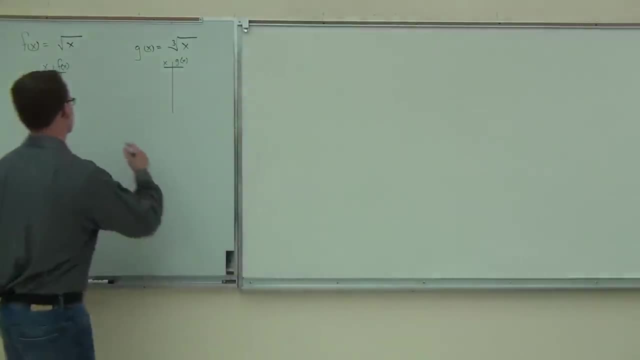 No, What number do you know? the square root of Four. Let's pick four And give me one more. Nine, Nine. Let's do nine four. one zero. Let's pick out some negatives, negative numbers. What do you want to pick for a negative number on the square root of x. 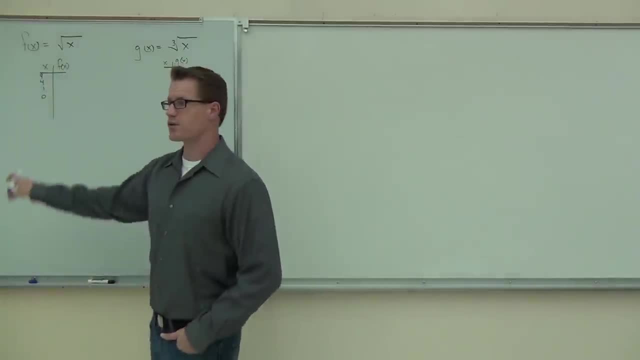 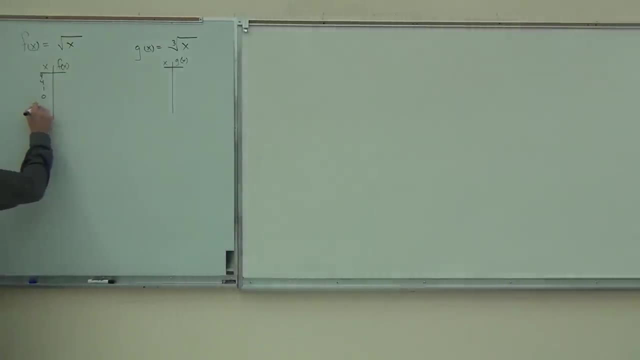 One, Negative one. Okay, we'll try negative one. You know what? Let me give you some more space here, so you can see those numbers a little better too. We had nine, Nine, Nine, Nine, Nine, Nine. 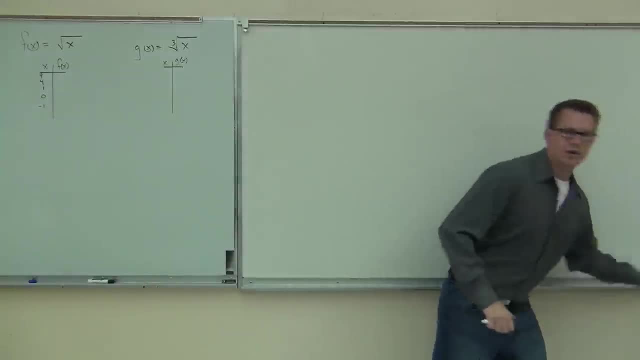 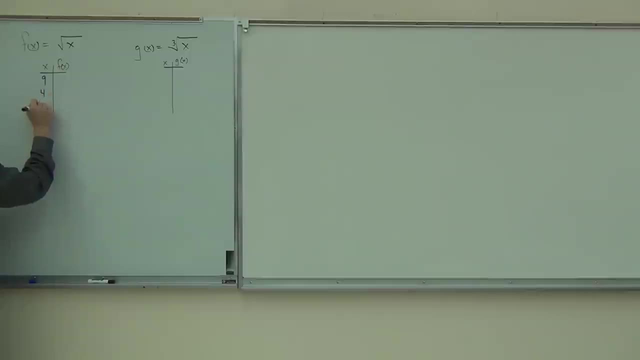 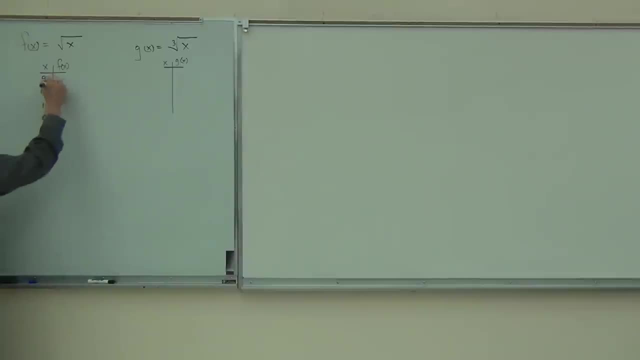 That'll be good enough for us. Let's see, We're taking nine, We're going to plug this in. What's the square root of nine, ladies and gentlemen. Three, Okay, So that gives me a point. Nine, three. 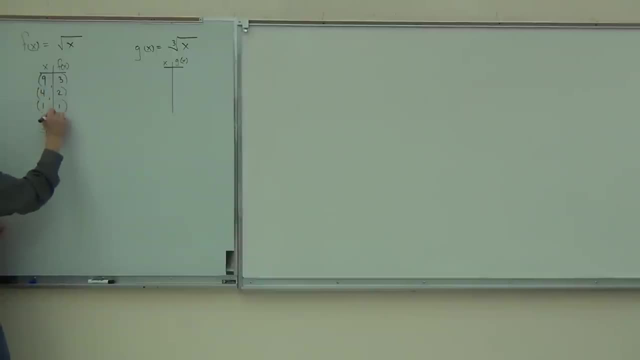 Four: what's square of four, Two, 12.. That gives me a point four, two: How about the square root of one, One One. Square root of zero, Zero, Good, that is possible. zero square root of negative one. 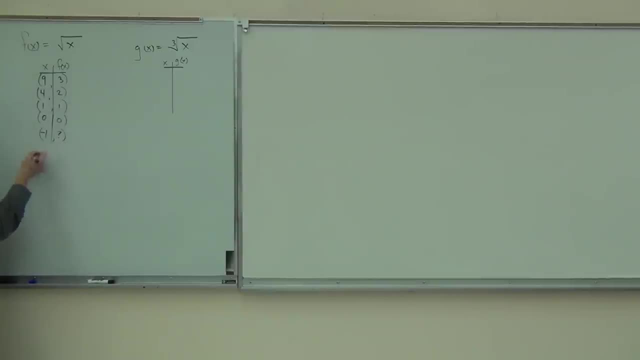 There is a nine Close Ah-ha Square root of one. that doesn't even happen. That's why on our graph, when we graph this thing, there's nothing on this side of our graph, because you can't even plug in a negative number. 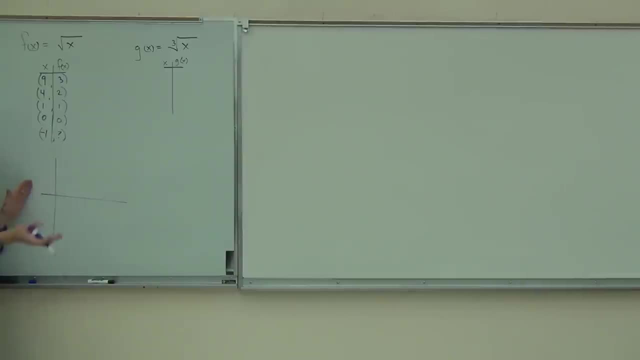 You can't plug in negative one to a square root, can you? No, You get no real solution. So when we graph these points, I'm going to start from the bottom up. I know 0, 0 was there. I know 1, 1 was there. 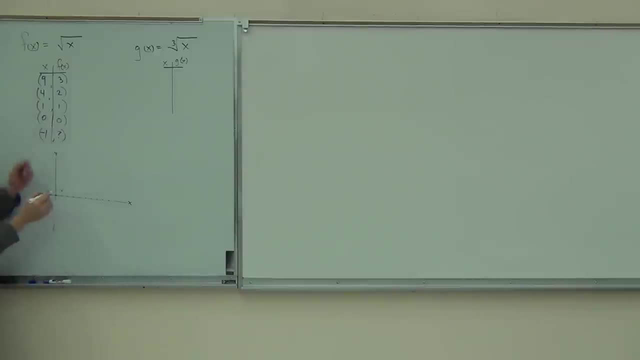 But then we have to go all the way over to 4 to get a 2.. So notice that this is x, y. So 1, 2, 3, 4, 2.. That's right here. And then to get up to 3, I have to go all the way over to 9.. 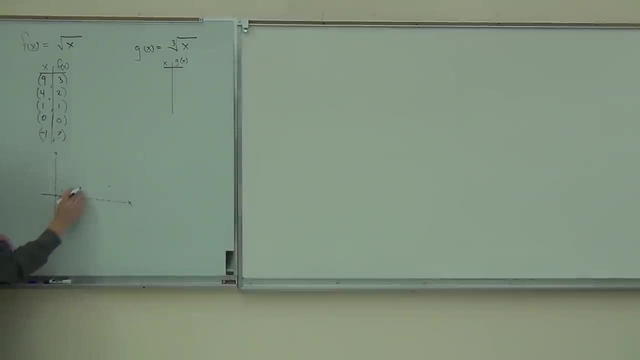 So 9, 3 is my last point. That's why we got this funny-looking curve. It's a half of a parabola on its side. That's why it kind of looked like a square root. actually, That's our graph. 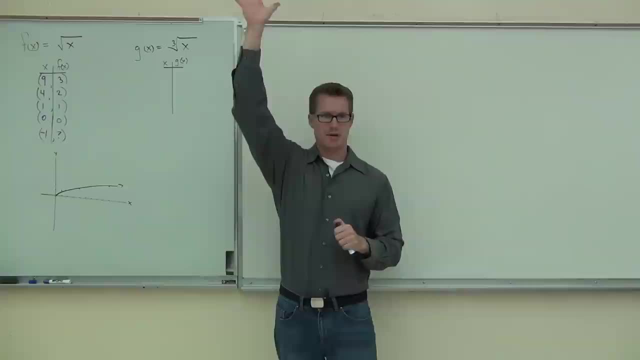 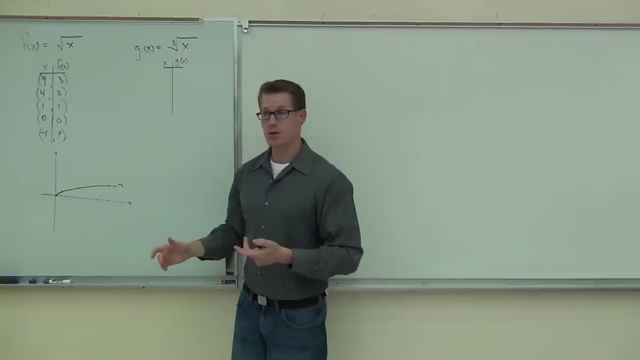 Do you guys remember that graph? Yes, It's from a while back. How many people do remember that? feel okay with it. See where these points are coming from And, most importantly, do you understand why we have no graph on this side of the y-axis? 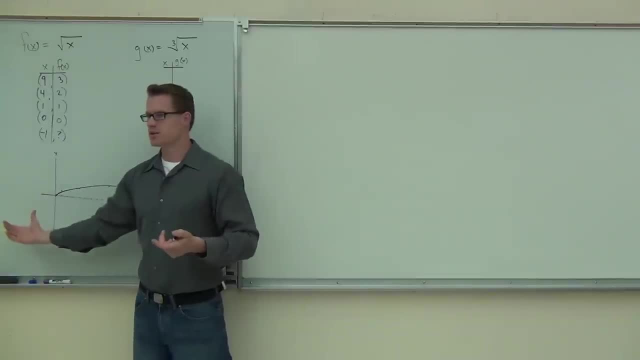 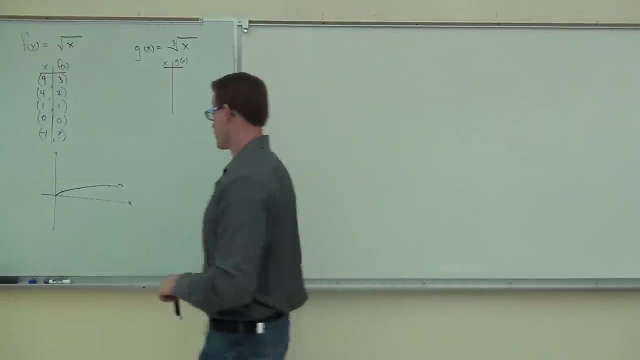 Yes, Do you all understand that one Can't plug in negatives? That means you're not going to get anything out over here on this section. Now let's see what happens with our cube root x. I still want to plug in. 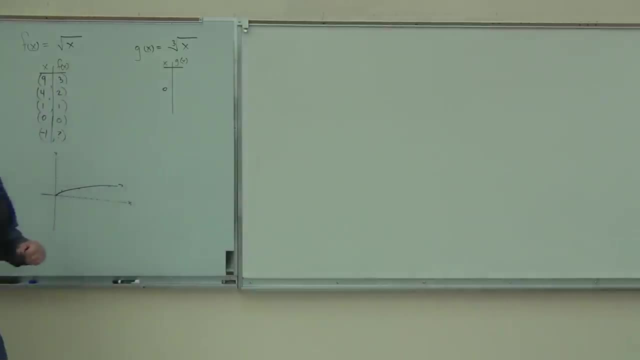 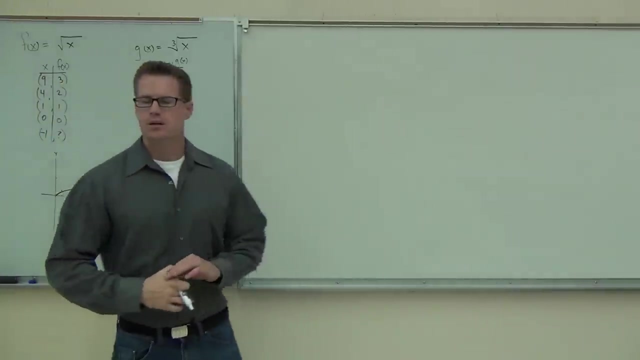 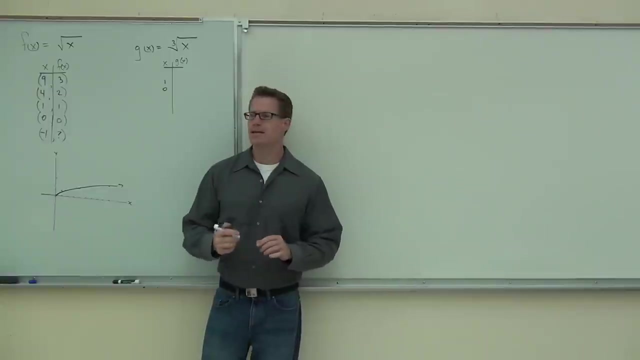 I definitely want to find out what happens there And I want to see what happens at 1.. Now do I want to see what happens at 4? Can you take the cube root of 4?? What can you take the cube root of? 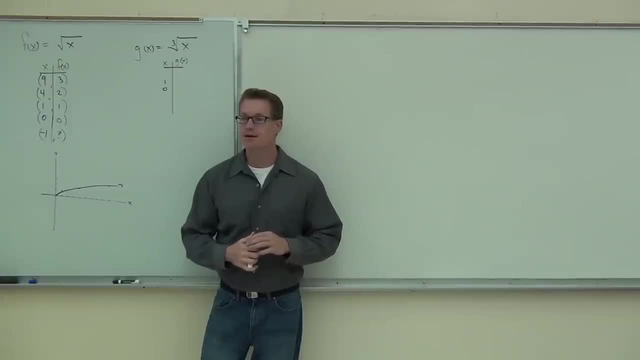 Not 3.. Not 9. 27.. Some people said that three times now I can do 27.. You're right, I can do 27.. But you know what? I don't want to put 27 on the hash marks because I am lazy. 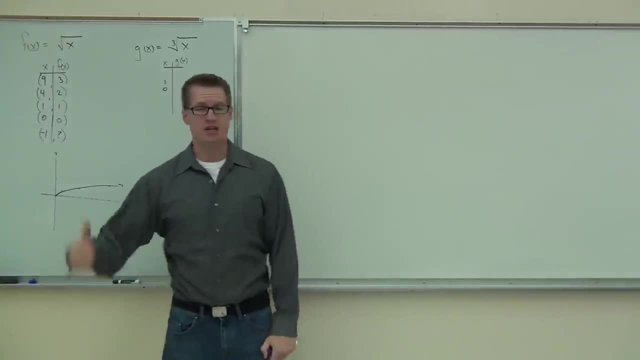 and I don't want to draw a graph that's this big. So, yeah, I can check 0 because 0 is nice. I can check 1 because 1 is nice. 2, what's the cube root of 2?? 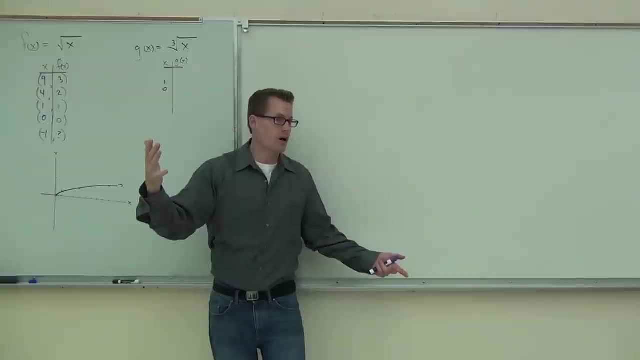 You go. I don't know What's the cube root of 3? I don't know. Cube root of 4? I don't know. I can take the square root of that. Cube root of 5?, No 6?. 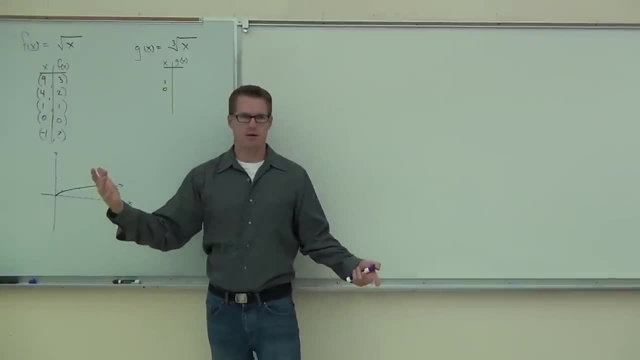 No 7? No 8? Yes, 9? No, 10? No, The next one would be 27.. So the numbers you can take the cube root of are the same numbers that we've actually only been taking the cube root of, which are 0,, 1,, 8,, 27.. 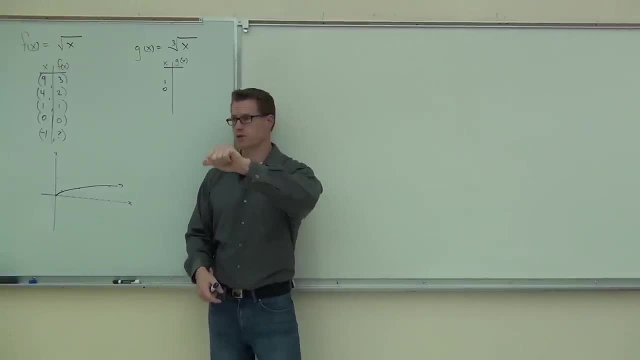 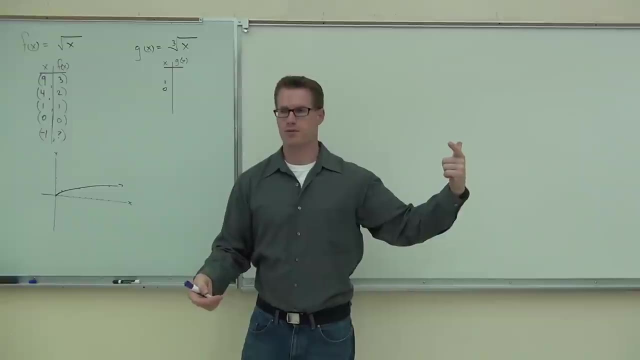 64,, 125,, 216, all right, Those are the only ones between there and 200 and, well, 300-something. So 343 is the next one for 7 cubes. So you don't want to do those right. 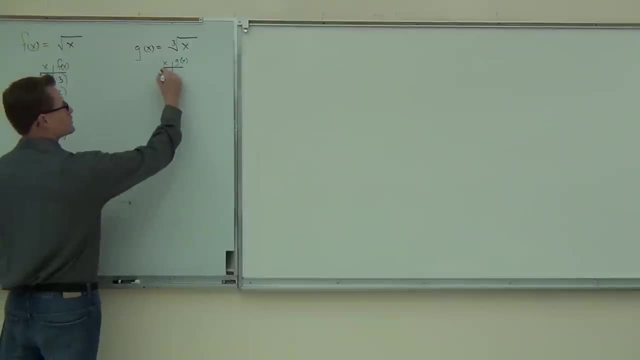 There's only a few of them, So the only ones we can pick are 0,, 1, or 8.. Maybe 27, if you really want to draw a large graph. You don't want to. Now let's try some negatives here. 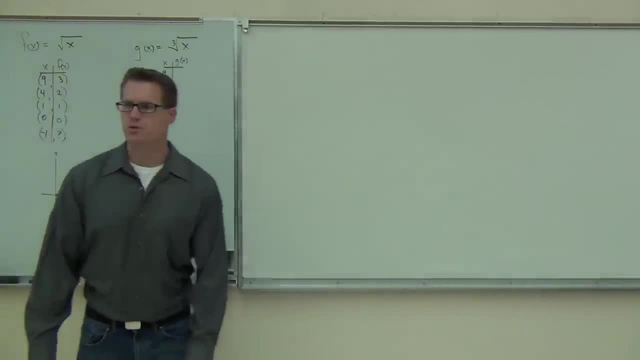 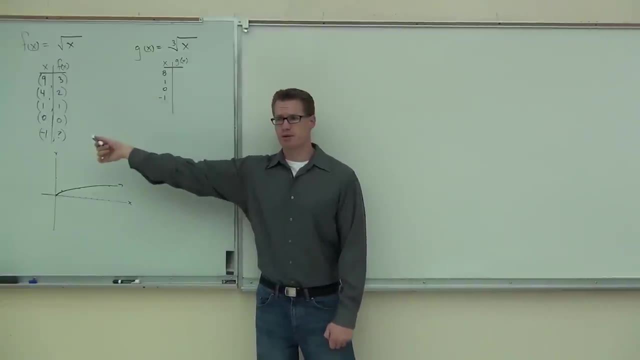 Let's try a negative 1 again. Let's see if that works. Is negative 1 going to be negative? Is negative 1 going to work in this particular problem? Is there a difference between a cube root and a square root? Yes, 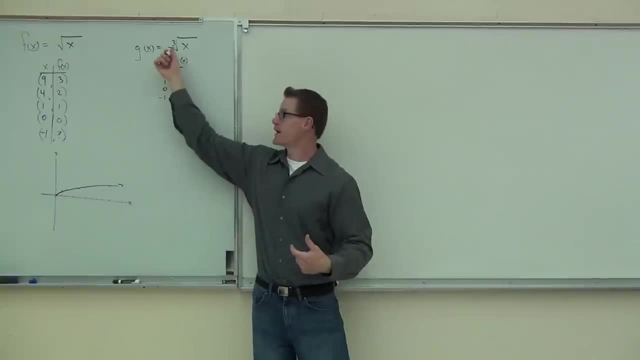 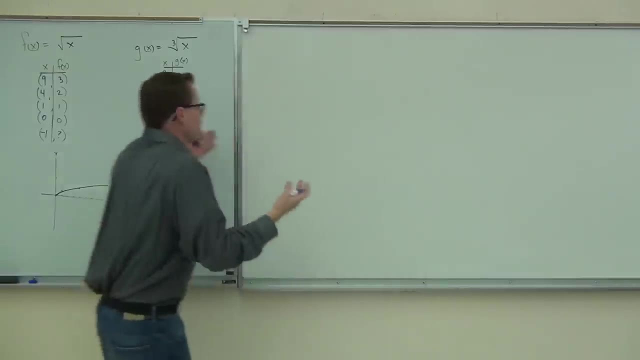 Yes, Cube root has one extra time, A negative and a negative, and a negative could potentially give you a negative, couldn't it So that for this reason, we can actually plug in negatives into our graph? We couldn't here, because a negative times a negative. 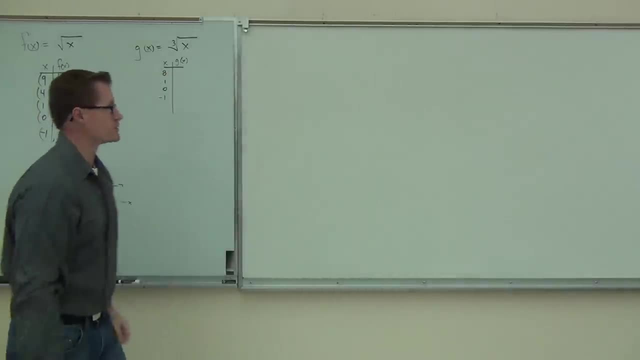 the only two times won't give you a negative. It'll always give you a positive. But we're doing three times equal to radicand. So a negative, negative, negative potentially could give you a negative. Well, always actually. 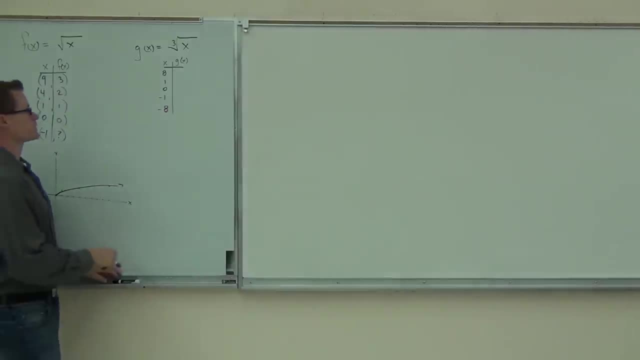 And then we'll try a negative 8.. So let's do this together. If I plug in 8, what's the cube root of 8,, ladies and gentlemen? 2., 2. Good, And that gives me a point. 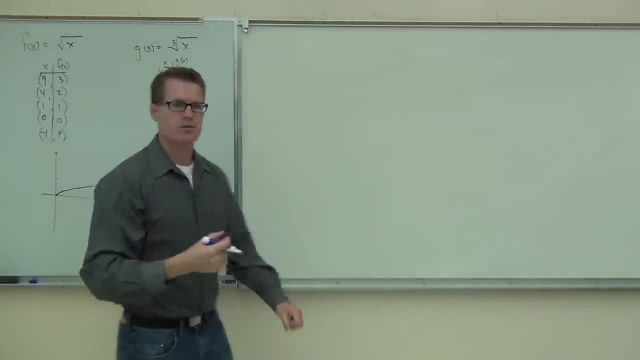 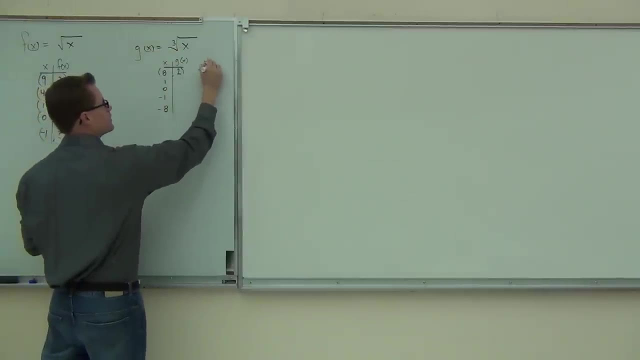 Cube root of 1.. What we're asking here again, remember we're saying: what times itself three times is giving us the 8? This is the cube root of 8.. What times itself three times, It's giving you the 8.. 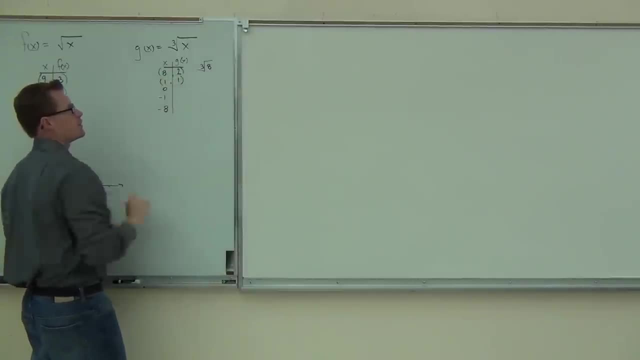 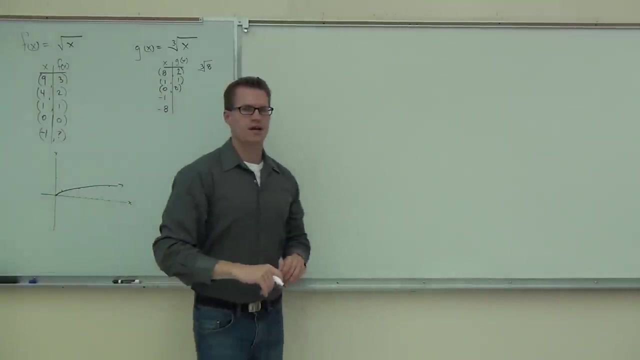 Well, that's 2.. Here it's going to be 1.. How about 0?? What's the cube root of 0?? For sure, What's the cube? Oh, negative 1.. The cube root of negative 1 asks: what times itself. 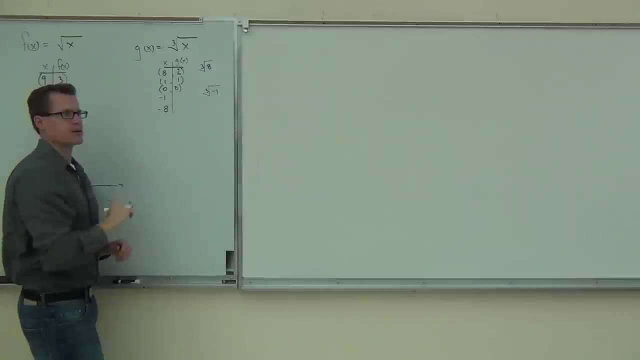 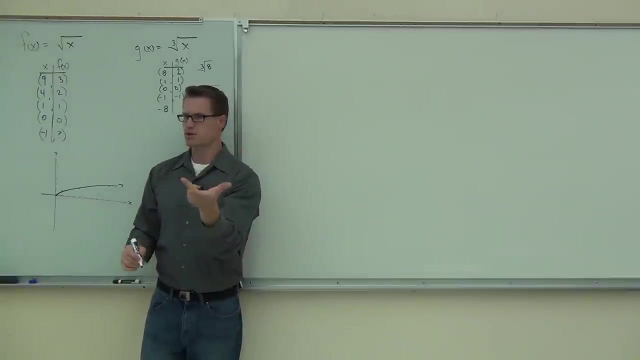 three times gives you the radicand of negative 1? Yeah, let's think about that. Negative 1 times negative 1, that's 1.. Times negative 1 gives you negative 1 again. So that means that our cube root of negative 1 is negative 1.. 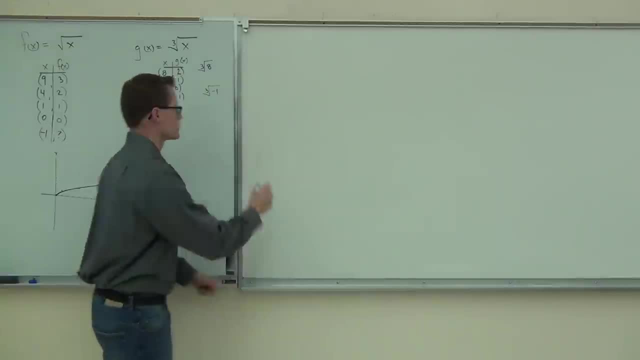 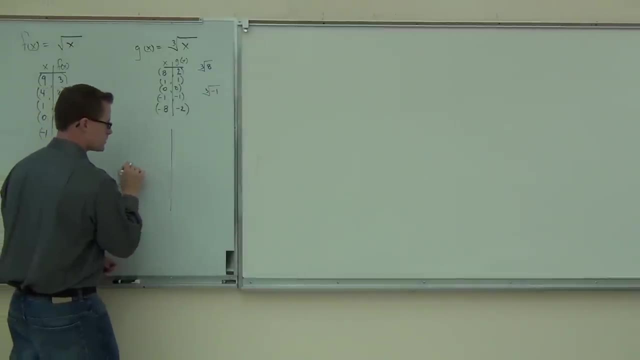 And lastly, cube, root of negative 8, everybody Negative 2. Negative, 2. Good, Well, we've got some points. Let's see what this looks like. Notice that our points do come x comma y, just like always. 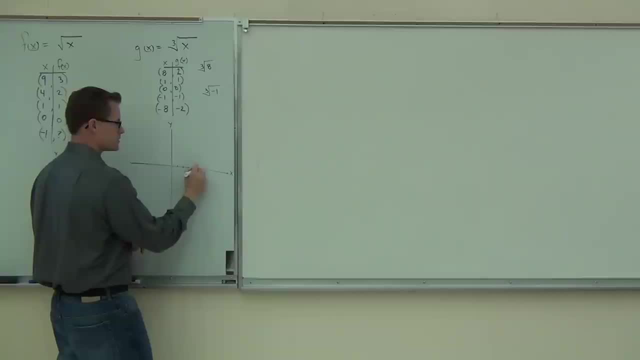 So we have to go over to 8 on our x axis. Also, am I going to have a piece of my graph Over on the left-hand side in this case? Yes, Yeah, this is different than over here. Here I couldn't plug in negatives. 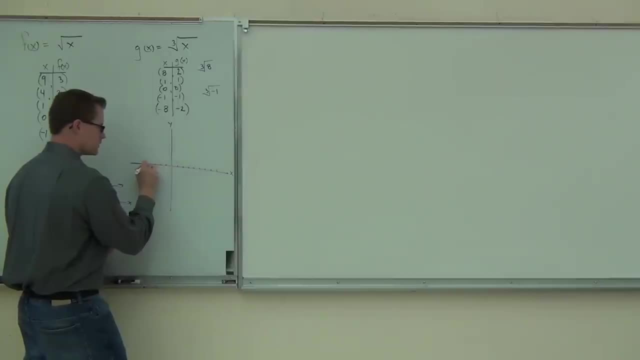 Here I could. Now I'm doing something here that's going to be a little bit off And I want you to see what I'm doing. But I'm doing it just so you can see the graph a little bit better. Do you notice how my hash marks here are a little bit bigger than my hash marks here? 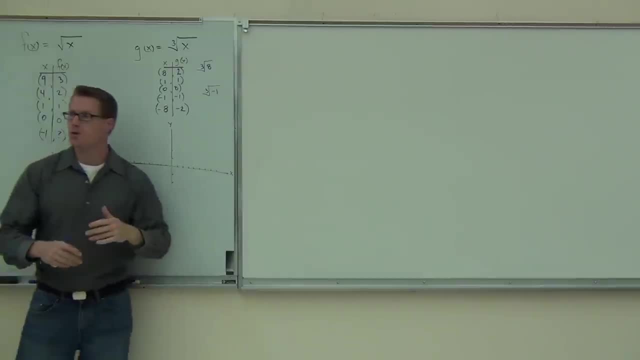 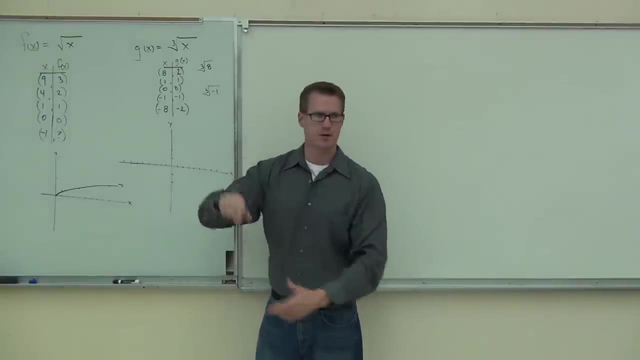 What that's going to do is expand my graph a little bit. this way. This is actually supposed to be a little bit flatter than what I'm going to draw. Are you with me on that? So I'm kind of biasing the graph vertically a little bit, just so we're able to see it. 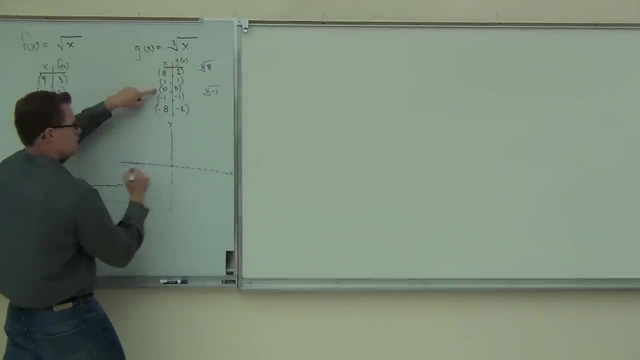 But let's go ahead and plot these points. I'm going to work from the middle. I have 0, 0.. I have 1, 1.. That's here. I also have negative 1, negative 1.. Is negative 1, negative 1 up here or down here? 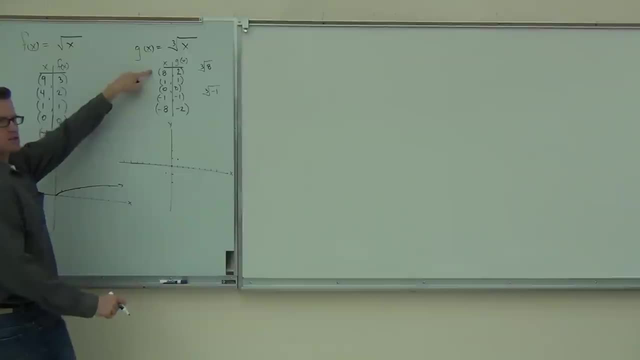 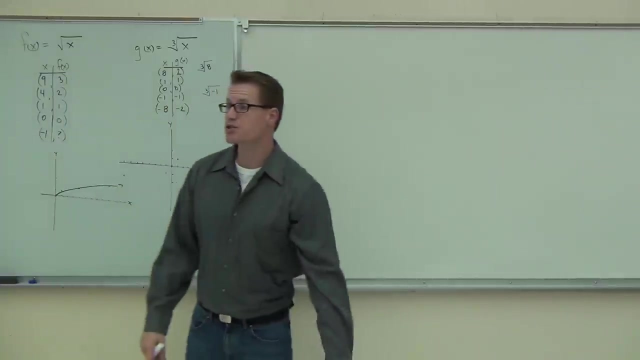 Down. Okay, Then I have 8, 2.. 8, 2.. That's over here. And I have negative 8, negative 2.. Negative 8, negative 2.. That's a weird looking graph. Can you picture in your head what it's doing? 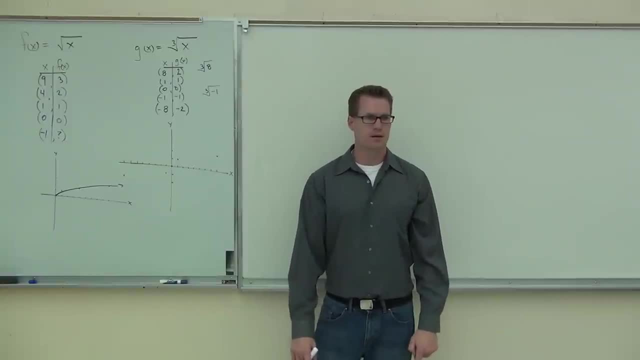 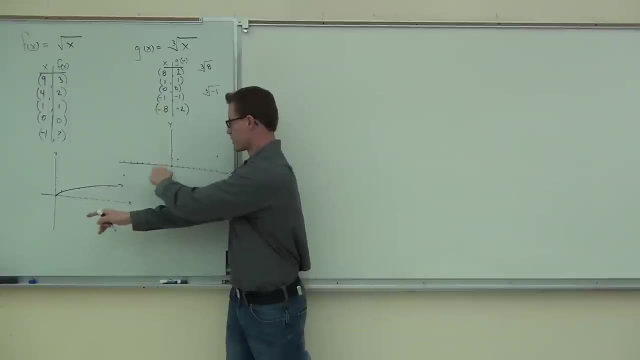 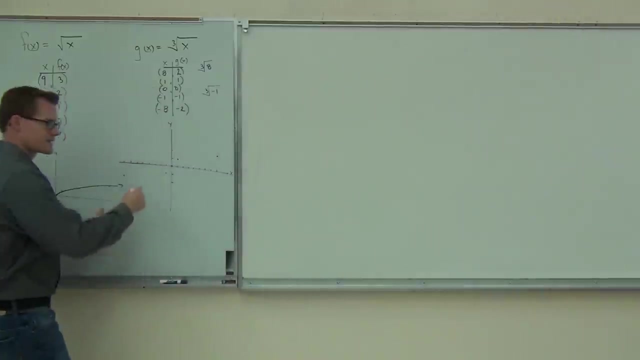 Picture what it's doing. It looks similar to this, doesn't it? For part of it. It looks similar to this for the other part, except it's rotated 180 degrees. All the way around This right here, this graph, it's like an S curve. 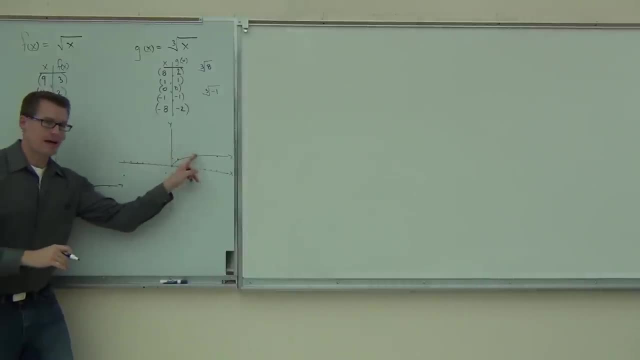 It does do that. Actually it doesn't. it's actually flatter than this. It's flatter than that graph. So I am lying a little bit. I've expanded this just so you can see the curvature of this, But this should be a little bit flatter than this one. 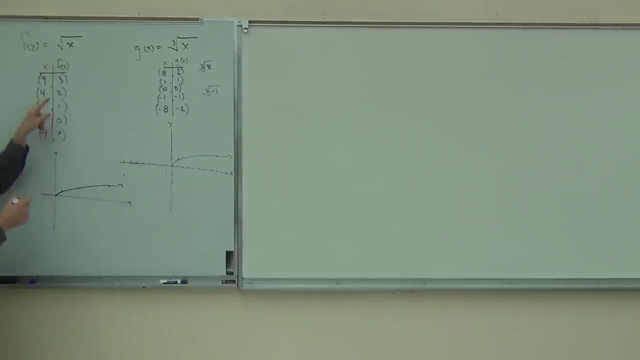 It's more radical, Because notice what you're doing. Here, to get out the value of 2, you only have to plug in 4.. Here, to get the value of 2, you have to plug in 8.. That's going to squeeze it down closer to the X axis. 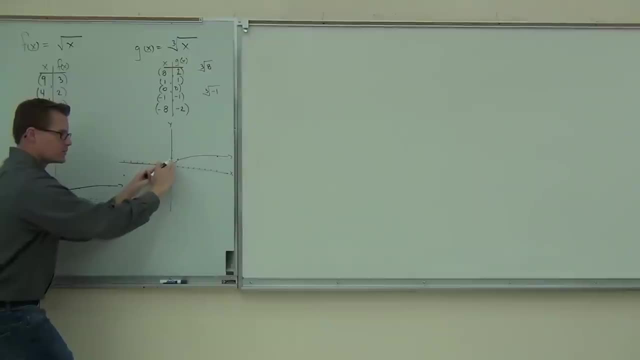 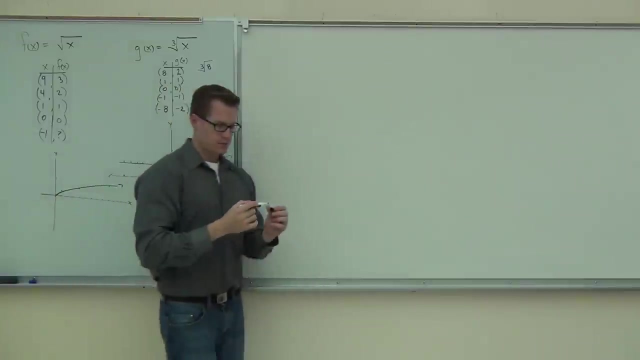 But then this side looks exactly the same, only going below the X axis. It's kind of like a reflection. It's really a rotation, But it does that curve. It's a nice S curve. That's the cube root function. That's the cube root. 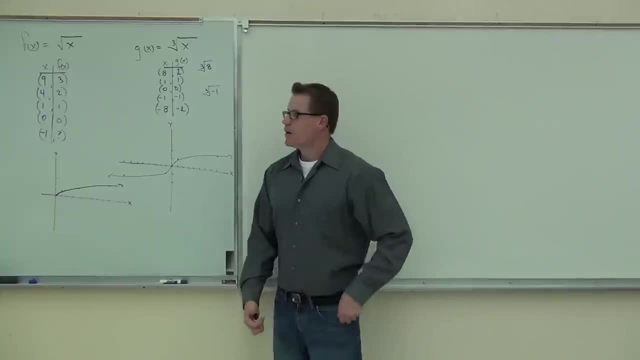 One more thing I want to talk about here. Let's say that I'm not going to graph all these. there's just a ton of them. But let's say we wanted to graph a fourth root. A fourth root- Can you plug in a negative number into a fourth root? 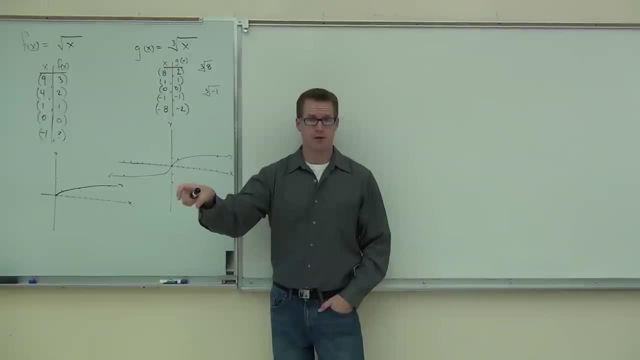 No. Can you plug it into a fifth root? Yes. How about a sixth root? No. Seventh root- No. So what will every even root look like? This one Or this one? What do you think? The square root or the cube root? 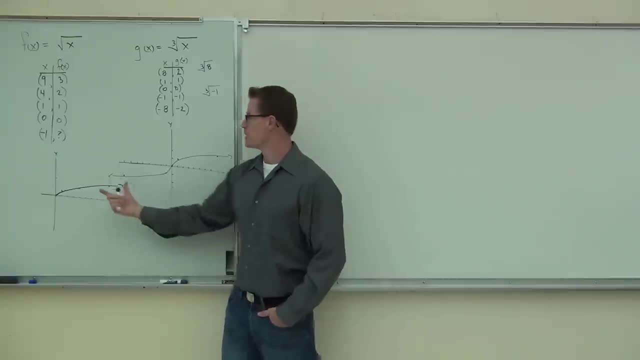 Square root, Square root. Every even type of root- fourth root, sixth root, eighth root, tenth root- will look similar to this. It will have this general shape and only be one-sided because you can't plug in negatives. However, the higher you go up in your root, the flatter this will get. 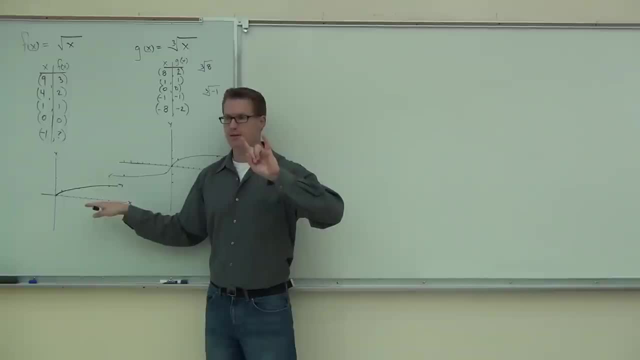 In order to get 2 out of a fourth root, you'd have to plug in 16.. All the way over here Just to get the value of 2.. It's going to flatten that out. It's going to really flatten it. 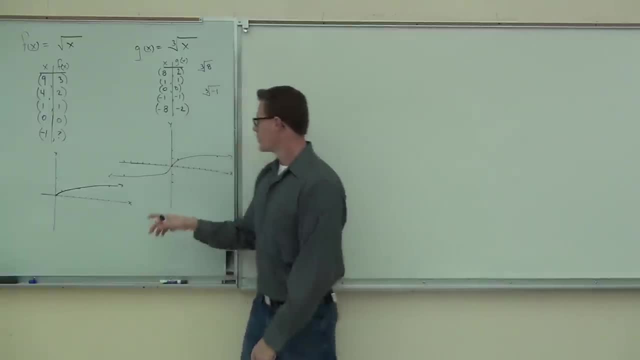 Every odd power root- 3,, 5,, 7,, 9, will look something like this: It'll have this negative version as well, because you can plug in negatives to it, So it'll be some sort of an S-curve. 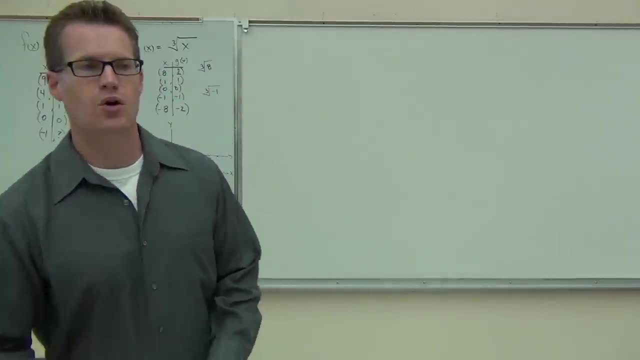 Now the only thing we've got to talk about is the shifting stillness. It still works On your homework. it's going to ask you to make tables for all this stuff. I really don't care about that. If you want to make tables, great. 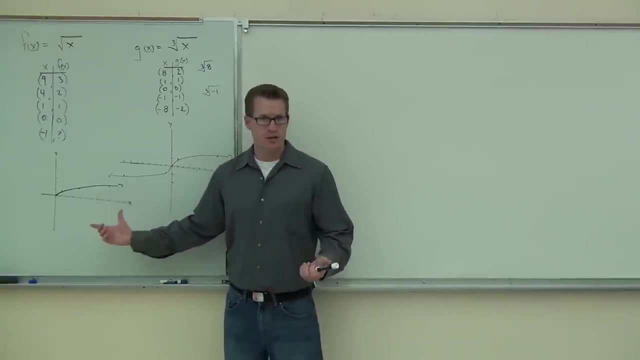 But do you understand the shapes of these guys? If you understand the shapes, you can manipulate them by shifting them around. Now for a fifth root or a fourth root. you might want to draw a table once, Just to kind of see the values and how it looks. 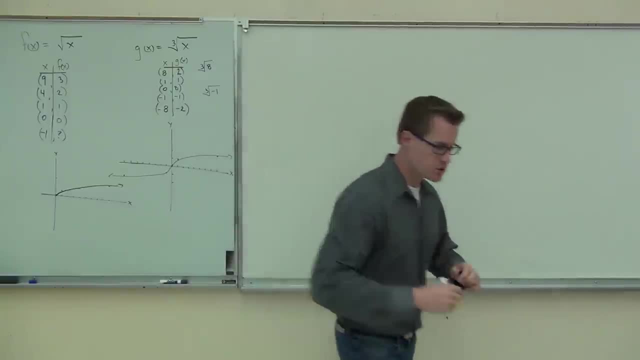 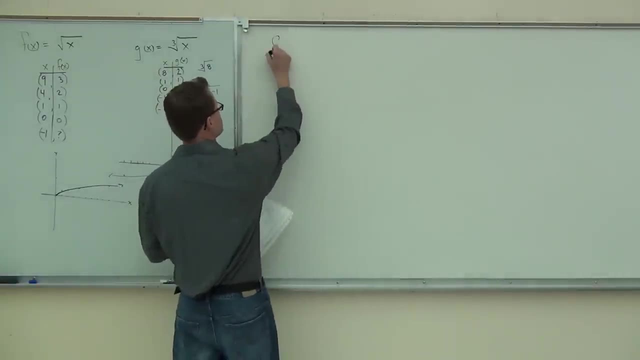 Okay, Draw it one time and then, if it asks you to shift it, go ahead and shift it. So, since we just graphed some of those things on your test, if I ask you to do, f of x equals square root of x plus one like this where it's inside of the radical. 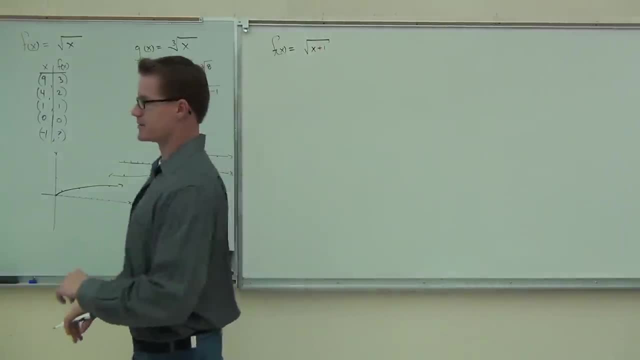 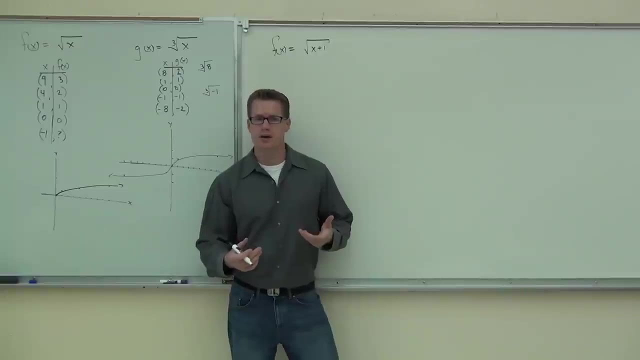 you should be able to tell me what type of a shift that is. Is that a shift up down, left or right? Firstly, let's determine whether it's a vertical or a horizontal shift. Now you tell me, is this plus one within the function or after the function? 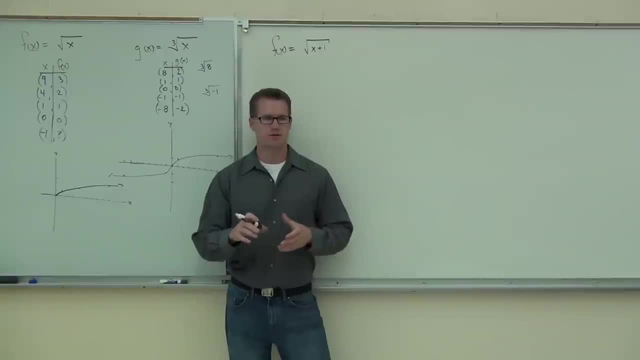 It's within. So is it a horizontal or a vertical shift? Remember after would have been up or down. This is within the square root. That's why this little tail, This tail here, is covering that plus one. This is within the square root. 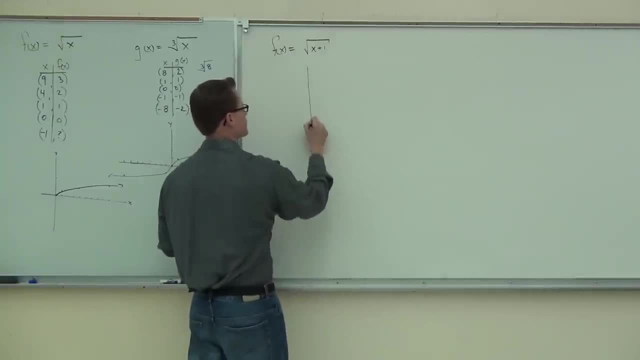 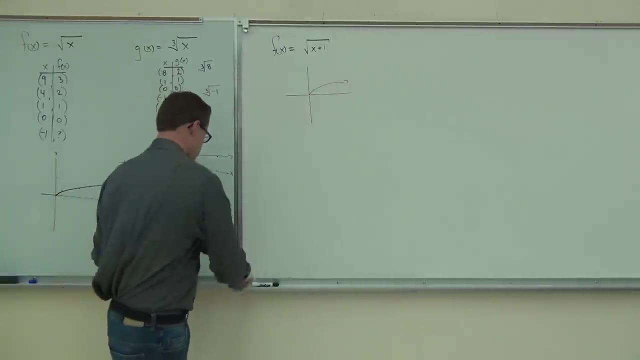 So this is going to be a shift either left or right. Remember, my original graph looks like this. My original graph looks like that. What did the plus one do if it's inside of your function? Was that a shift to the right or a shift to the left? 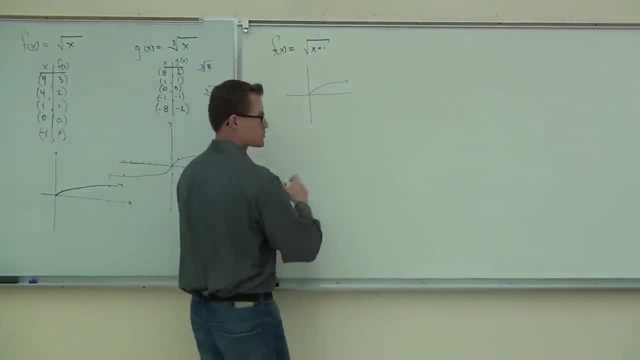 Which one was that Left? That's right, That's correct. So this is a shift to the left If it's inside. it was horizontal And it was kind of backwards of what your head wanted to say. This was left one. 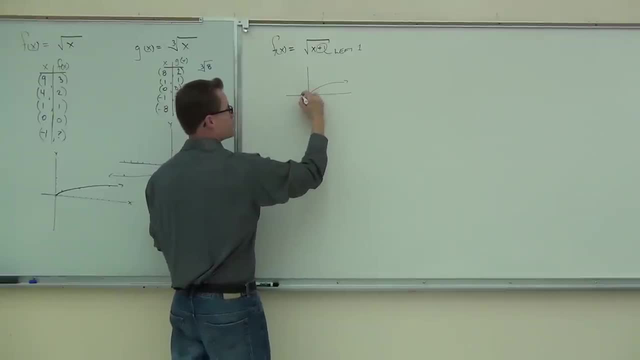 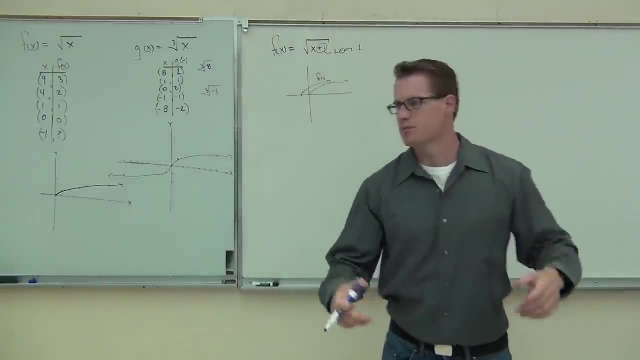 So here we say: oh okay, Let's move over. It takes one spot, Redraw our graph. We can shift these graphs around just like we did before. Are you okay with this? Okay, Let's try one more. 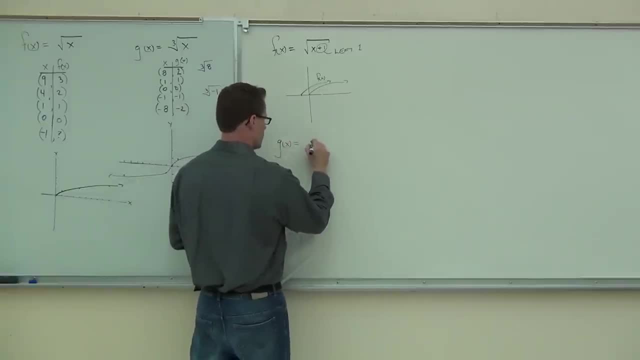 Let's do g of x: Cube root of x plus two. Cube root of x plus two. Of course, you need to know what the shape of the graph looks like, which is why I'm going to have you draw at least one graph using a table for like a fourth root and a fifth root. 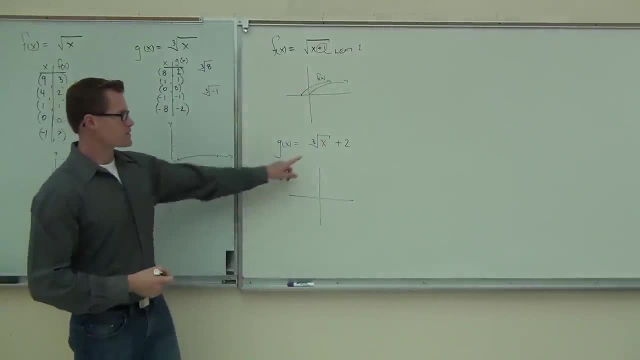 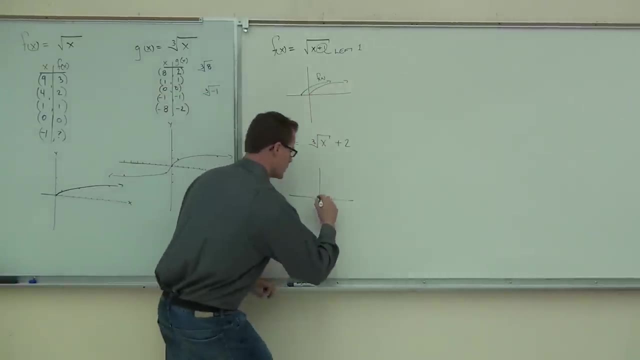 But then after that you can just shift them around. That's fine. What's this graph look like? Does it look exactly like this? No, No, It's also. it's got that other side to it, So the original one.